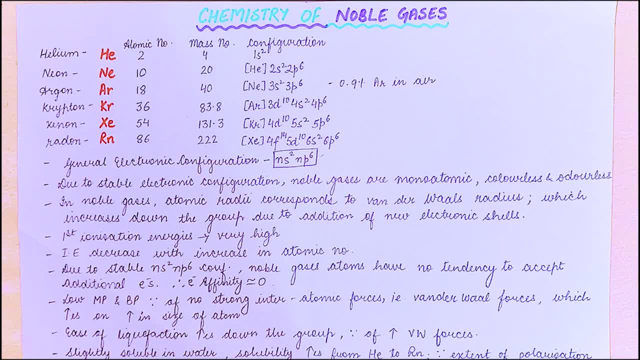 18 of the periodic table. These are gases at ordinary temperature and do not have chemical reactivity. Due to chemical inertness, these were called inert gases. However, nowadays, a number of compounds of these gases, particularly of xenon and krypton, have been prepared. This shows that 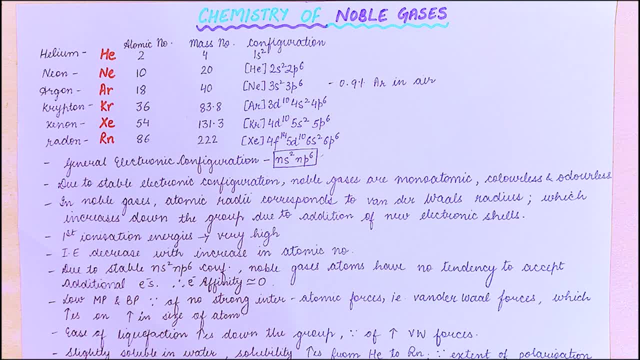 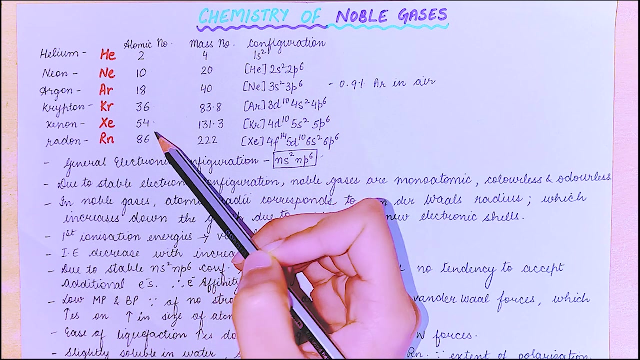 these gases are not completely inert. Consequently, these gases are now called noble gases instead of inert gases, which signifies that they are not completely inert. The atomic numbers of these gases are 2,, 10,, 18,, 36,, 54, 86.. The way to remember the atomic 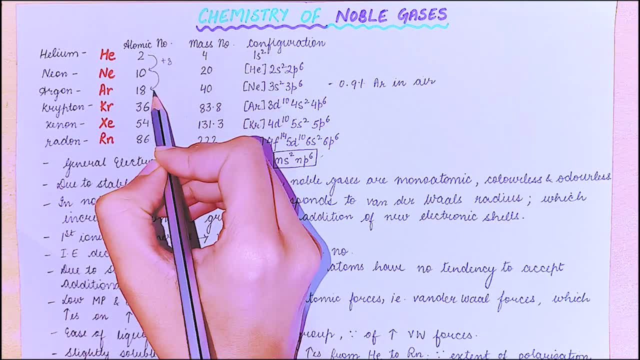 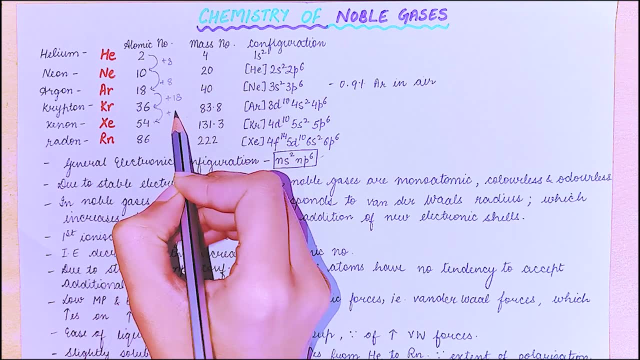 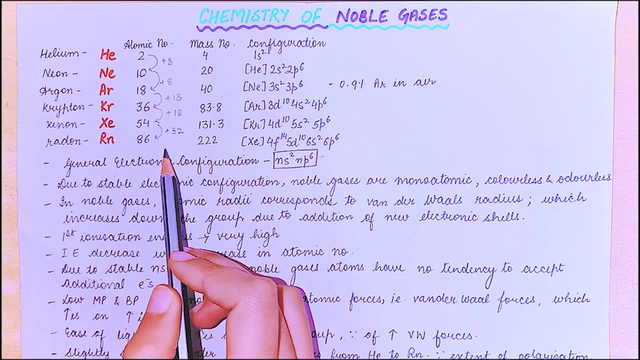 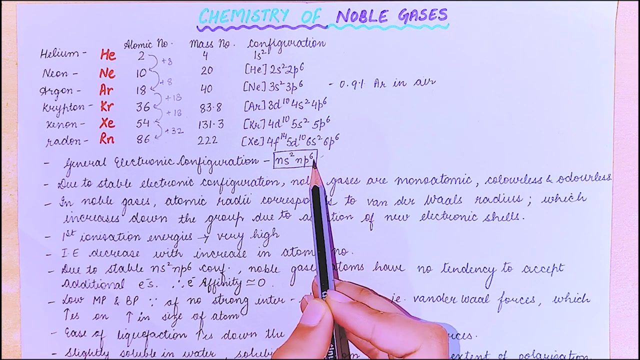 numbers I have told you in the previous video. You will get the link of that video in the description box. In this way you can learn all the atomic numbers. And the general electronic configuration of these gases is NS2NP6.. So you can see here that the electronic configuration is a fulfilled, stable. 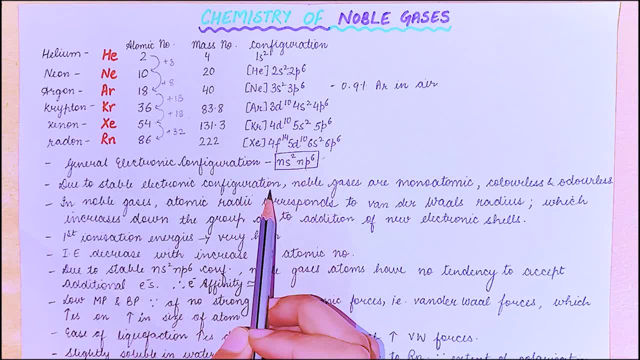 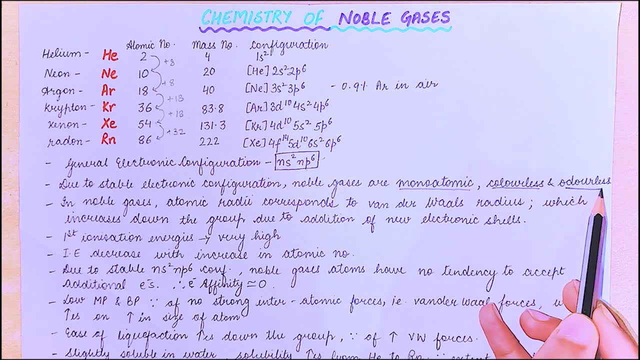 configuration. So, due to the stable electronic configuration, noble gases are monoatomic and they are colorless and odorless Because they are monotonic. they are monotonic, So they are fully filled In noble gases. atomic radii corresponds to van der Waals radius, which increases down. 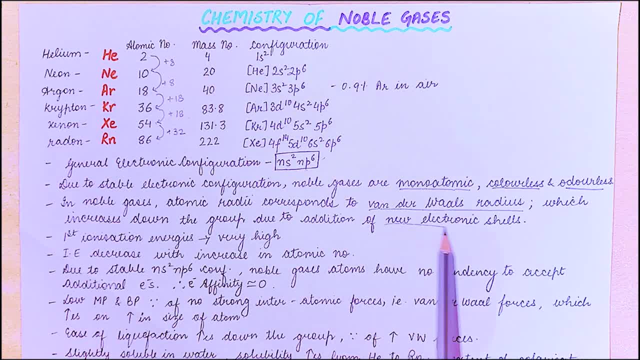 the group due to addition of new electronic shells. The first, ionization energies are very high because you know that it has a stable, fully filled configuration. Due to stable NS2NP6 configuration, these atoms have no tendency to accept additional electrons. That means electron affinity of these. 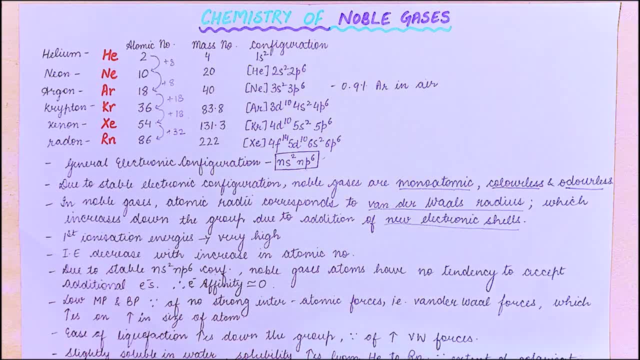 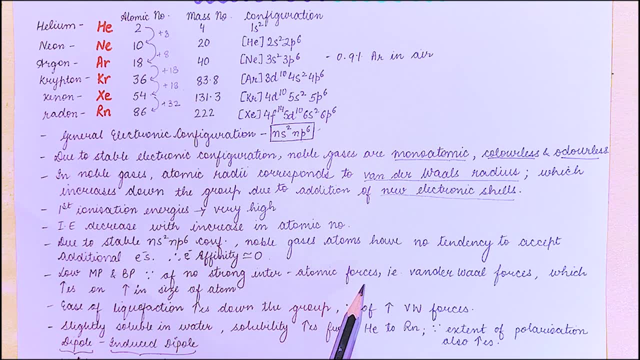 atoms of these elements is zero. Noble gases have low melting point and boiling point because of no strong interatomic forces, That is, it has van der Waals forces, which are weak forces, And these forces increases on increasing size of the atom, So down the group size. 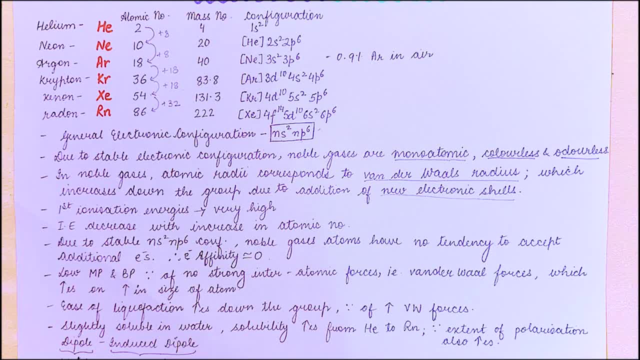 of atom increases, That means the forces between the atoms also increases. Ease of liquefaction increases down the group because of more van der Waal forces. So just keep in mind: more the van der Waal forces, stronger will be the bonding of these atoms Slightly soluble in water. So these 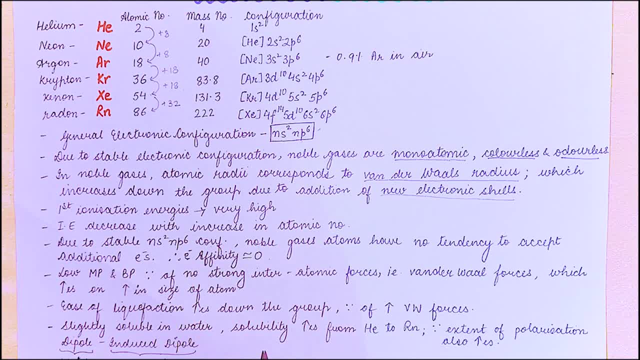 gases are slightly soluble in water And the solubility increases from helium to radon, As I told you, that the van der Waal forces between these increases. So these gases are increases or we can say the extent of polarization also increases. that is the dipole, induced dipole. 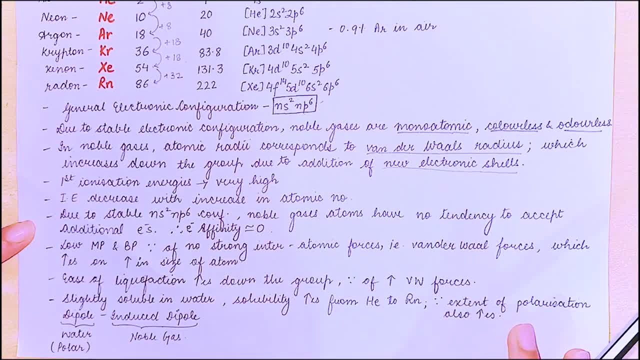 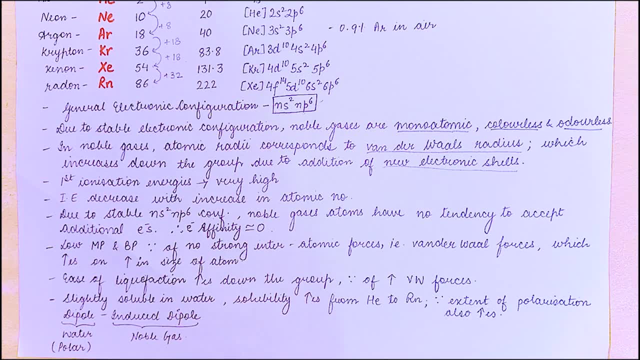 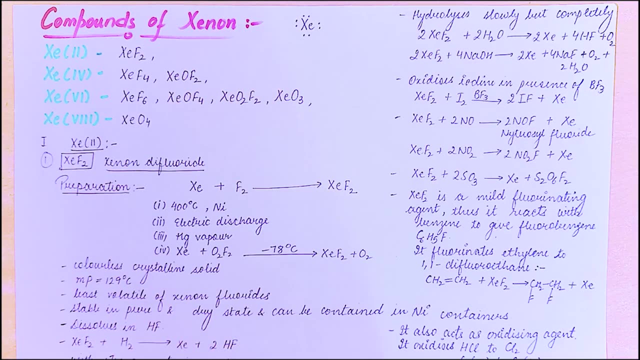 dipole means for polar, that is water, and induced dipole means noble gases. that means water will induce a dipole, will induce a charge into the noble gas which is neutral. now let's come to the main topic of this chapter, that is, compounds of xenon. the question will come. 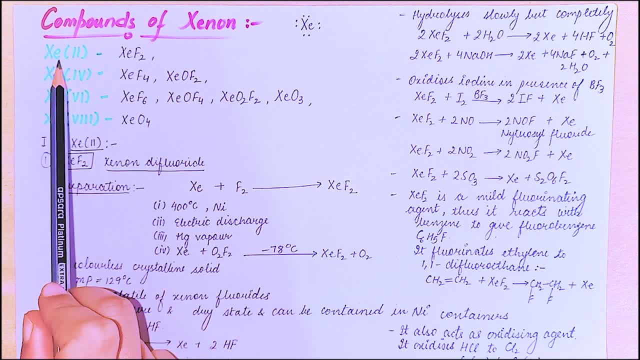 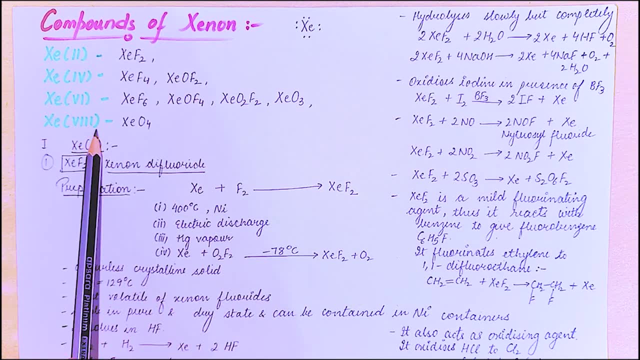 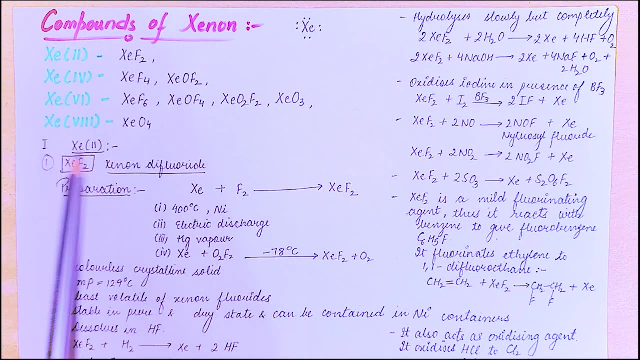 from this section, mostly xenon in plus two oxidation state, xenon in plus four oxidation state, xenon in plus six and plus eight oxidation states. we have four oxidation states in which xenon exists, so let's have a look over the first, that is, plus two oxidation state of xenon. the 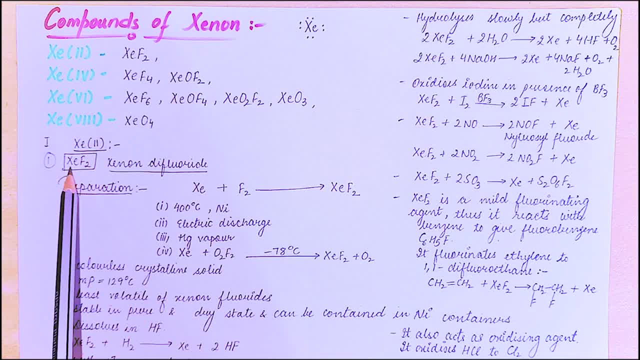 compound of xenon is the compound of xenon and the compound of xenon is the compound of xenon, which is in plus two oxidation state of xenon is xef2, that is xenon diphloride. how do we prepare xenon plus fluorine? when fluorine reacts with xenon, it forms xenon diphloride. so what are the? 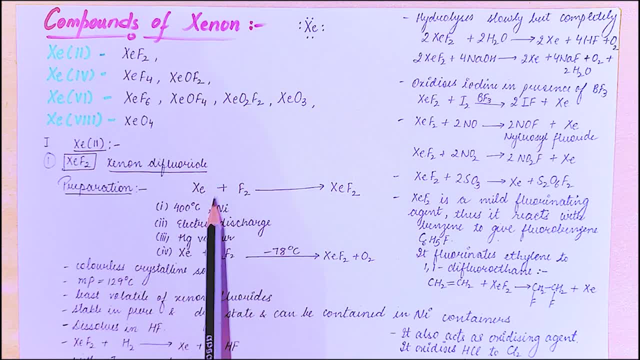 conditions. the conditions are. there can be four conditions. we can do this in four different conditions. the first condition is 400 degrees celsius temperature and in the presence of nickel. right, so you can do this. the reaction with this condition, or the second condition, is you can use electric discharge. 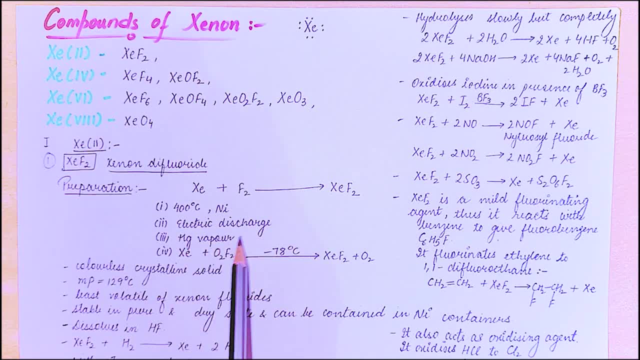 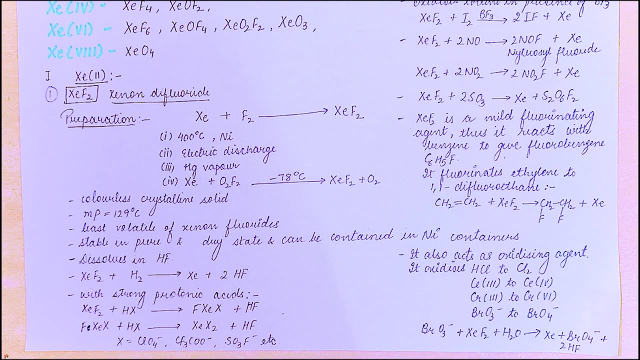 or we can use mercury vapors, or the fourth reaction, that is, xenon plus o2f2, gives xef2 plus o2 at a temperature of minus 78 degrees celsius, and then we can do this with the second. let's see the physical properties. it is a colorless crystalline, solid its 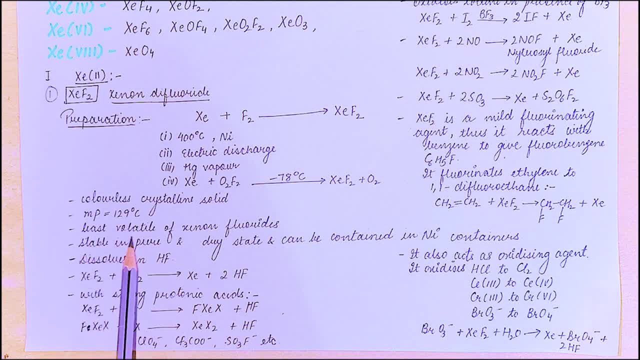 melting point is 129 degree Celsius. it is least volatile of xenon fluorides, stable in pure and dry state and can be obtained in nickel containers. can be contained and it dissolves in HF. xenon fluoride plus hydrogen gives xenon plus two molecules of HF. it gives substitution reaction with strong. 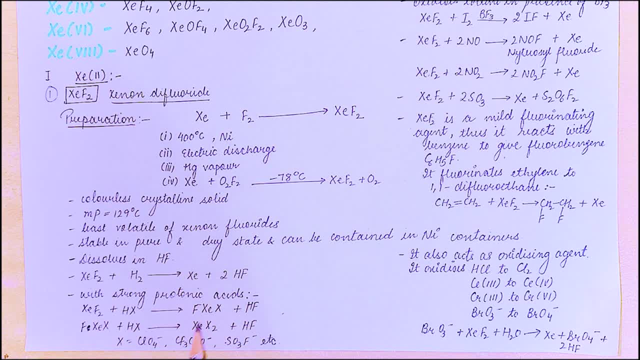 protonic acids. xe F 2 plus HX gives fxe x plus HF. fxe X plus HX gives Xe x2 plus HF. so you can understand the reactions just by listening. you have to write it along with the equation with me and try to understand from where the element is being displaced from. 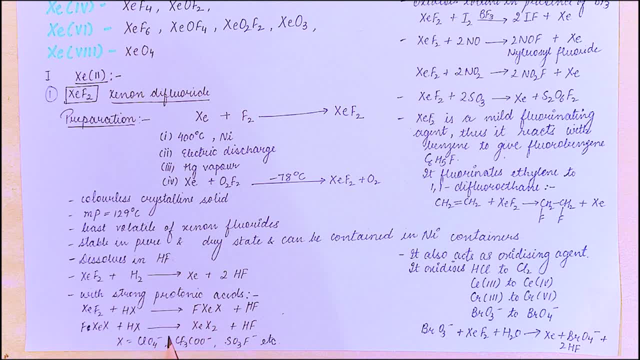 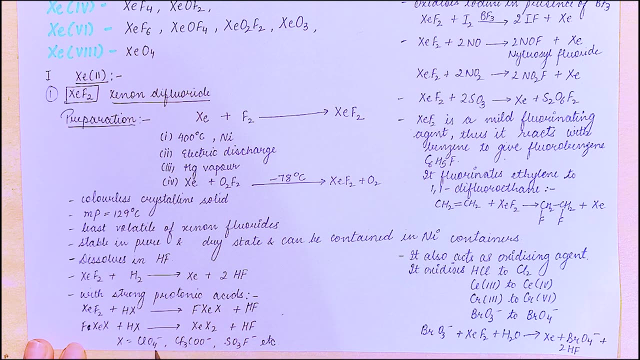 from where the element is being substituted, because these are substitution reaction. in this reaction you can see that one fluorine leaves and in place of fluorine X joins. X is a group. it can be ClO4 negative, Cf3COO negative, SO3F negative. so this group joins in place of one fluorine. so we get: 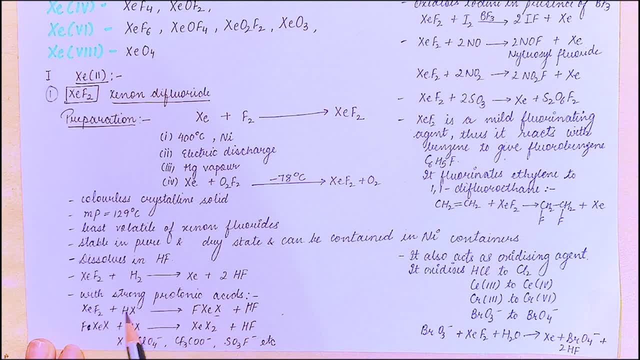 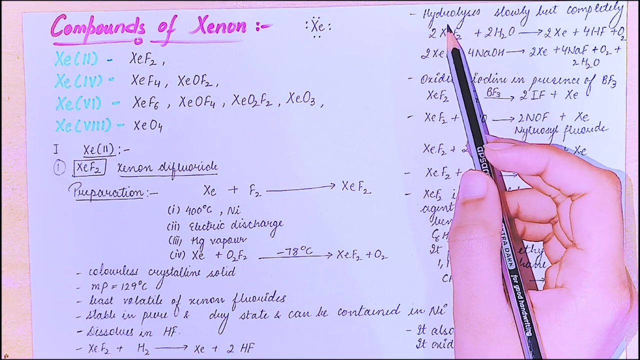 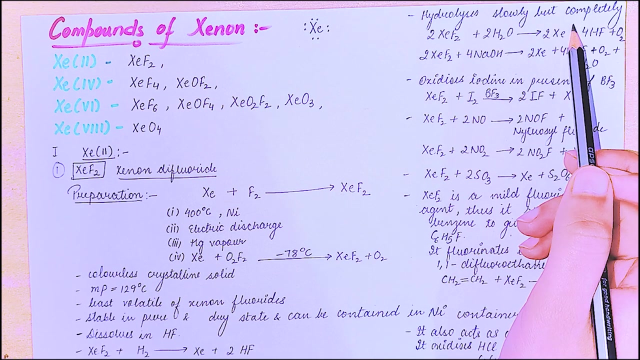 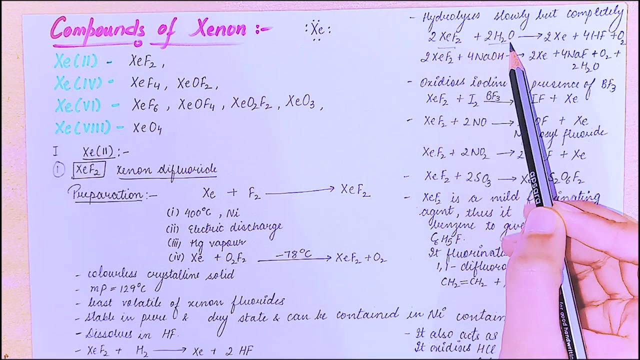 FXCX now, and from here we get HF right. similarly, in the other reaction, from here fluorine goes and this X group joins. we get XCX2 plus HF. it slowly but completely hydrolyzed in acidic or neutral medium or alkaline medium, right. so XCF2 plus water gives XC plus HF plus O2. so it is getting 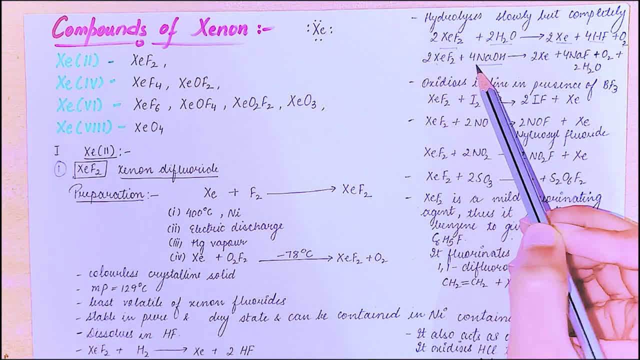 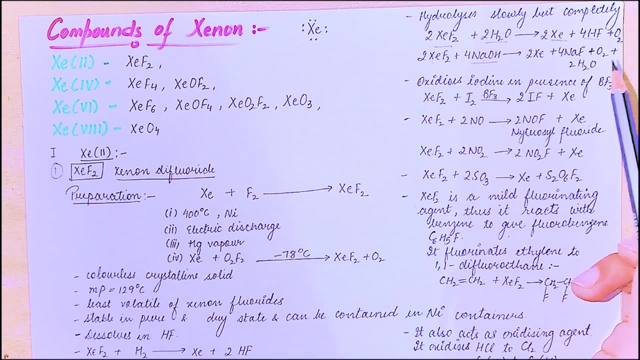 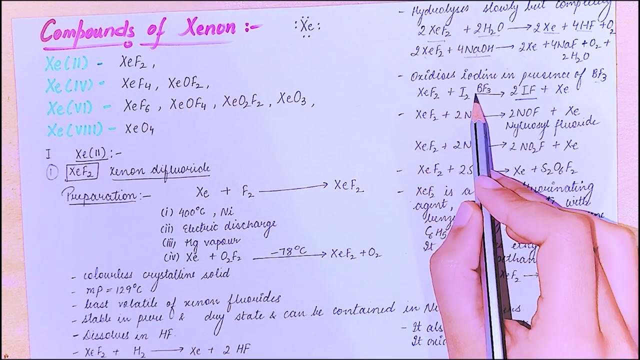 hydrolyzed XCF2 plus NaOH. that is an alkaline medium also. let's see, it gives XC plus NaF plus O2 plus water. it oxidizes iodine in the presence of BF3 to give IF. in all these reactions you can see we get IF here: XCF2 plus I2. 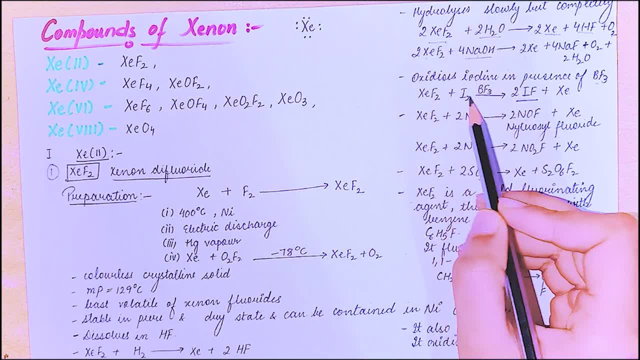 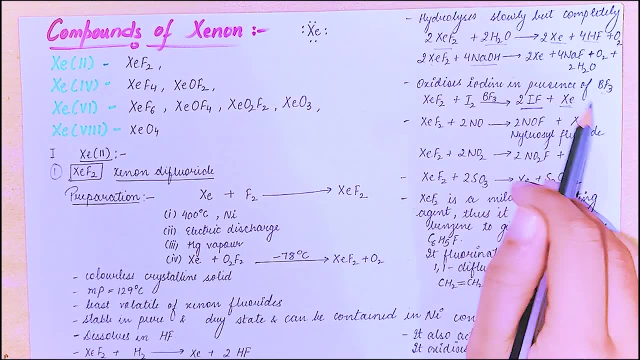 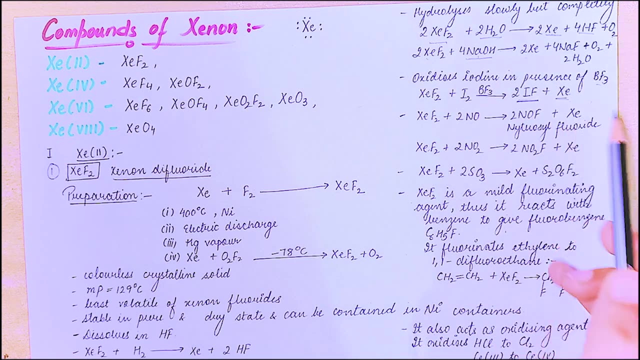 in the presence of BF3 we get IF. that means iodine plus fluorine gives IF and Xenon as it is. next we have XCF2 plus NO gives NOF plus XE. these reactions are just to show the reactivity of xenon diphylloride. so 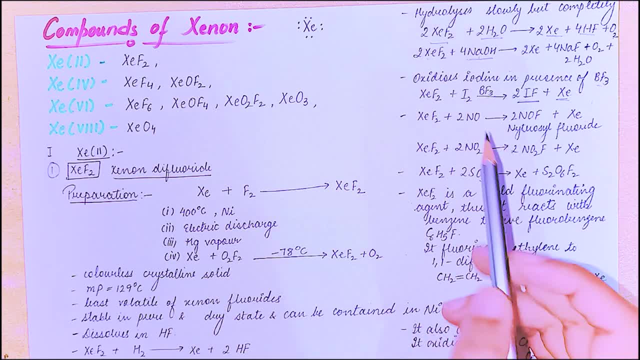 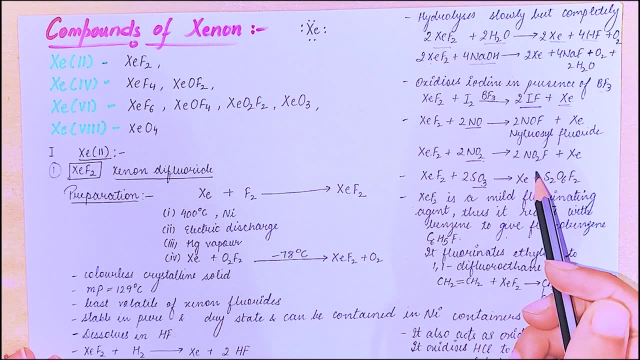 here we say that it reacts with 한노, NO2 and SO3 as well. so here we say that it reacts with Füranon, Endусовon, Endosanen and So3 as well. so these are just to show the reactivity of XC F2. 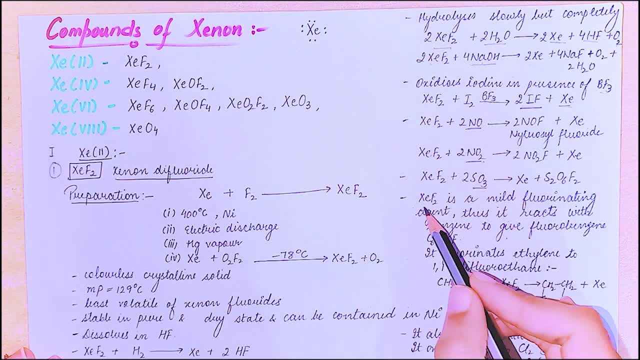 it is a mild fluorinating agent. XC F2 is a mild fluorinating agent. XCF2 is a mild fluorinating agent as well. XCf2 is a mild fluorinating agent. XCf2 is a mild fluorinating agent. XCf2 is a mild fluorinating agent. 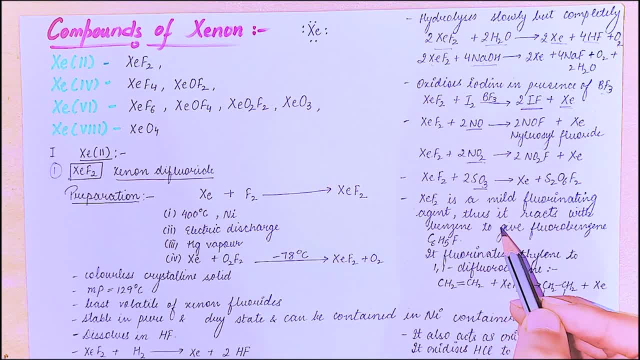 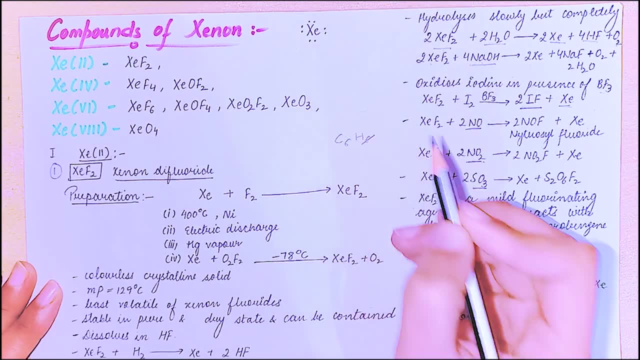 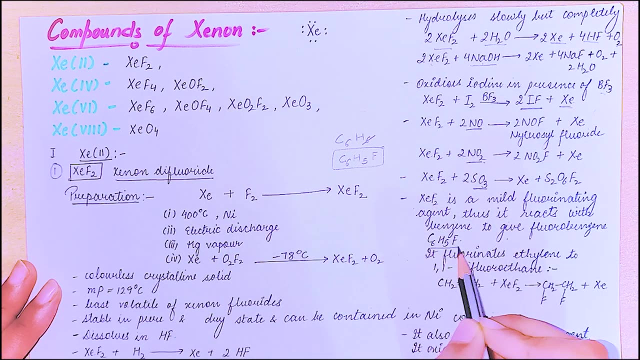 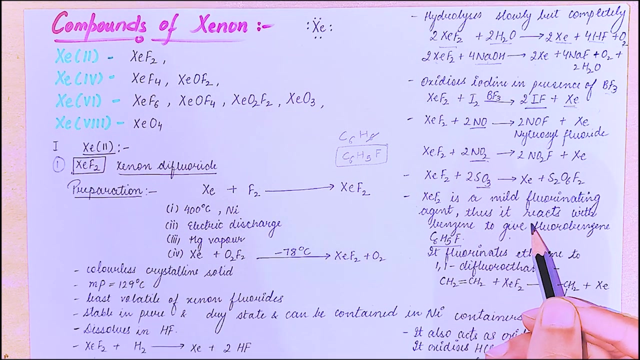 fluorinating agent. thus it reacts with benzene to give fluorobenzene. what is benzene? benzene is c6h6 if we remove one hydrogen and write fluorine in place of it. so we get fluorobenzene. so it is a fluorinating agent. it also fluorinates ethylene to 1,1-difluoroethane. 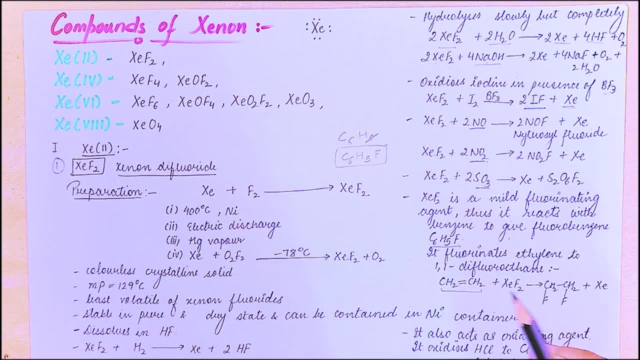 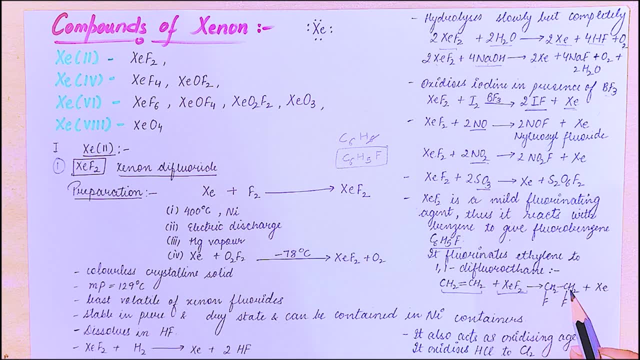 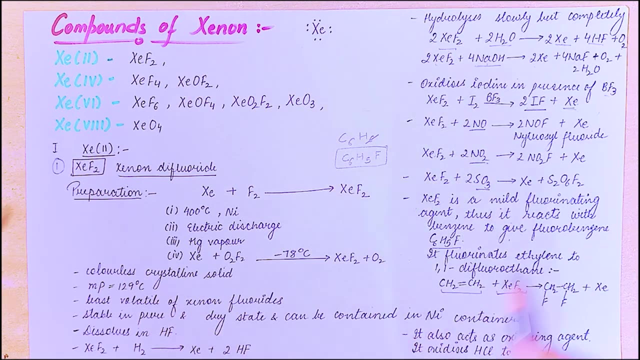 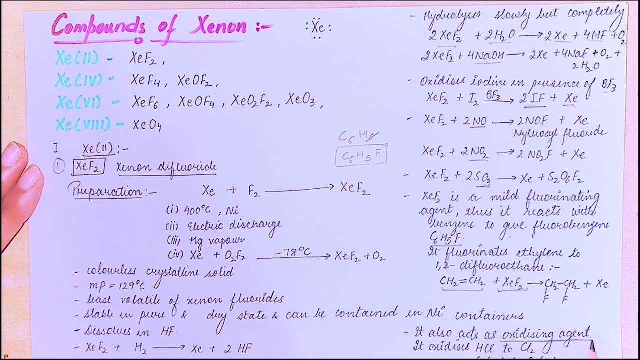 this is ethylene and this is xenon difluoride. when they both react, we get 1,1,1,2-difluoroethane right. let me correct it here. it must be 1,2, all right. so it also adds as oxidizing agent. 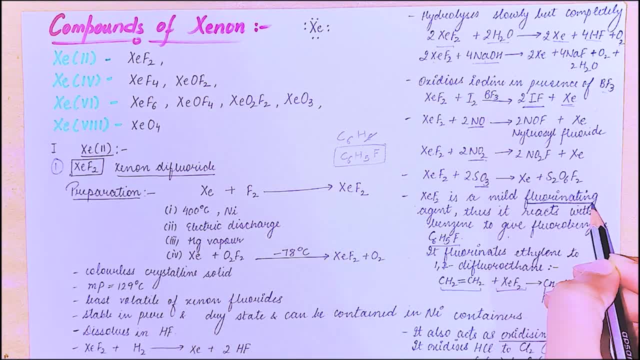 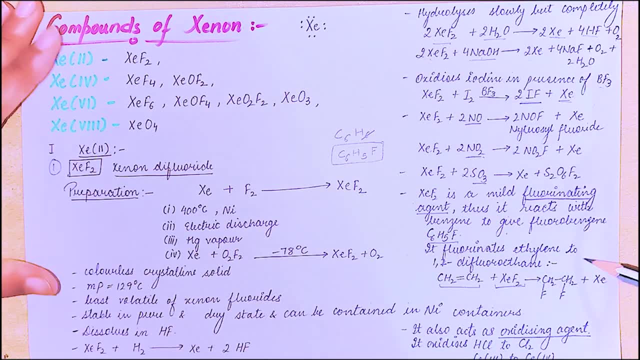 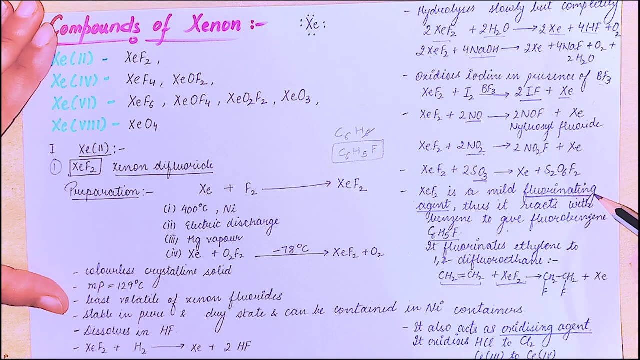 just note these points. these are the main points. like it is a fluorine eating agent, it is an oxidizing agent. then in the exam the examiner will ask you to give, to explain and to give examples of this. so you have to just write the examples to write that it is a fluorinating agent. it is an oxidizing. 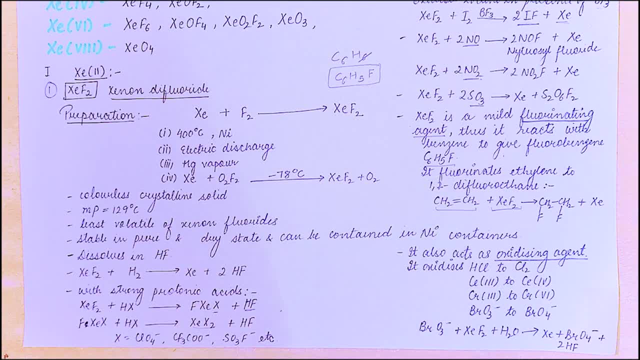 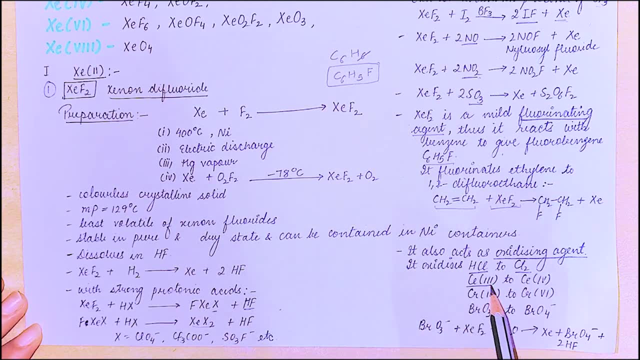 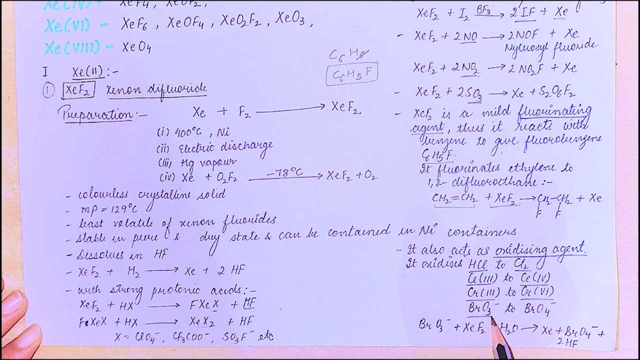 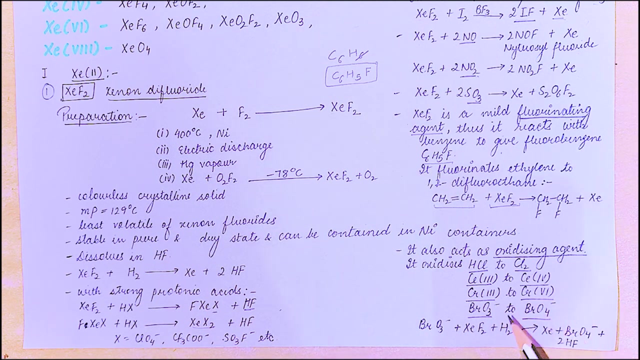 agent. so, being a strong oxidizing agent, it oxidizes HCl to chlorine cerium in plus three- state two plus four state chromium in plus three, two plus six state BrO3 negative to BrO4 negative. so you can see that the oxidation states are increasing in positive way. so these are getting oxidized in this reaction. you. 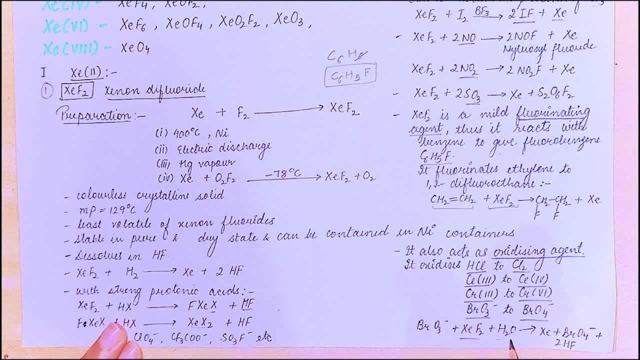 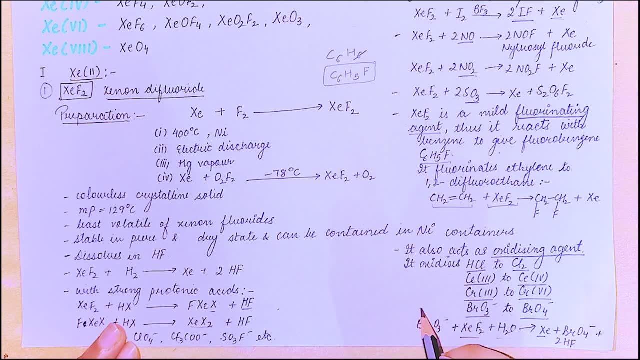 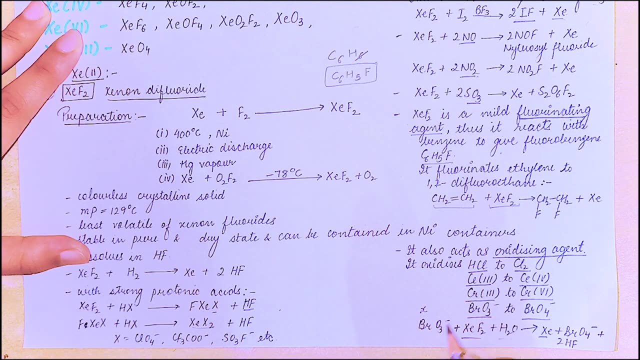 can see BrO3 negative plus CsF2. this water gives xenon. so here, okay, let me tell you how the oxidation states are changing. let the oxidation state of bromine be X and then give it as observed from oxygen. it will be minus 2. into 3, will be minus 6 is equal to minus 1. so 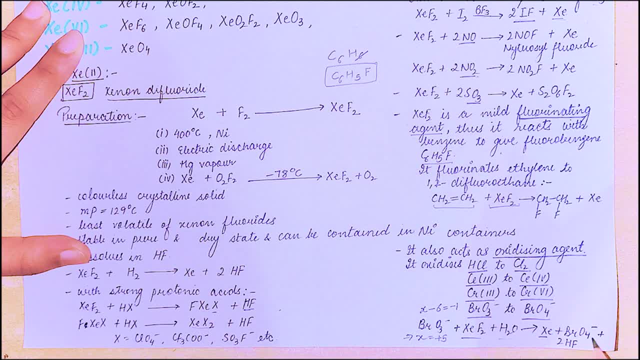 which implies X is plus 5 in this case, and in here we have X minus 8 is equal to minus 1, which implies X is equal to plus 7. so the state of bromine is changing from plus 5 to plus 7. that means it is being oxidized. Br o3. 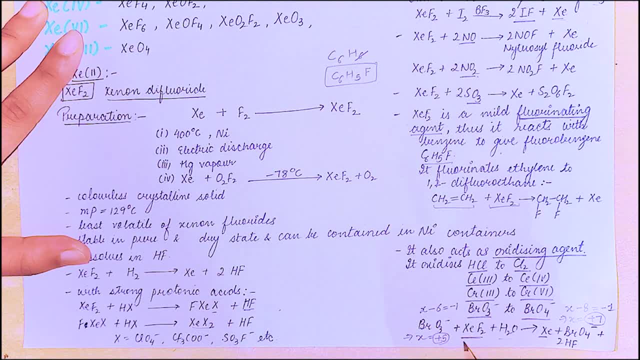 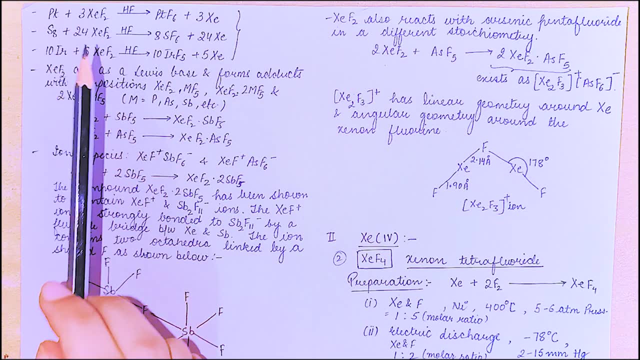 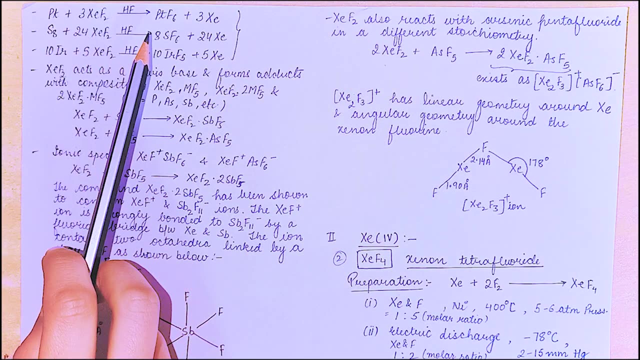 negative is being oxidized, and oxidized oxidizing agent is Xe f2. all right now xenon difluoride in anhydrous HF, that is, hydrogen fluoride. it reacts readily with platinum metals or sulphur powder or iridium to produce highest fluorides. as 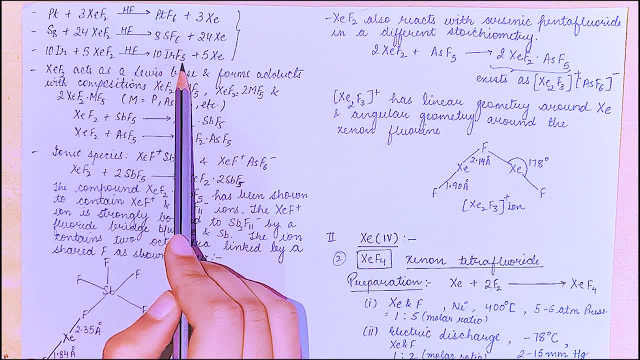 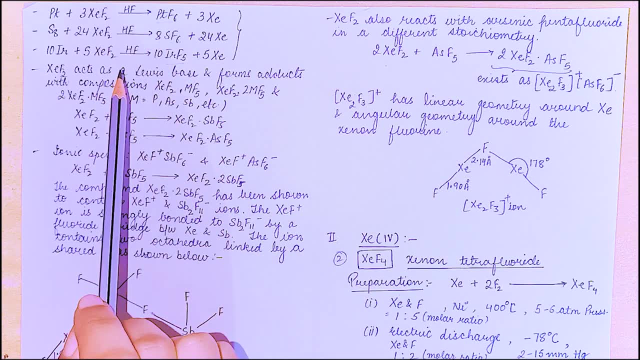 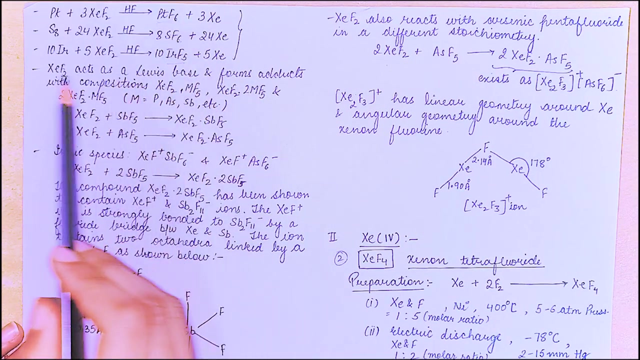 you can see Pt f6, sf6, iridium f5, so you can see that the hydrogen fluoride is being oxidized and oxidizing agent is: these are highest fluorides which are produced on reaction with HF. all right, in Br f2 solution, xenon difluoride act as a Lewis base and form adducts right it. 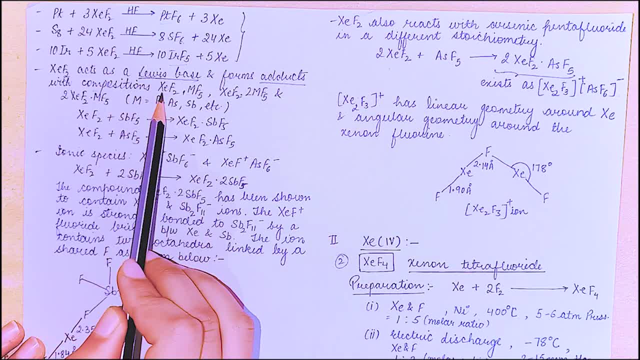 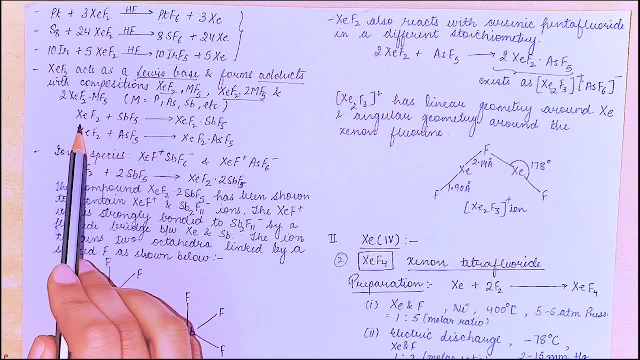 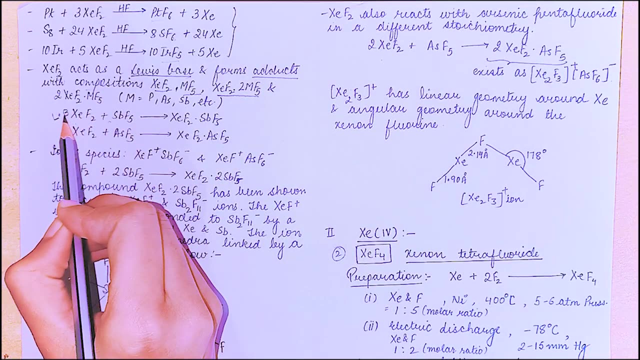 acts as a Lewis base and it forms adducts with compositions: Xe f2, M f5, Xe f2 dot, M f5. right, so let's see, this is Xe f2 plus Sb f5. now this acts as a Lewis base base- Lewis. 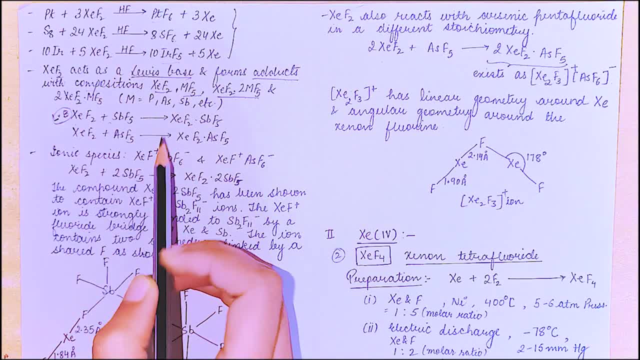 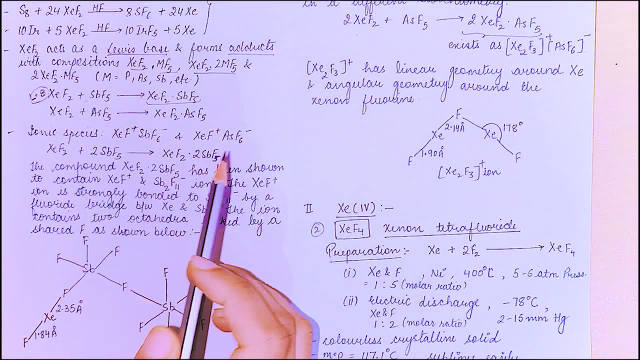 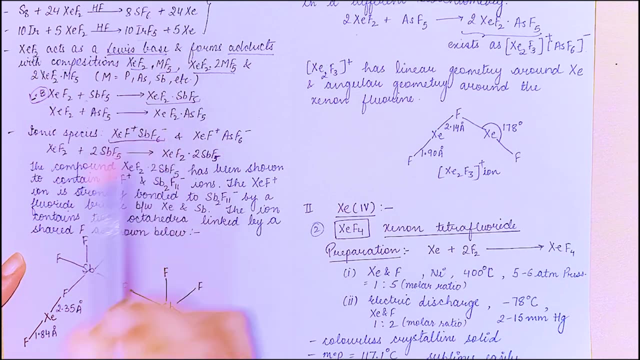 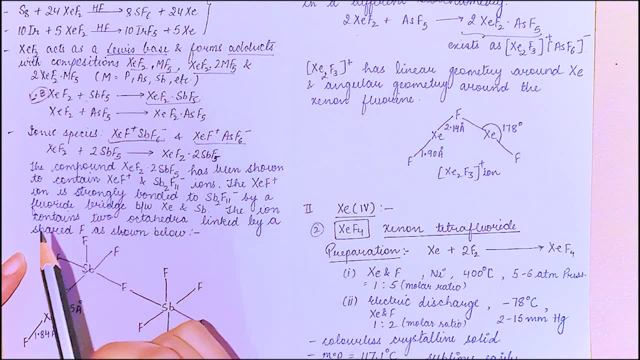 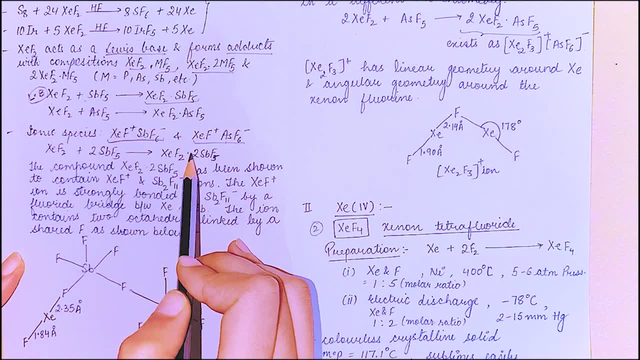 Xe f plus FB F5. negative: Xe f2 when reacts with Sb f5. it forms Xe f2 dot 2. reacts with Sb f5. it forms Xe f2 dot 2. reacts with Sb f5. it forms Xe f2 dot 2- Sb f5. the compound Xe f2 dot 2- Sb f5. 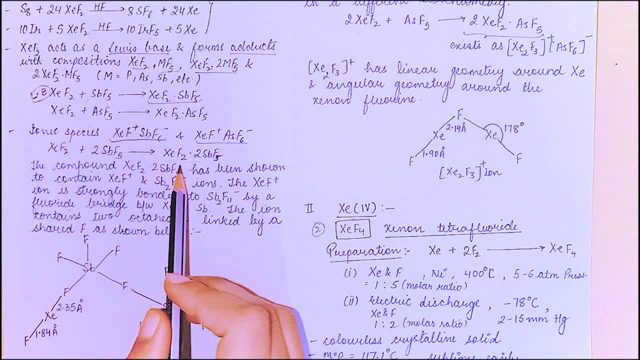 Sb f5. the compound Xe f2- dot 2- Sb f5. Sb f5. the compound Xe f2- dot 2- Sb f5. this compound has been shown to contain. this compound has been shown to contain. this compound has been shown to contain Xe f positive and SB 2 f11 negative ions. 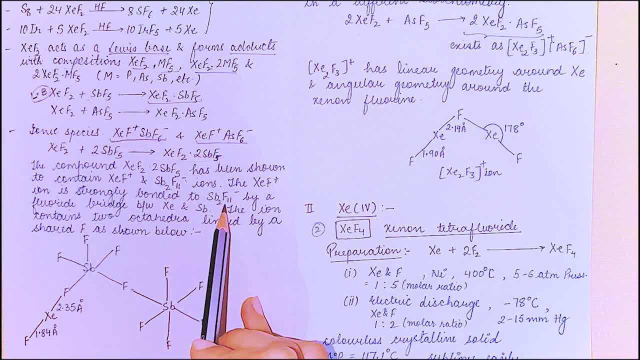 Xe f positive and SB 2 f11 negative ions. Xe f positive and SB 2 f11 negative ions. the Xe f positive ion is strongly bonded. the Xe f positive ion is strongly bonded. the Xe f positive ion is strongly bonded to SB 2 f11 negative by a fluoride. 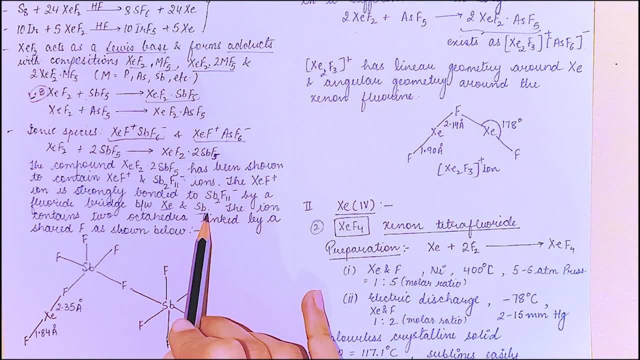 to SB 2 f11 negative by a fluoride to SB 2 f11 negative by a fluoride. bridge between xenon and antimony: the bridge between xenon and antimony: the bridge between xenon and antimony. the ion contains two octahedral linking. 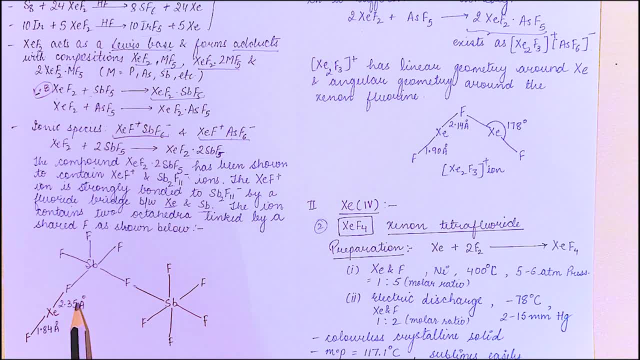 ion contains two octahedral linking. ion contains two octahedral linking between the shared F fluorines. so this between the shared F fluorines. so this between the shared F fluorines. so this is the octahedral linkage one you can is the octahedral linkage one you can. 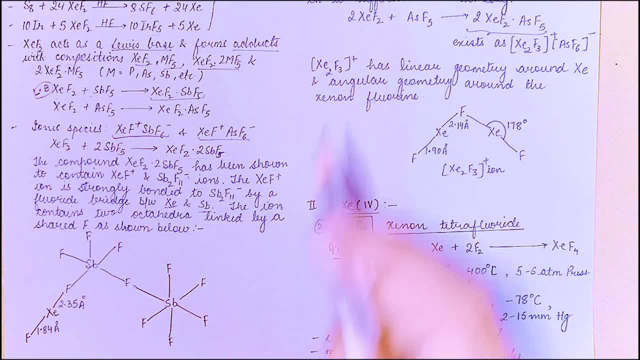 is the octahedral linkage one you can see in the figure. see in the figure. see in the figure. Xe f2 also reacts with the arsenic. Xe f2 also reacts with the arsenic. Xe f2 also reacts with the arsenic pentafluoride in a different. 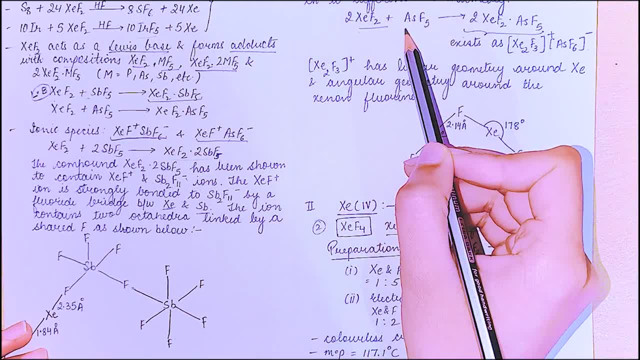 pentafluoride in a different pentafluoride in a different stoichiometry, like Xe f2. two molecules stoichiometry like Xe f2. two molecules stoichiometry like Xe f2. two molecules plus arsenic right and the fluoride it. 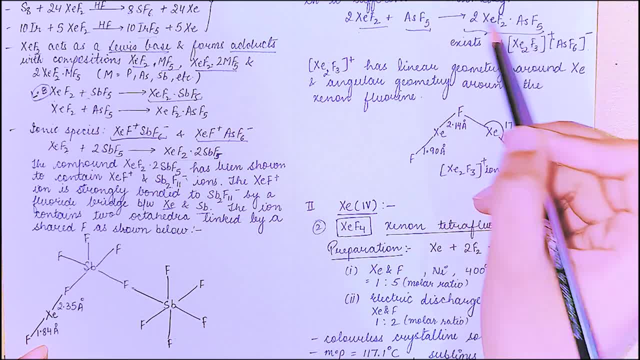 plus arsenic right and the fluoride. it plus arsenic right and the fluoride. it gives Xe f2 dot a SF 5: 2 with this one. gives Xe f2 dot a SF 5: 2 with this one. gives Xe f2 dot a SF 5: 2 with this one. so it exists as ionic species also, Xe 2. 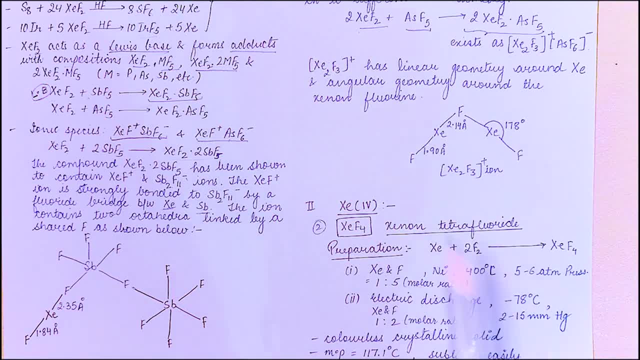 so it exists as ionic species also Xe 2. so it exists as ionic species also Xe 2- f3 positive, a s f6 negative. Xe 2- f3 f3 positive, a s f6 negative. Xe 2- f3 positive, Xe 2- f3 positive. it has a linear 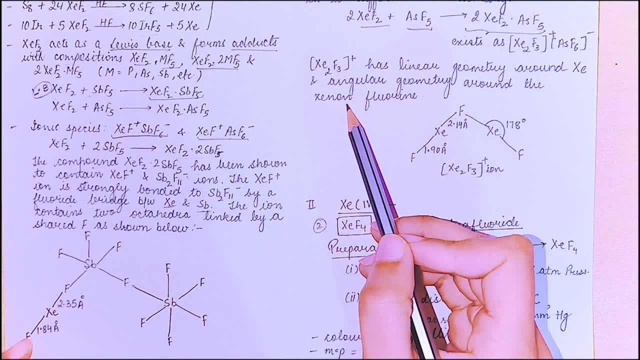 f3 positive. it has a linear f3 positive. it has a linear geometry around xenon and angular geometry geometry around xenon and angular geometry geometry around xenon and angular geometry around the xenon flow to chlorine. so around the xenon flow to chlorine. so 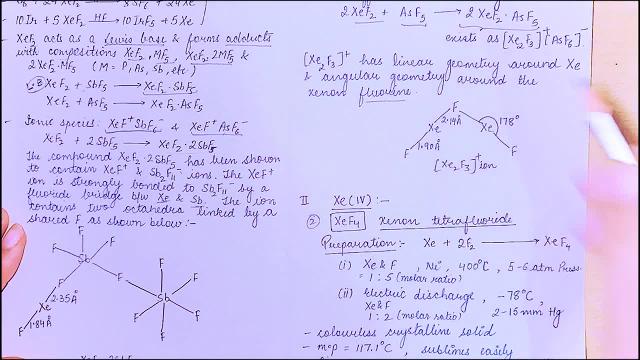 around the xenon flow to chlorine. so you can see in this figure that it has a. you can see in this figure that it has a. you can see in this figure that it has a linear geometry along xenon and angular. linear geometry along xenon and angular. 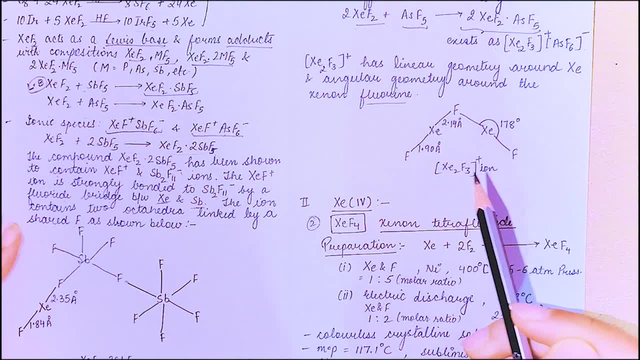 linear geometry along xenon and angular geometry at fluorine like this: okay, so geometry at fluorine like this: okay, so geometry at fluorine like this: okay, so these were. these were, these were compounds of xenon in plus two. compounds of xenon in plus two. compounds of xenon in plus two oxidation state. so let's see the plus oxidation state. so let's see the plus oxidation state. so let's see the plus four oxidation state of xenon: it is xenon. four oxidation state of xenon: it is xenon. 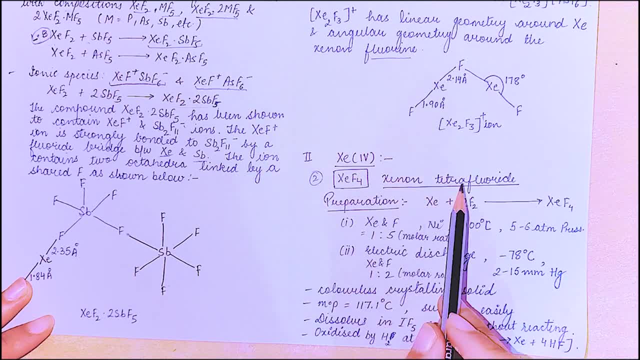 four: oxidation state of xenon. it is xenon tetrafluoride the first compound, tetrafluoride the first compound. tetrafluoride, the first compound we are going to study in plus four status. we are going to study in plus four status. 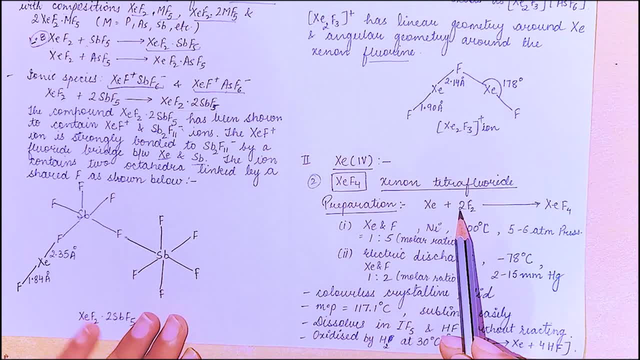 we are going to study in plus four status: xenon tetrafluoride: that means for xenon tetrafluoride. that means for xenon tetrafluoride. that means for fluorine xenon combines with two fluorine. fluorine xenon combines with two fluorine. 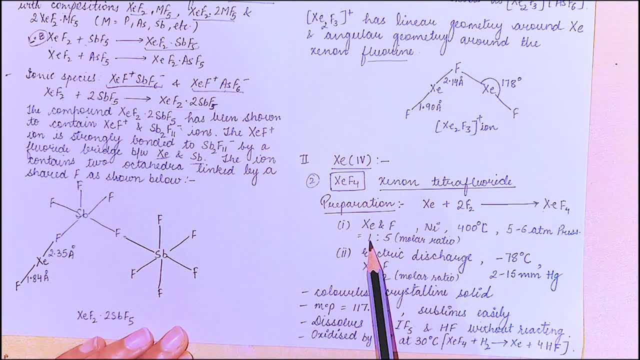 fluorine. xenon combines with two fluorine to form xcf4. they combine in a to form xcf4. they combine in a to form xcf4. they combine in a molar ratio of 1 is to 5 in the presence of molar ratio of 1 is to 5 in the presence of. 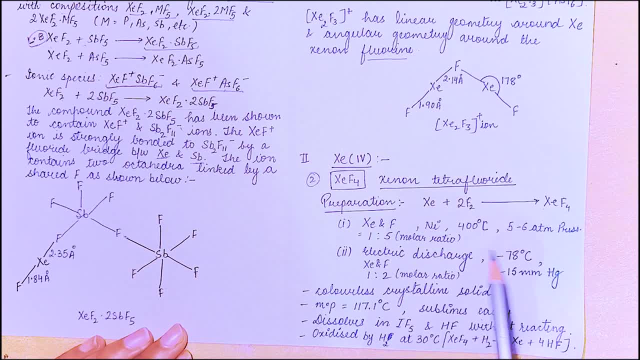 molar ratio of 1 is to 5. in the presence of nickel at 400 degree Celsius: 5 to 6. nickel at 400 degree Celsius: 5 to 6. nickel at 400 degree Celsius: 5 to 6 atmosphere pressure. or you can use the: 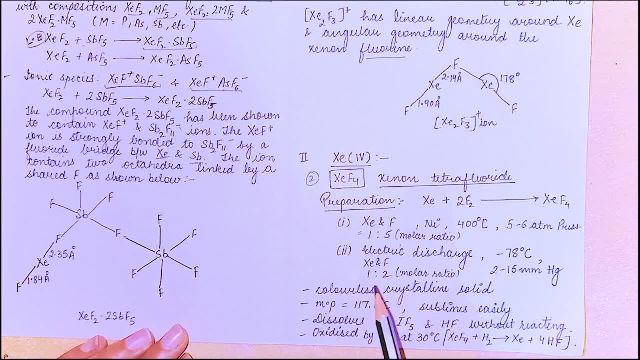 atmosphere pressure. or you can use the atmosphere pressure or you can use the second condition, that is electric. second condition: that is electric. second condition: that is electric discharge at minus 78 degree Celsius. in discharge at minus 78 degree Celsius. in discharge at minus 78 degree Celsius. in the molar ratio 1 is to 2 at the 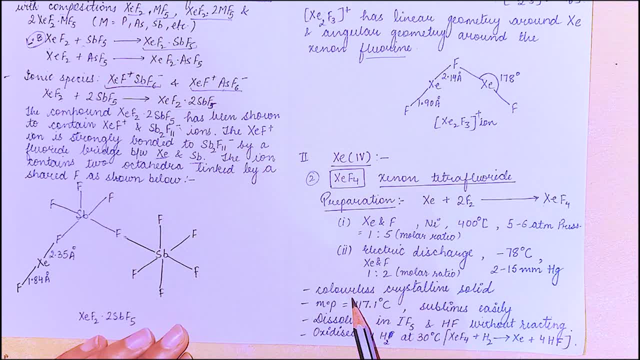 the molar ratio 1 is to 2 at the: the molar ratio 1 is to 2 at the pressure of 2 to 15 millimeter mercury. pressure of 2 to 15 millimeter mercury. pressure of 2 to 15 millimeter mercury. it is a colorless crystalline, solid. 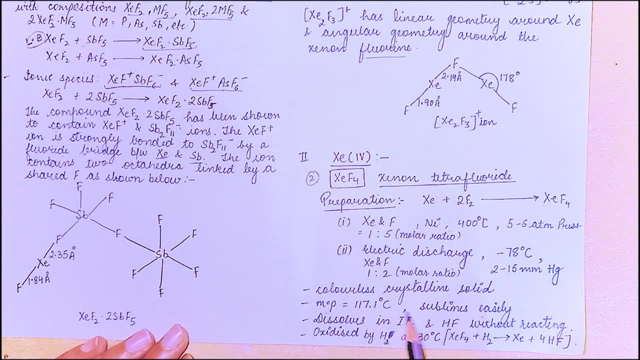 it is a colorless crystalline solid. it is a colorless crystalline solid which have a melting point of 117 point, which have a melting point of 117 point, which have a melting point of 117 point. 1 degree Celsius sublimes easily, right? 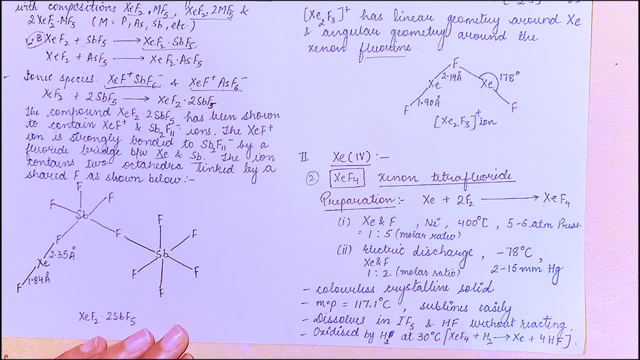 1 degree Celsius sublimes easily right. 1 degree Celsius sublimes easily right. it dissolves in if7 and HF without it dissolves in if7 and HF without. it dissolves in if7 and HF without reacting and it is oxidized by hydrogen. 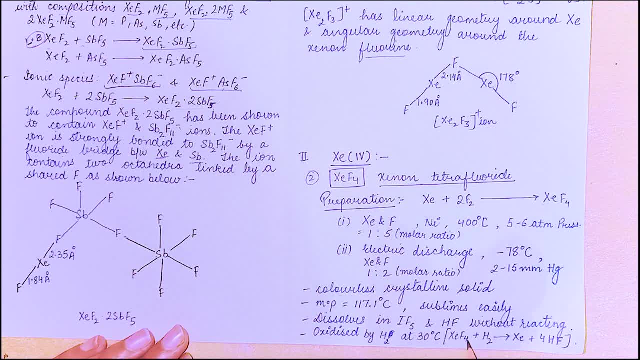 reacting and it is oxidized by hydrogen reacting and it is oxidized by hydrogen at 30 degrees Celsius. you can see that at 30 degrees Celsius. you can see that at 30 degrees Celsius. you can see that XC, f4 plus hydrogen gives X C plus 4 HF. 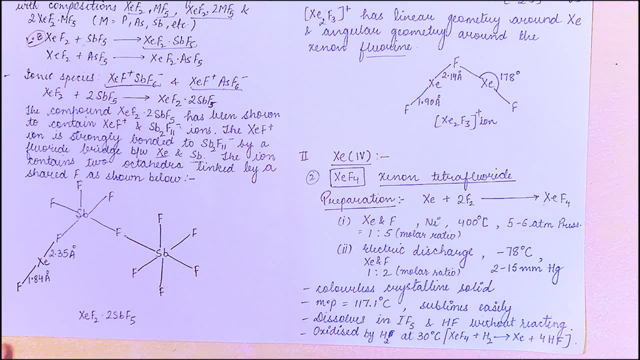 so, if you are listening to me carefully, so if you are listening to me carefully, so if you are listening to me carefully, you must have noted that I have said, you must have noted that I have said, you must have noted that I have said: oxidized by hydrogen at 30 degrees. 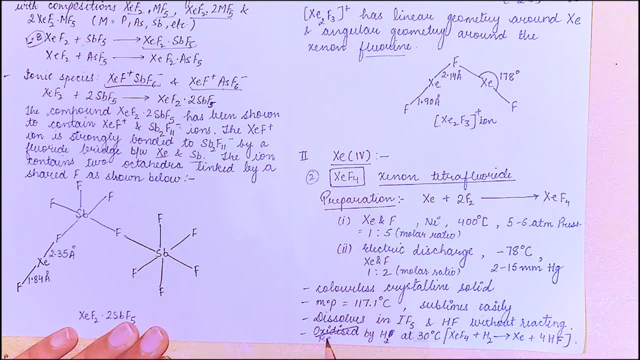 oxidized by hydrogen at 30 degrees. oxidized by hydrogen at 30 degrees Celsius. it must be reduced. it should not Celsius. it must be reduced. it should not Celsius. it must be reduced. it should not be oxidized. how can hydrogen oxidize be oxidized? how can hydrogen oxidize? 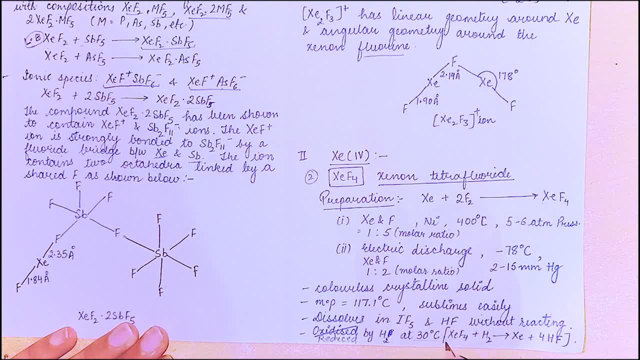 be oxidized. how can hydrogen oxidize anything so hydrogen XE f4 is xenon? is anything so hydrogen XE f4 is xenon? is anything so hydrogen XE f4 is xenon? is in plus 4 oxidation state and it is in plus 4 oxidation state and it is. 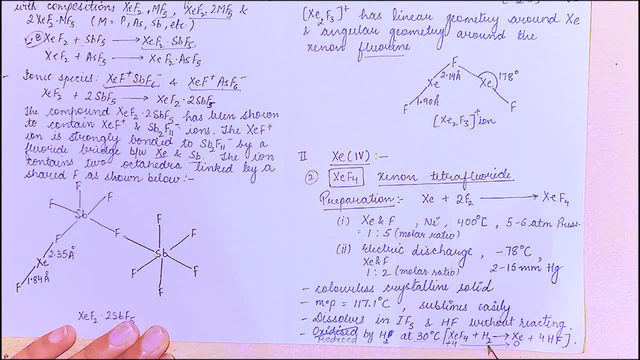 in plus 4 oxidation state and it is going to zero oxidation state. so it is going to zero oxidation state, so it is going to zero oxidation state, so it is going to zero oxidation state and the hydrogen is going to zero oxidation state and the hydrogen is. 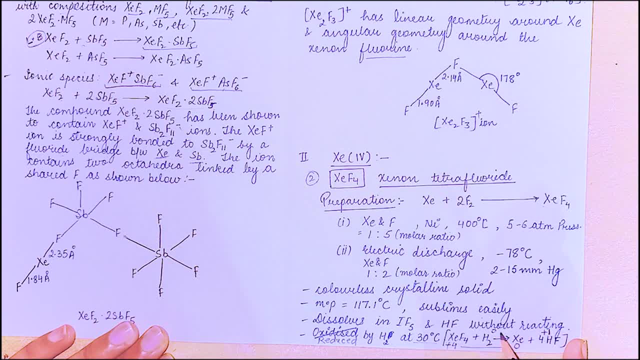 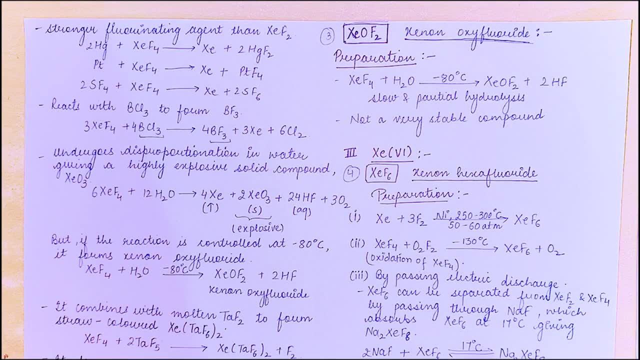 going to zero oxidation state and the hydrogen is converting from 0 to plus 1. converting from 0 to plus 1, converting from 0 to plus 1 oxidation state. that means the hydrogen is oxidation state. that means the hydrogen is oxidation state. that means the hydrogen is getting oxidized. right, it is a better 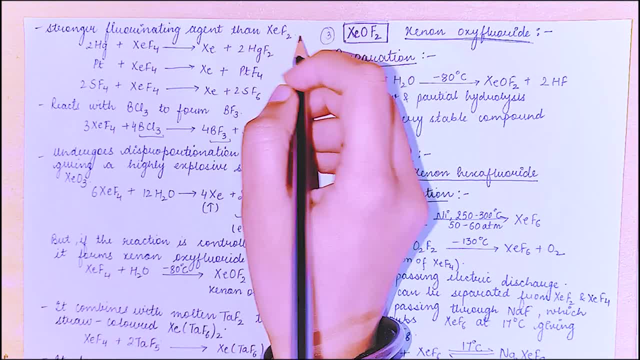 getting oxidized right, it is a better getting oxidized right, it is a better. ox fluorinating agent then xenon fluoride. ox fluorinating agent then xenon fluoride. ox fluorinating agent then xenon fluoride- di fluoride. so mercury when reacts with di fluoride. so mercury when reacts with. 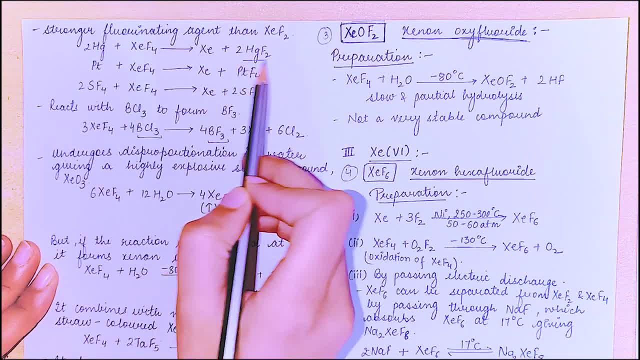 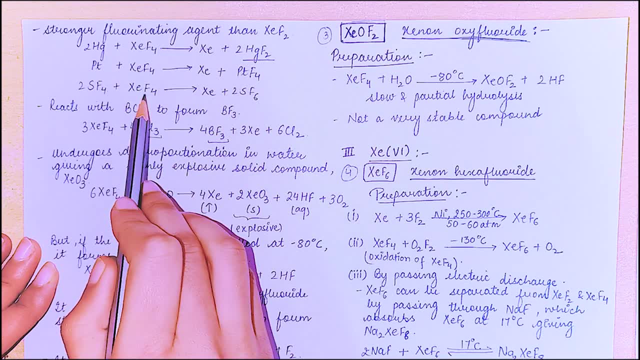 di fluoride. so mercury when reacts with XE f4 gives xenon plus HD f2. platinum on XE f4. gives xenon plus HD f2- platinum on XE f4. gives xenon plus HD f2- platinum on reaction. gives PT f4, SF 4 on reaction. 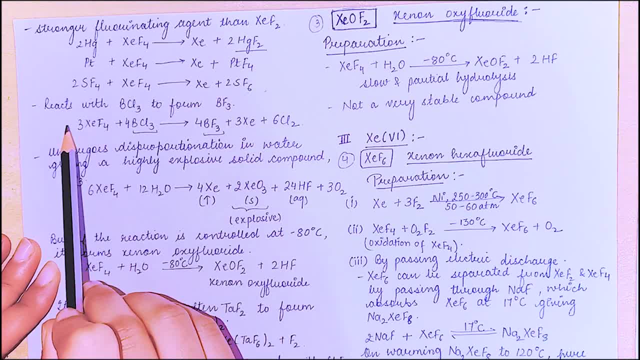 reaction gives PT f4- SF 4 on reaction. reaction gives PT f4- SF 4 on reaction with XE f4 gives SF 6 the xenon. it also with XE f4 gives SF 6 the xenon. it also with XE f4 gives SF 6 the xenon. it also reacts with bcl-3 to form bf3. let's see: 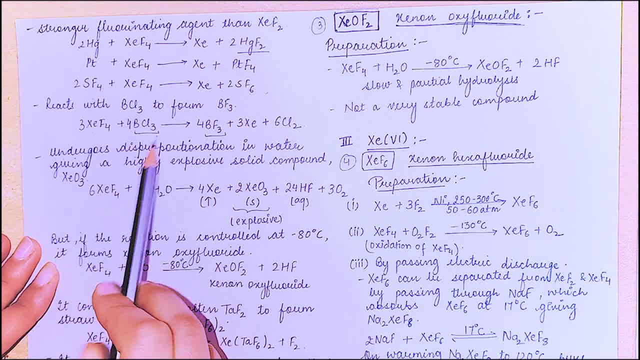 reacts with bcl-3 to form bf3. let's see reacts with bcl-3 to form bf3. let's see how xenon tetrafluoride or reaction. how xenon tetrafluoride or reaction. how xenon tetrafluoride or reaction with bcl-3 forms bf3 plus xenon plus. 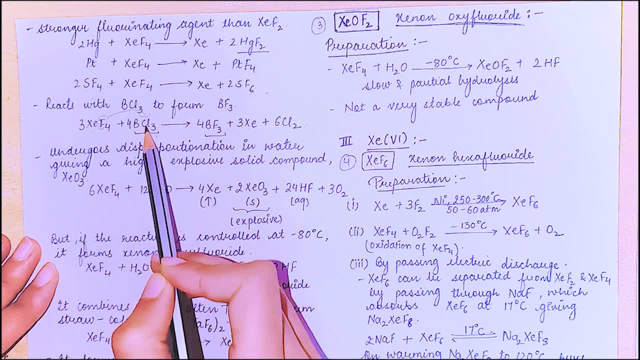 with bcl-3 forms, bf3 plus xenon plus with bcl-3 forms, bf3 plus xenon plus chlorine. that means the fluorine ions are with bcl-3 forms, bcl-3 forms, bcl-3 ions are with bcl-3 forms- bcl-3 ions are transferred here and chlorine forms cl2. 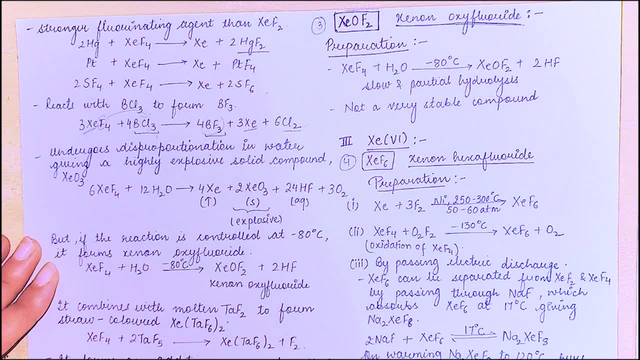 transferred here, and chlorine forms cl2 transferred here, and chlorine forms cl2. it forms bf3 and the xenon it undergoes. it forms bf3 and the xenon it undergoes. it forms bf3 and the xenon it undergoes disproportionation in water, giving a 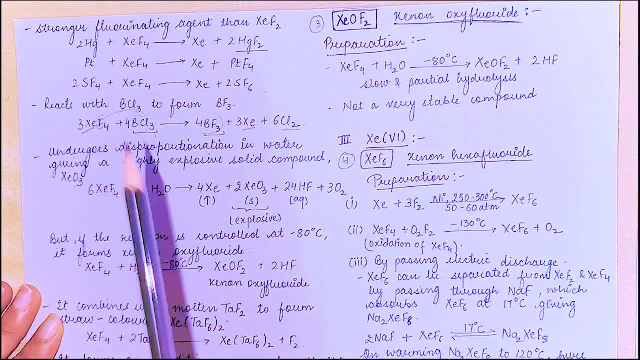 disproportionation in water, giving a disproportionation in water, giving a highly explosive solid compound. that is highly explosive solid compound. that is highly explosive solid compound. that is XCO 3- dot 6. okay, let's see this. it is XCO 3- dot 6. okay, let's see this. it is. 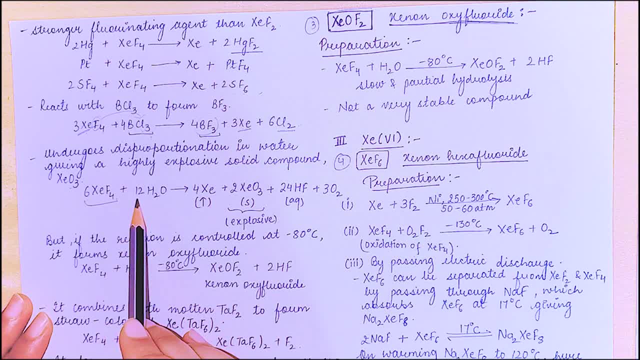 XCO 3, dot 6. okay, let's see this. it is very interesting. this is XE f4 on an very interesting. this is XE f4 on an very interesting. this is XE f4 on an addition of water, on reacting with water. 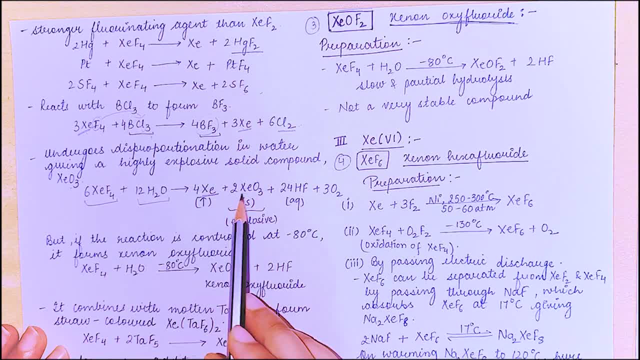 addition of water on reacting with water. addition of water. on reacting with water, it forms xenon plus XCO 3 plus HF plus. it forms xenon plus XCO 3 plus HF plus. it forms xenon plus XCO 3 plus HF plus O2. this XCO 3 is a solid compound and 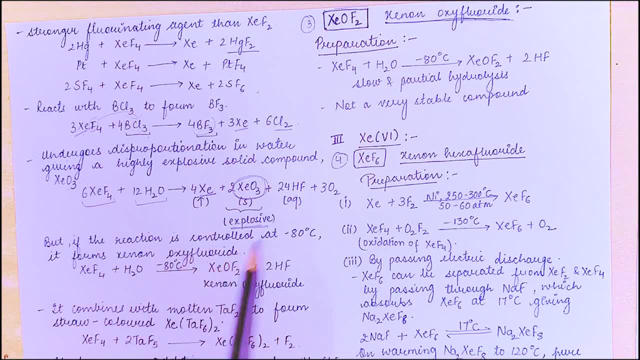 O2- this XCO 3- is a solid compound. and O2- this XCO 3- is a solid compound and it is explosive, right. but if the reaction, it is explosive, right. but if the reaction, it is explosive, right, but if the reaction is controlled at minus 80 degree Celsius. 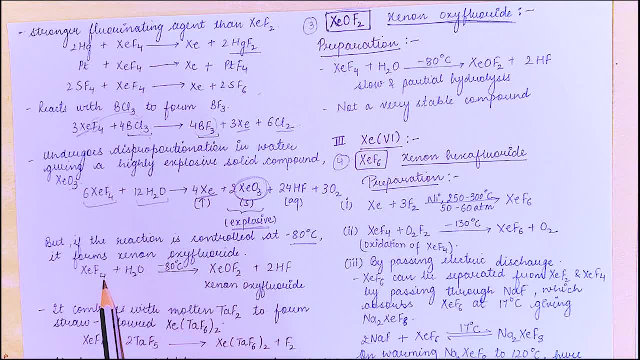 is controlled at minus 80 degree Celsius. is controlled at minus 80 degree Celsius, it forms xenon oxy fluoride. that is xenon. it forms xenon oxy fluoride. that is xenon. it forms xenon oxy fluoride. that is xenon tetrafluoride plus water at minus 80. 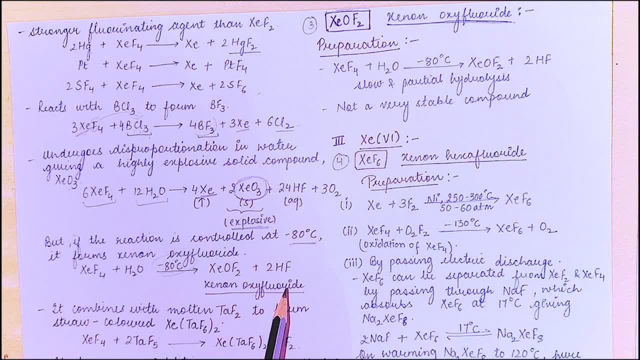 tetrafluoride plus water at minus 80. tetrafluoride plus water at minus 80 degrees Celsius gives xenon oxy fluoride degrees Celsius. gives xenon oxy fluoride degrees Celsius. gives xenon oxy fluoride plus HF. right, it combines with molten. 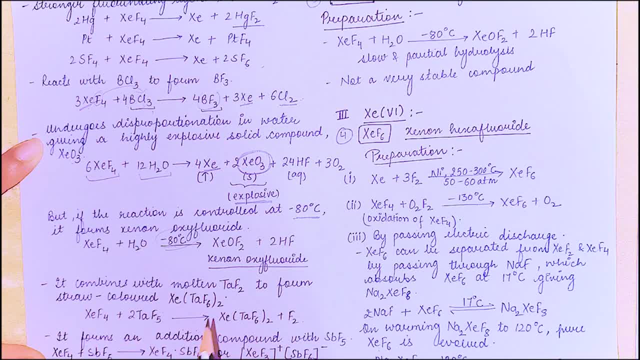 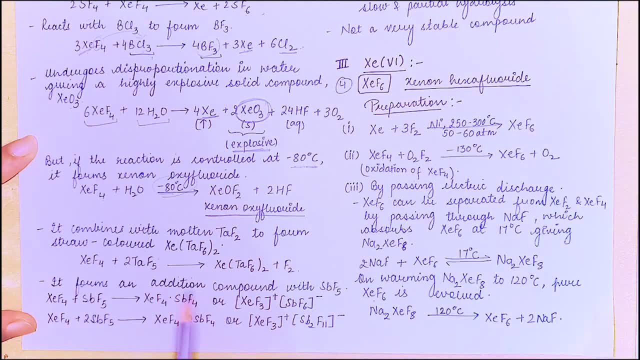 plus HF, right it combines with molten plus HF, right it combines with molten. taf2 to form straw colored xenon compound. taf2 to form straw colored xenon compound. taf2 to form straw colored xenon compound which is XE, PA, f6, whole twice alright. so 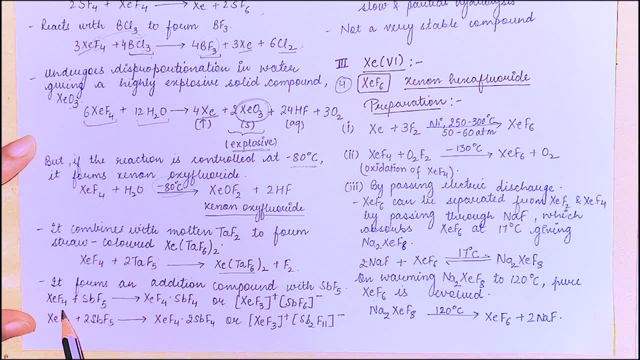 which is XE PA f6 whole, twice alright. so which is XE PA f6 whole, twice alright. so this is a reaction, it forms an addition. this is a reaction, it forms an addition. this is a reaction, it forms an addition. compound with SB f5, XE f4 plus XE SB f5. 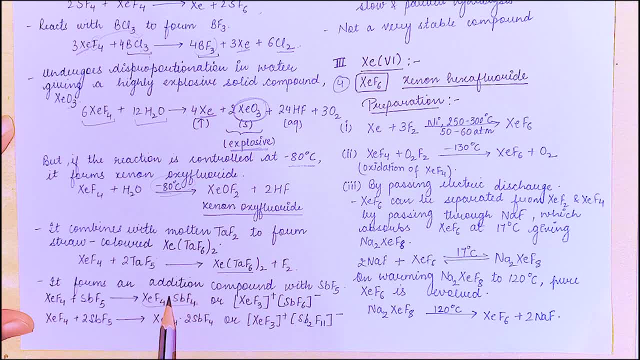 compound with SB f5: XE f4 plus XE SB f5. compound with SB f5: XE f4 plus XE SB f5. is this compound? this is an addition. is this compound? this is an addition. is this compound? this is an addition compound. just put a dot between both the. 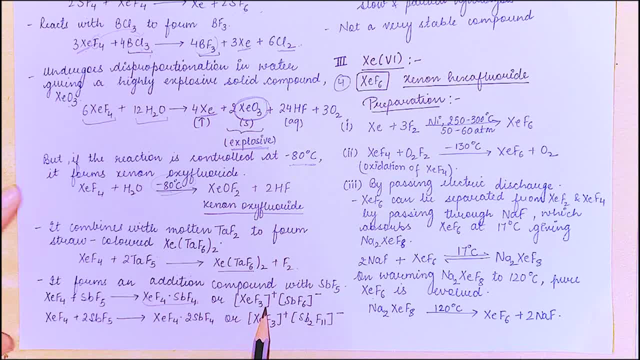 compound. just put a dot between both the compound. just put a dot between both the compounds. or you can show that in form compounds, or you can show that in form compounds, or you can show that in form of ions also. that is just remove one of ions also. that is just remove one. 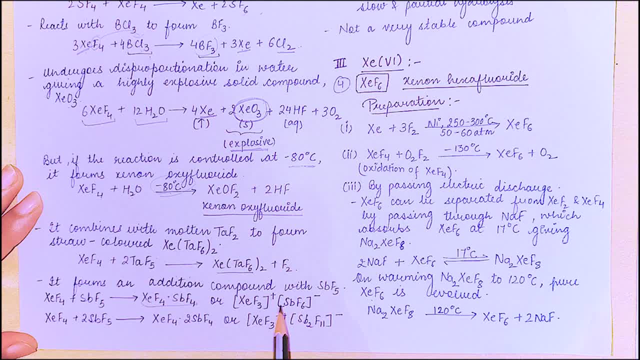 of ions also. that is: just remove one fluorine from here- yet XE f3 positive fluorine from here. yet XE f3 positive fluorine from here, yet XE f3 positive. and add one fluorine- here we have fx SB. and add one fluorine- here, we have fx SB. 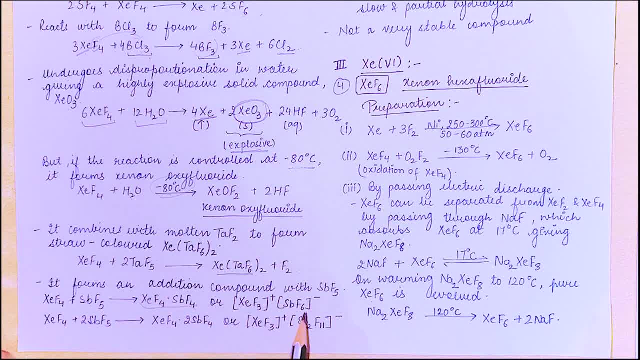 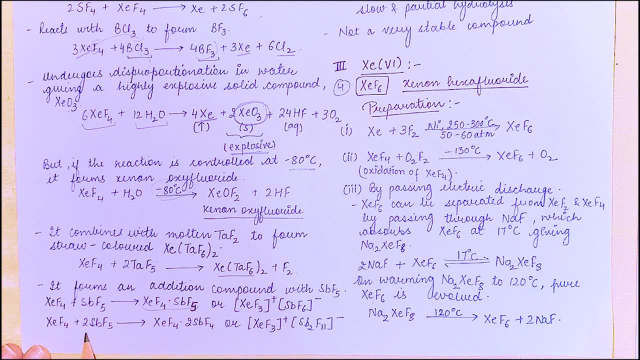 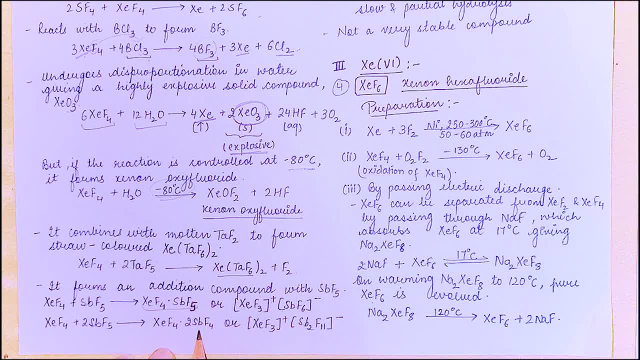 it's five, right. so XE f4 plus two SB f5. yes, XE f4 plus two SB f5. here also. so yes, XE f4 plus two SB f5. here also. so yes, XE f4 plus two SB f5. here also. so when one hydrogen fluorine is removed. 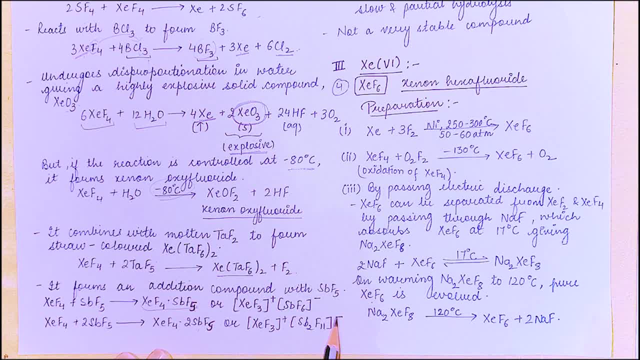 when one hydrogen fluorine is removed. when one hydrogen fluorine is removed from here it gets positive charge, and on from here it gets positive charge, and on from here it gets positive charge. and on addition of one fluorine: here it gets a. addition of one fluorine, here it gets a. 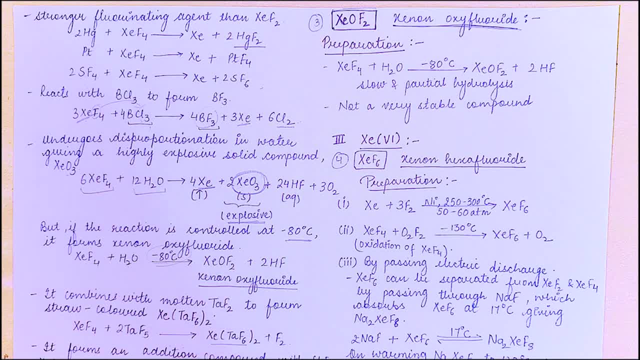 addition of one fluorine. here it gets a negative charge. so the next compound is negative charge. so the next compound is negative charge. so the next compound is xenon oxy fluoride. it is prepared by slow xenon oxy fluoride. it is prepared by slow xenon oxy fluoride. it is prepared by slow and partial hydrolysis of XE f4, that is. 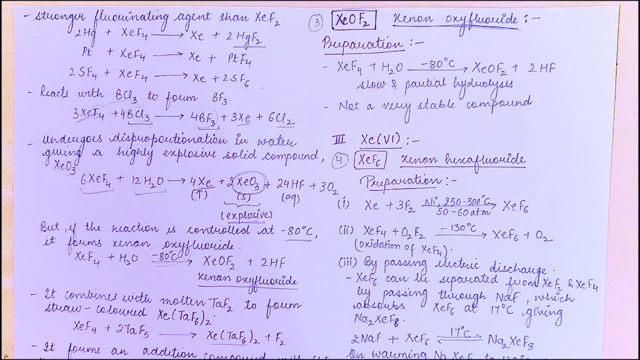 and partial hydrolysis of XE f4. that is, and partial hydrolysis of XE f4. that is the compound we have just prepared in the compound we have just prepared in the compound we have just prepared in the previous reactions. it is xenon. 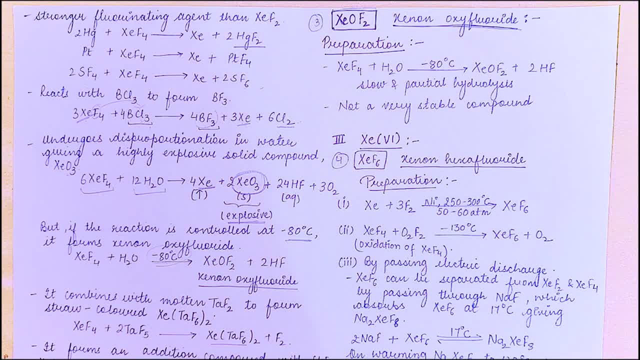 the previous reactions. it is xenon. the previous reactions: it is xenon tetrafluoride. so by slow and partial tetrafluoride, so by slow and partial tetrafluoride, so by slow and partial hydrolysis of xenon tetrafluoride at low. 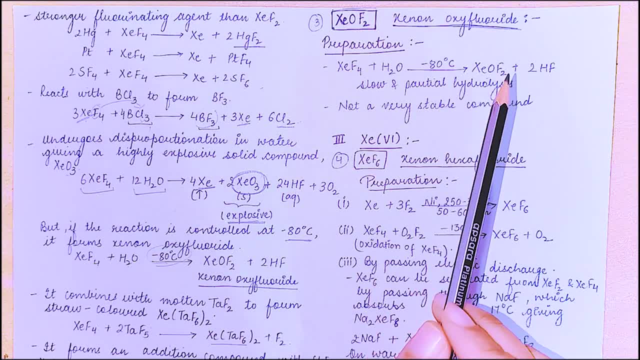 hydrolysis of xenon tetrafluoride at low hydrolysis of xenon tetrafluoride at low temperature. we can get xenon oxy temperature. we can get xenon oxy temperature. we can get xenon oxy fluoride. all right, so it is not a very 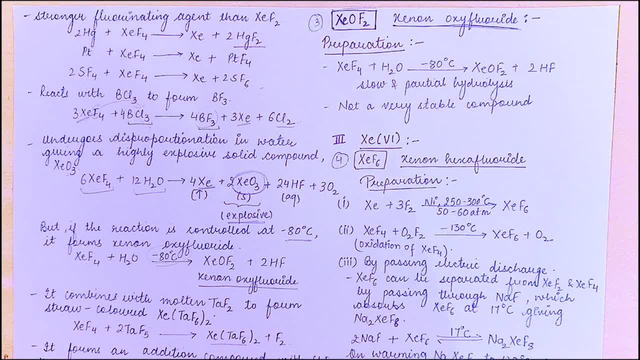 fluoride. all right, so it is not a very fluoride. all right, so it is not a very stable compound. the structures of all stable compound. the structures of all stable compound, the structures of all these compounds. we are going to do at these compounds, we are going to do at. 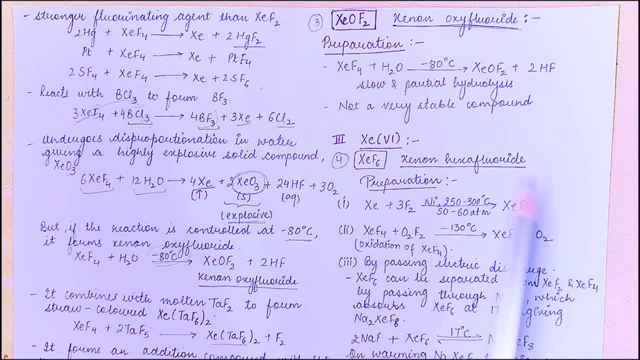 these compounds we are going to do at the end, all right. so next we have xenon, the end. all right. so next we have xenon, the end, all right. so next we have xenon, in plus six oxidation state- the first, in plus six oxidation state, the first. 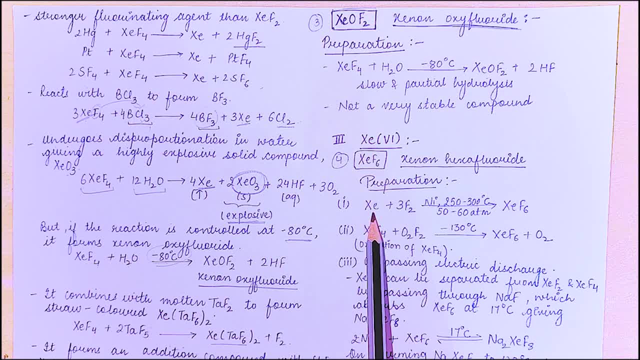 in plus six oxidation state. the first compound is xenon hexafluoride compound. is xenon hexafluoride compound. is xenon hexafluoride preparation. xenon plus fluorine gives preparation. xenon plus fluorine gives preparation. xenon plus fluorine gives XE f6 at 250 to 300 degrees. 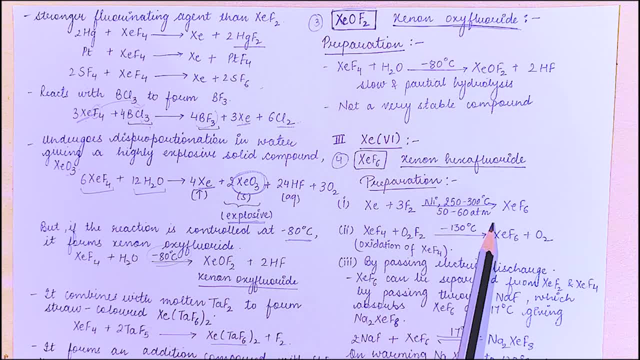 XE f6 at 250 to 300 degrees. XE f6 at 250 to 300 degrees Celsius and in the presence of nickel Celsius, and, in the presence of nickel Celsius, and in the presence of nickel vessel right, at 50 to 60 atmosphere. 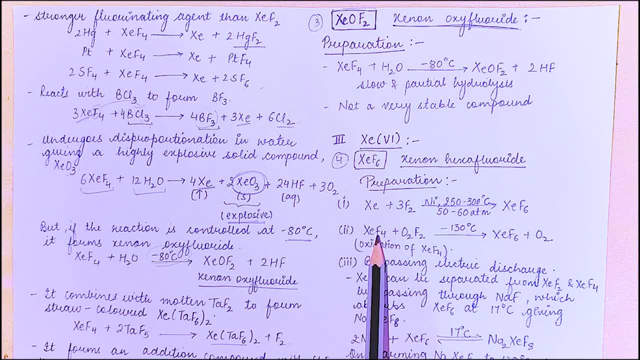 vessel right at 50 to 60 atmosphere vessel right at 50 to 60 atmosphere pressure. so these conditions are pressure, so these conditions are pressure, so these conditions are important to perform the reaction next. important to perform the reaction next. important to perform the reaction next. we have xenon tetrafluoride plus o2 f2. 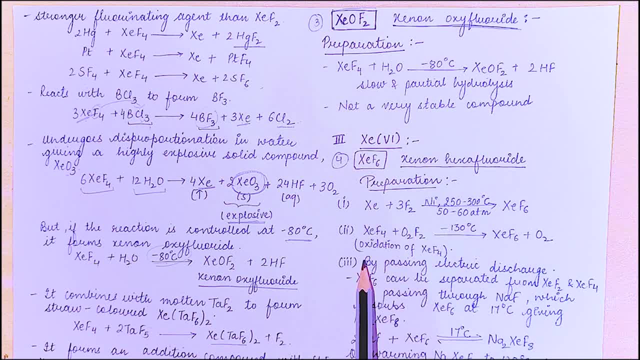 we have xenon tetrafluoride plus o2 f2. we have xenon tetrafluoride plus o2 f2 at minus 130 degrees Celsius. forms at minus 130 degrees Celsius. forms at minus 130 degrees Celsius forms. xenon hexafluoride plus oxygen. this is 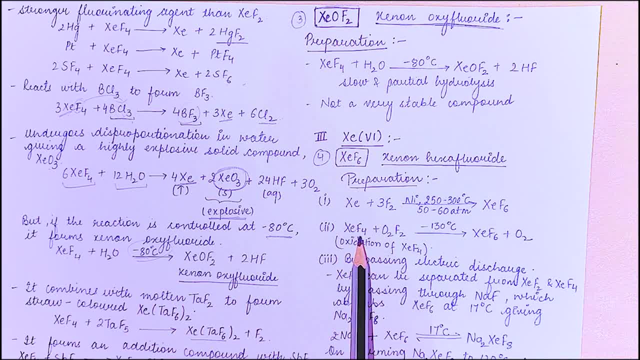 xenon hexafluoride plus oxygen. this is xenon hexafluoride plus oxygen. this is called oxidation of xenon tetrafluoride, called oxidation of xenon tetrafluoride, called oxidation of xenon tetrafluoride. as you can see that we are oxidizing it. 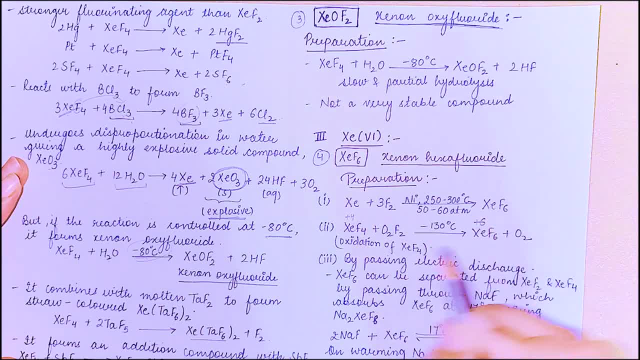 as you can see that we are oxidizing it. as you can see that we are oxidizing it to xenon from plus 4 oxidation state 2 to xenon from plus 4 oxidation state 2 to xenon from plus 4 oxidation state 2 plus 6 oxidation state. so this is an 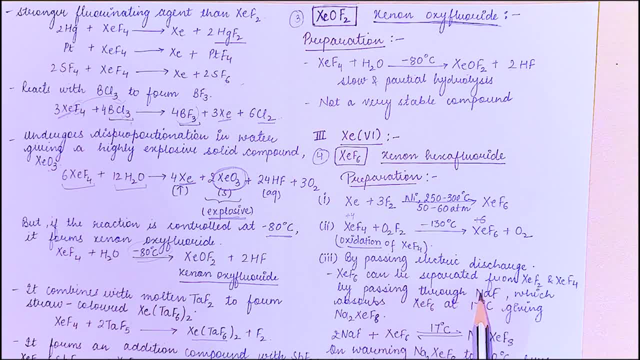 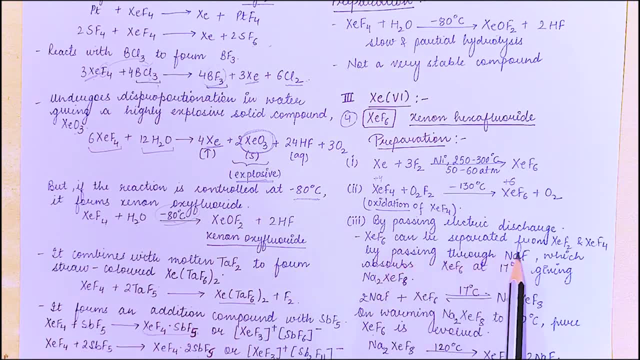 plus 6 oxidation state. so this is an plus 6 oxidation state. so this is an oxidation right by passing electric oxidation, right by passing electric oxidation, right by passing electric discharge, as we have read in all other discharge, as we have read in all other discharge, as we have read in all other reactions also. right next we have XE f6. 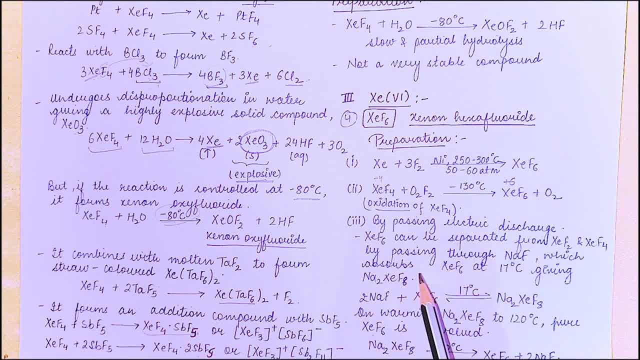 reactions also. right next we have XE f6. reactions also. right next we have XE f6. can be separated from XE f2 and XE f4 by. can be separated from XE f2 and XE f4 by. can be separated from XE f2 and XE f4 by passing through naf, which absorbs xenon. 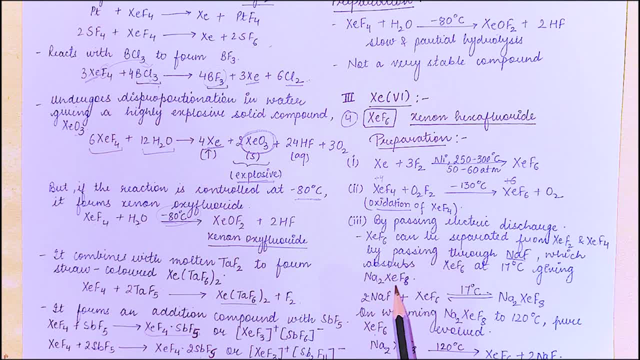 passing through naf, which absorbs xenon. passing through naf, which absorbs xenon, hexafluoride at 17 degree Celsius. giving hexafluoride at 17 degree Celsius. giving hexafluoride at 17 degree Celsius. giving na2 XE f8, so we can separate XE f6 two. 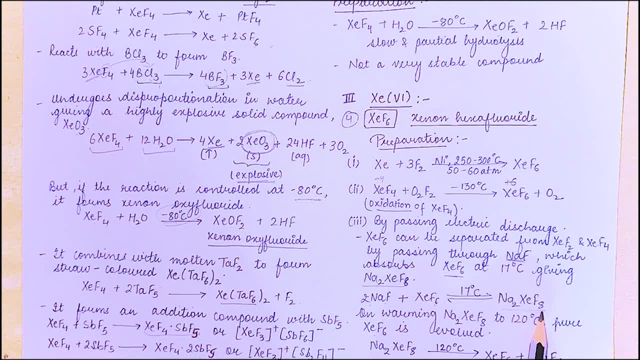 na2 XE f8, so we can separate XE f6 two na2 XE f8, so we can separate XE f6- two molecules of naf in the presence of this molecules of naf in the presence of this molecules of naf. in the presence of this, yes, the compound to separate the xenon. 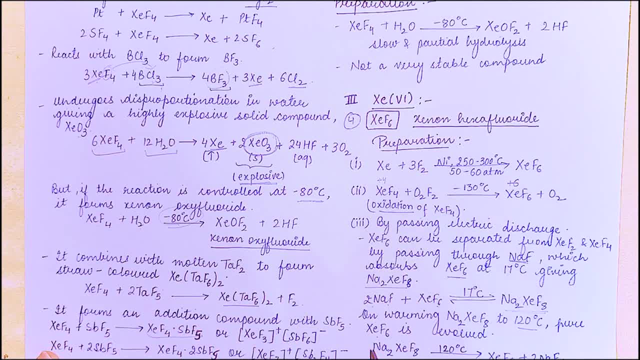 yes, the compound to separate the xenon. yes, the compound to separate the xenon: hexafluoride. on warming this at 120 hexafluoride. on warming this at 120 hexafluoride. on warming this at 120 degrees Celsius: pure xenon hexafluoride. 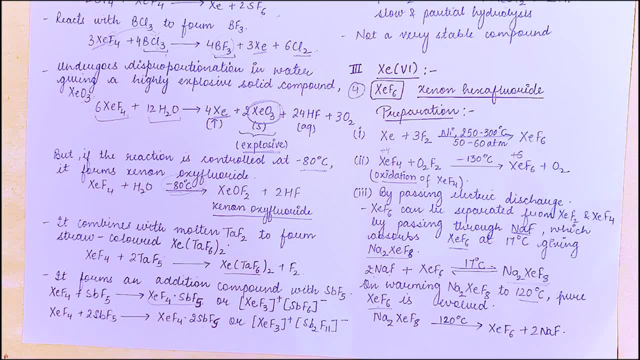 degrees Celsius, pure xenon hexafluoride. degrees Celsius: pure xenon hexafluoride is evolved. so this is a way to separate. is evolved. so this is a way to separate. is evolved. so this is a way to separate xenon hexafluoride. let's see the 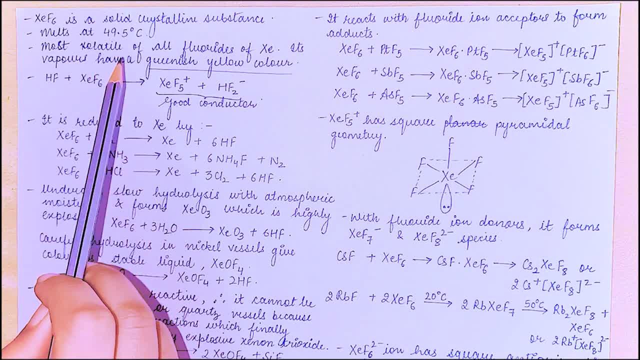 xenon hexafluoride. let's see the xenon hexafluoride. let's see the properties. it is a solid crystalline properties. it is a solid crystalline properties. it is a solid crystalline substance. it melts at 49.5 degrees. substance: it melts at 49.5 degrees. substance: it melts at 49.5 degrees Celsius. it is most volatile of all Celsius. it is most volatile of all Celsius. it is most volatile of all. fluorides of xenon: its vapors have a. fluorides of xenon: its vapors have a. 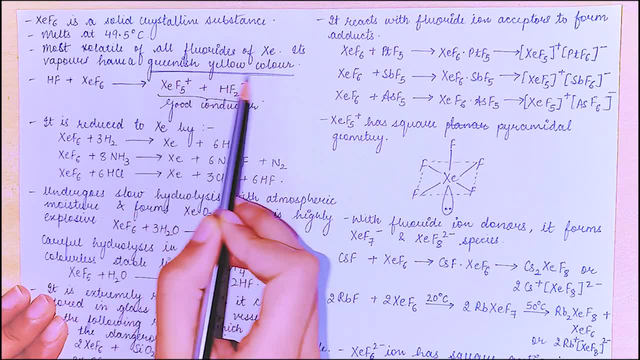 fluorides of xenon, its vapors have a greenish yellow color. so these are the greenish yellow color. so these are the greenish yellow color. so these are the points through which you can remember, points through which you can remember, points through which you can remember which compound was performing which. 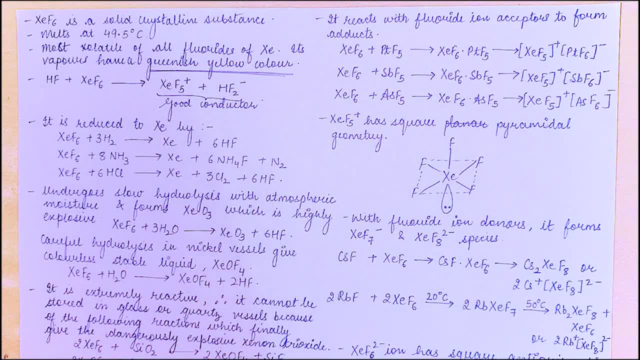 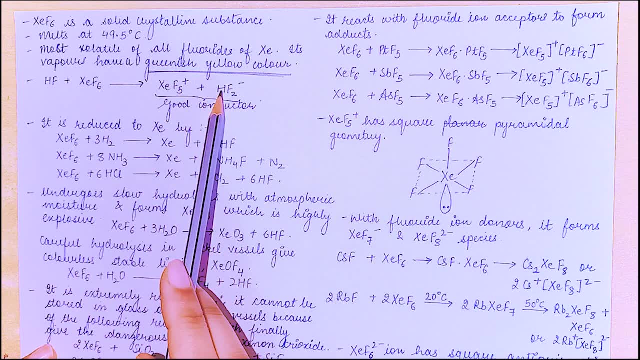 which compound was performing, which which compound was performing which reactions just correlated with their reactions, just correlated with their reactions, just correlated with their colors, and you will be able to remember colors and you will be able to remember colors and you will be able to remember the compounds: HF plus XE, f6 forms, XE, f5. 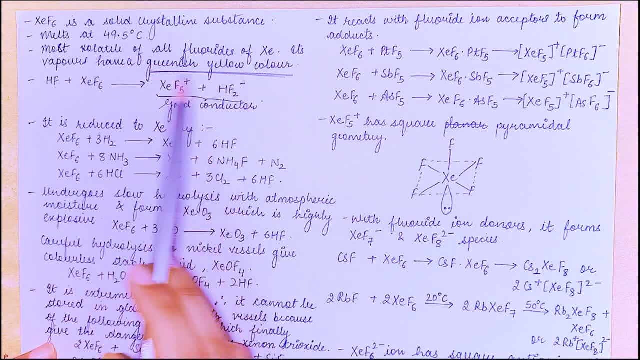 the compounds HF plus XE f6 forms XE f5. the compounds HF plus XE f6 forms XE f5. positive plus HF to negative, so it is a positive plus HF to negative, so it is a positive plus HF to negative, so it is a good conductor because it is forming. 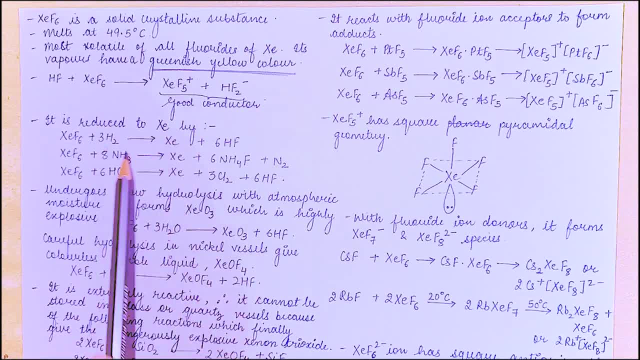 good conductor because it is forming good conductor because it is forming ions. right. it is reduced to xenon by ions- right. it is reduced to xenon by ions right. it is reduced to xenon by hydrogen ammonia- HCL- right, so it forms hydrogen ammonia- HCL- right, so it forms. 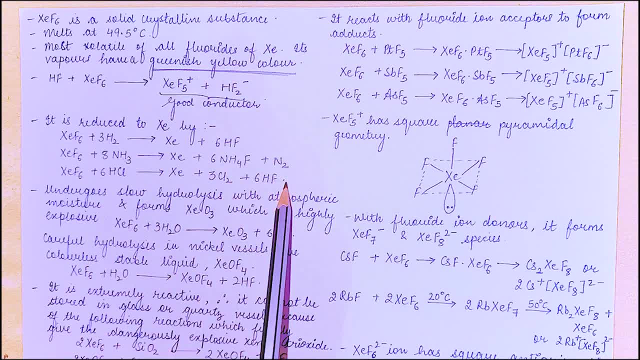 hydrogen ammonia, HCL, right. so it forms xenon plus HF and that's 4f chlorine. xenon plus HF and that's 4f chlorine. xenon plus HF and that's 4f chlorine, etc. it undergoes slow hydrolysis with, etc. it undergoes slow hydrolysis with. 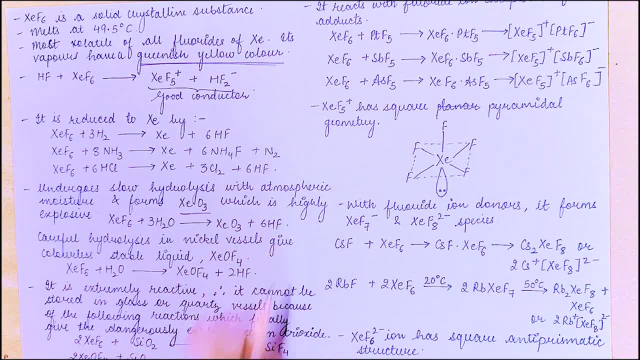 etc. it undergoes slow hydrolysis with atmospheric moisture and forms XCO 3 atmospheric moisture and forms XCO 3 atmospheric moisture and forms XCO 3, which is highly explosive. this is also we which is highly explosive. this is also we which is highly explosive. this is also we have already done one explosive. 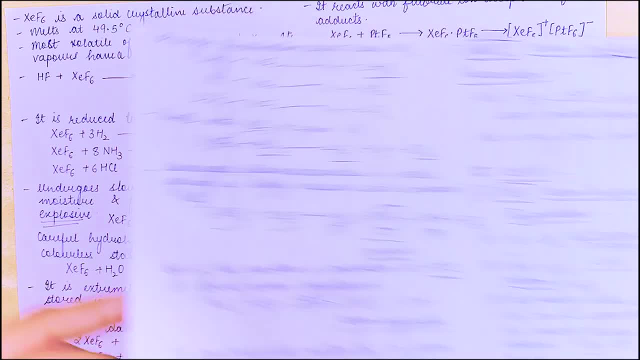 have already done one explosive, have already done one explosive compound reaction. let's see this one compound reaction. let's see this one compound reaction. let's see this one: here also, XCO 3 was formed, which was here also. XCO 3 was formed, which was. 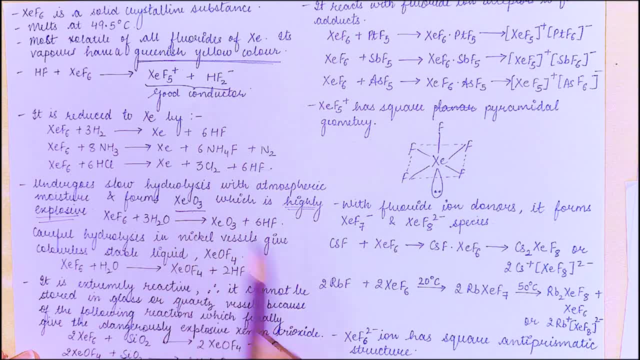 here also XCO 3 was formed, which was explosive. now in this reaction also, we explosive. now in this reaction also we explosive. now in this reaction also we get XCO 3, which is explosive, so just get XCO 3, which is explosive, so just. 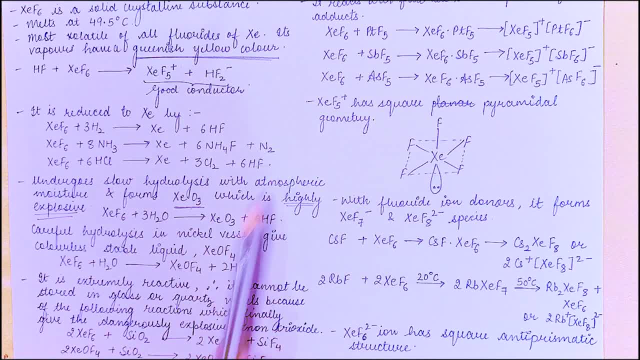 get XCO 3, which is explosive. so just remember if explosive compound is being remember, if explosive compound is being remember, if explosive compound is being asked or the reaction is being asked- so asked. or the reaction is being asked- so asked, or the reaction is being asked. so just remember that they are talking about. 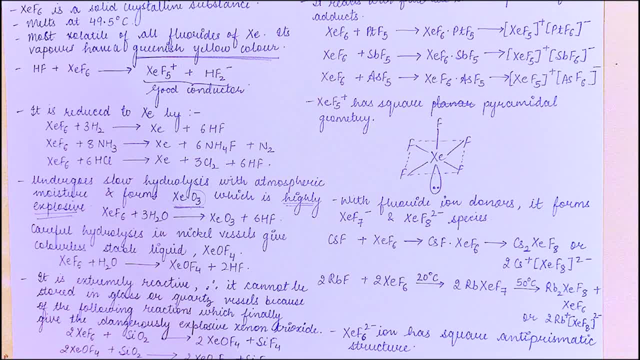 just remember that they are talking about. just remember that they are talking about XCO 3, just remember that they are talking about XCO 3. right, and therefore we have to be right and therefore we have to be right and therefore we have to be carefully. hydraulic hydrolyzed in nickel. 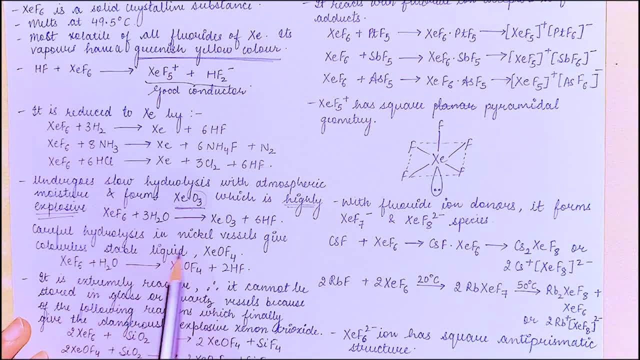 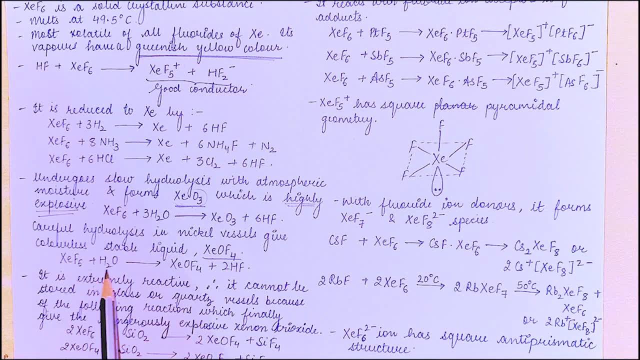 carefully hydraulic hydrolyzed in nickel. carefully hydraulic hydrolyzed in nickel vessel. right so careful hydrolysis in vessel. right so careful hydrolysis in vessel. right so careful hydrolysis in nickel vessel. give colorless, stable nickel vessel. give colorless, stable nickel vessel. give colorless, stable liquid which is XCO, f4, X, C, f6, plus water. 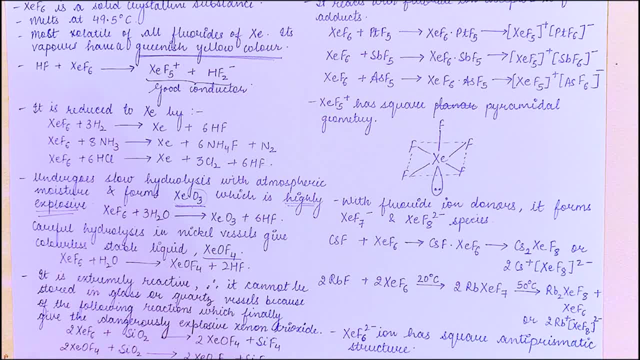 liquid which is XCO f4, X C f6 plus water. liquid which is XCO f4, X C f6 plus water, gives X E o f4 plus 2 HF. it is gives X E o f4 plus 2 HF. it is gives X E o f4 plus 2 HF. it is extremely reactive. therefore it cannot be. 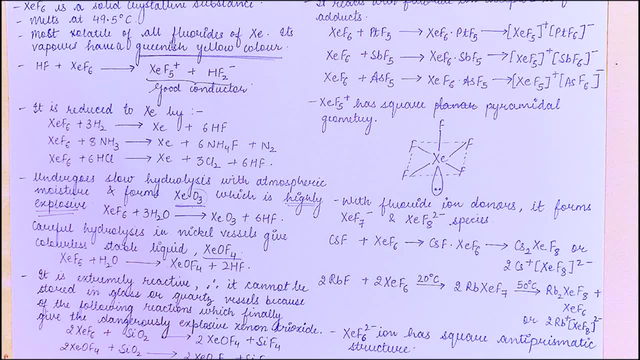 extremely reactive. therefore, it cannot be extremely reactive. therefore, it cannot be stored in, stored in, stored in glass or quartz vessel because of the glass or quartz vessel, because of the glass or quartz vessel, because of the falling reactions which finally give the falling reactions which finally give the 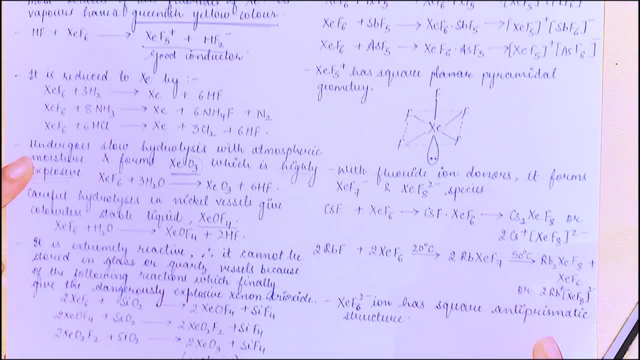 falling reactions which finally give the dangerous explosive xenon trioxide. this dangerous explosive xenon trioxide, this dangerous explosive xenon trioxide. this one right, so let's see which reactions. one right, so let's see which reactions. one right, so let's see which reactions they're talking about. it is X, C, f6, on. 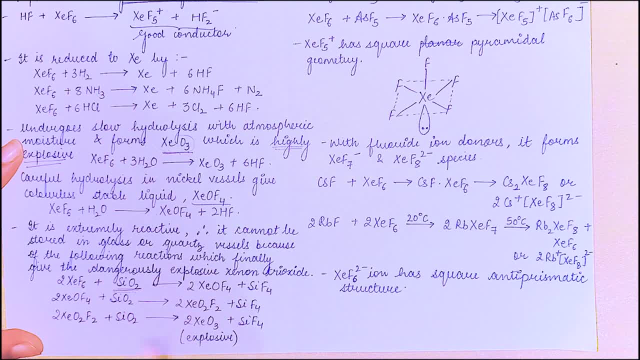 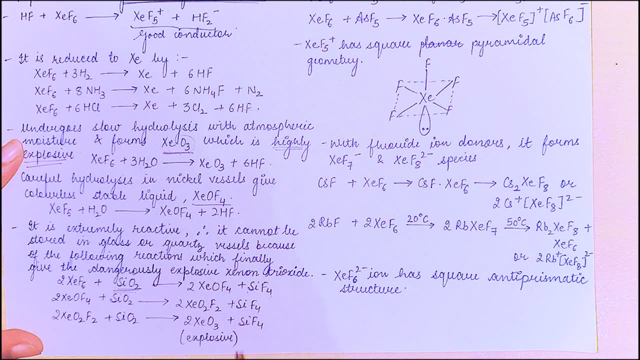 they're talking about. it is X C f6 on. they're talking about. it is X C f6 on. reaction with the two silica quads glass. reaction with the two silica quads glass. reaction with the two silica quads glass. right, so we get X E o f4 plus si f4. 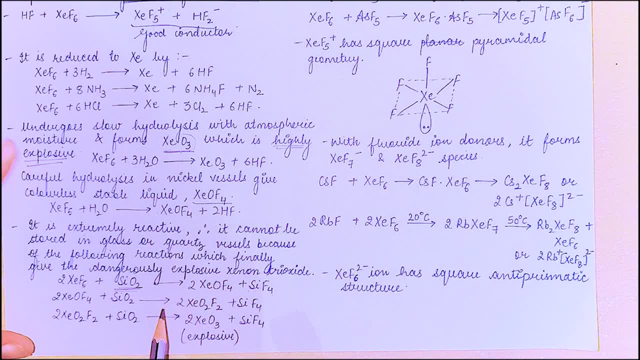 right, so we get X E o f4 plus si f4. right, so we get X E o f4 plus si f4. now this, okay. now this okay. now this, okay, how to remember these reactions in this, how to remember these reactions in this, how to remember these reactions in this reaction. you can see that there are six. 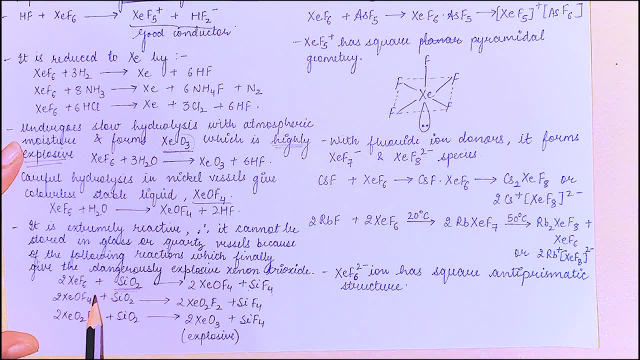 reaction. you can see that there are six reaction. you can see that there are six fluorines. if it okay, do you know what is fluorines? if it okay, do you know what is fluorines? if it okay, do you know what is the valency of fluorine and what is the? 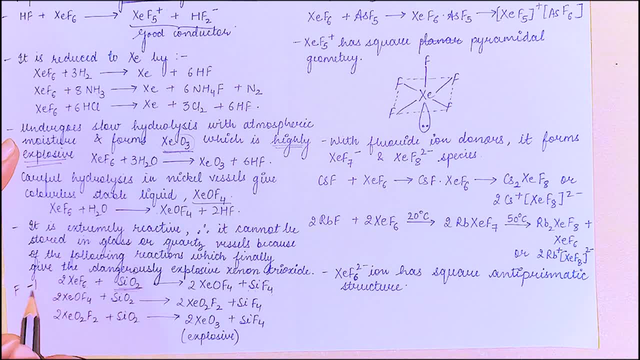 the valency of fluorine and what is the the valency of fluorine and what is the valency of oxygen? valency of fluorine is valency of oxygen. valency of fluorine is: valency of fluorine is minus one and for oxygen it is minus two. 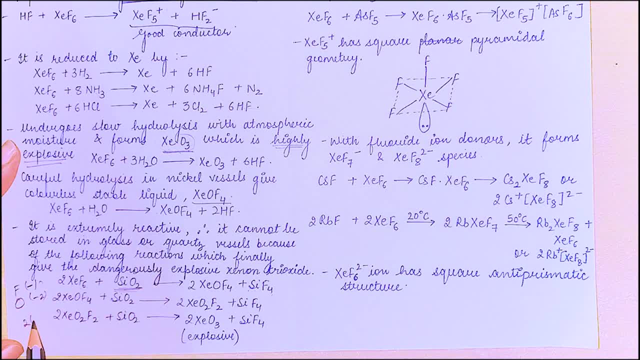 minus one, and for oxygen it is minus two. minus one, and for oxygen, it is minus two. right? so if we do two times the valency, right. so if we do two times the valency, right. so if we do two times the valency of fluorine, we get the valency of. 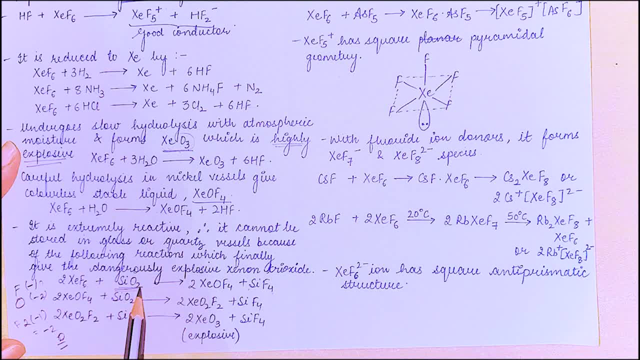 of fluorine, we get the valency of of fluorine, we get the valency of oxygen. so if you remove two fluorines and oxygen, so if you remove two fluorines and oxygen, so if you remove two fluorines and add one oxygen, we get the same. 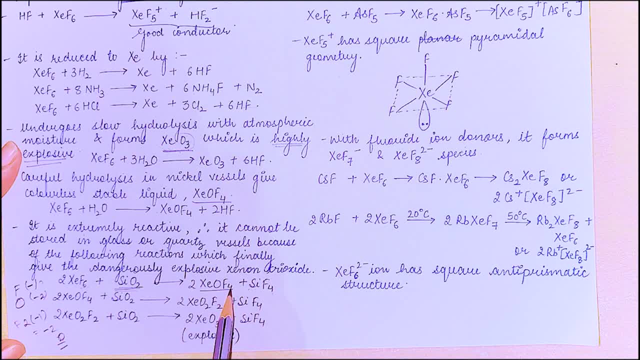 add one oxygen, we get the same. add one oxygen, we get the same. oxidation states of oil. so here if we oxidation states of oil, so here if we oxidation states of oil. so here, if we have removed two fluorines, we get four. have removed two fluorines, we get four. 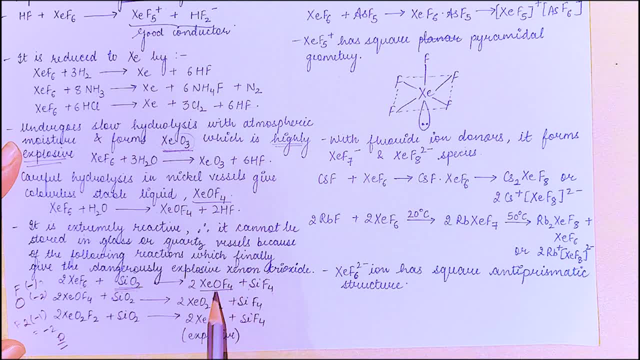 have removed two fluorines, we get four, and we have added one oxygen in place of, and we have added one oxygen in place of, and we have added one oxygen in place of those two fluorines. just this is it to those two fluorines. just this is it to. 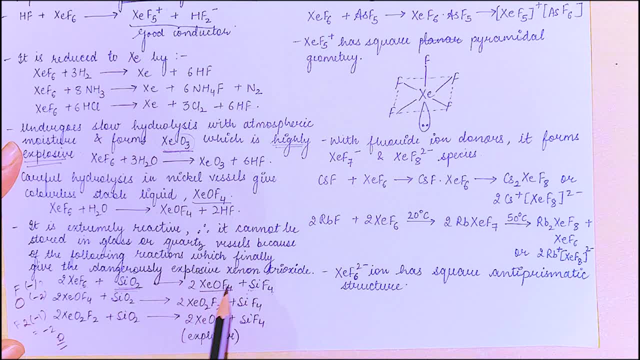 those two fluorines. just this is it to remember, right? so we get a si f4. now this, remember right. so we get a si f4 now this, remember right. so we get a si f4 now this compound. again, we remove two fluorine compound. again, we remove two fluorine. 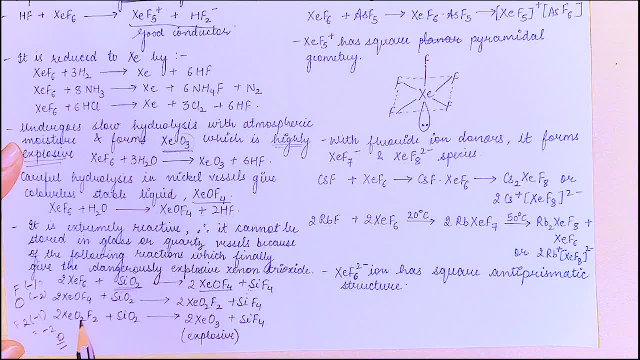 compound. again we remove two fluorine, add one oxygen XC to f2 fair. then again add one oxygen XC to f2 fair. then again add one oxygen XC to f2 fair. then again we remove two hydrofluorines and add one. we remove two hydrofluorines and add one. 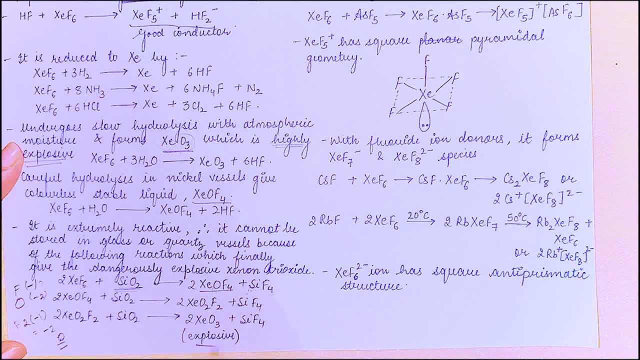 we remove two hydrofluorines and add one oxygen, we get XCO 3, the compound oxygen. we get XCO 3, the compound oxygen. we get XCO 3, the compound. which is explosive. all right, it reacts with. which is explosive, all right, it reacts with. 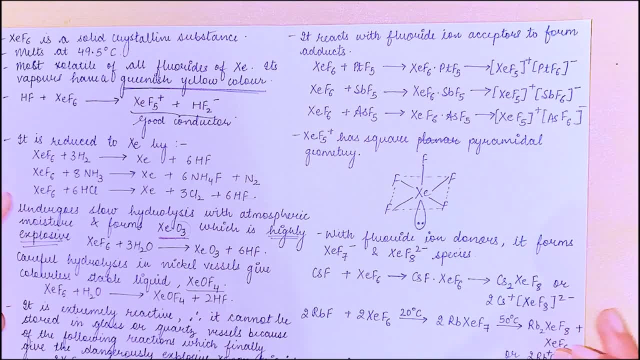 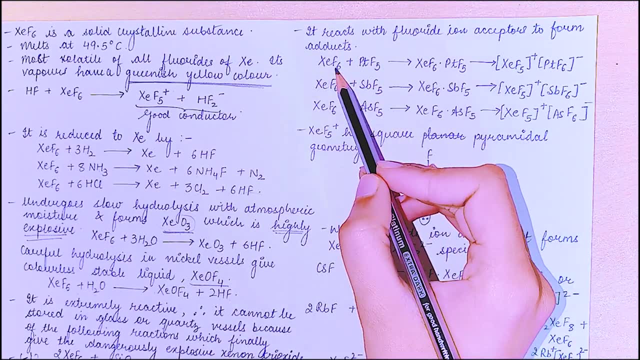 which is explosive. all right, it reacts with fluorine fluoride ion. fluorine fluoride ion. fluorine fluoride ion. it reacts with fluoride ion acceptors to it. reacts with fluoride ion acceptors to it. reacts with fluoride ion acceptors to form adults. right, so this is XC f6 plus. 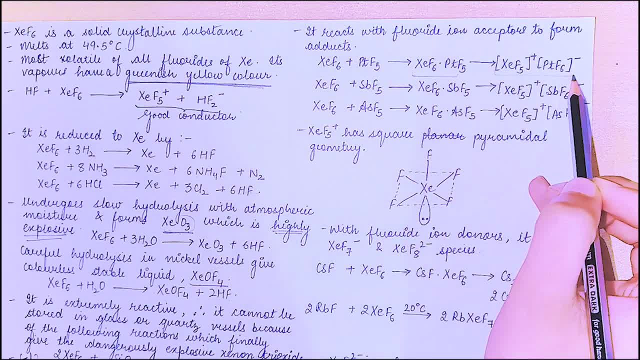 form adults, right? so this is XC f6 plus form adults, right? so this is XC f6 plus PTF 5 and it forms adapts on the ionic PTF 5 and it forms adapts on the ionic PTF 5 and it forms adapts on the ionic form of this and the same reaction goes. 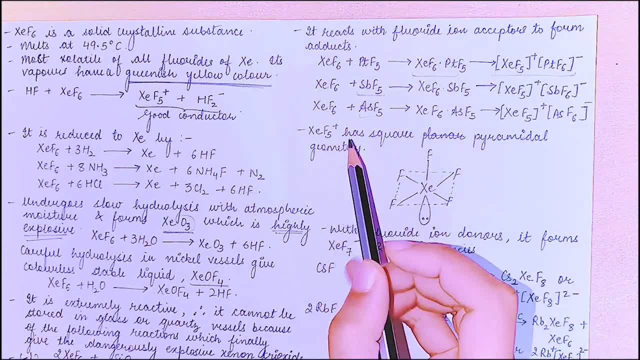 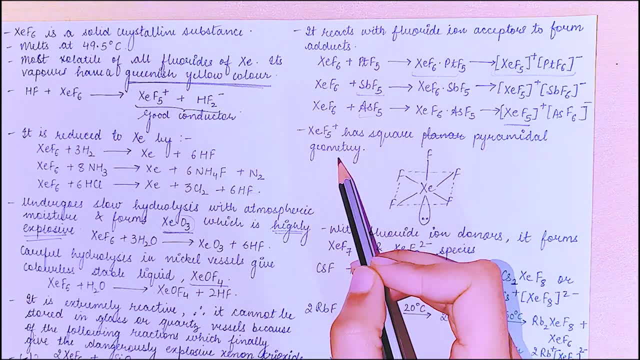 form of this and the same reaction goes. form of this and the same reaction goes with antimony arsenic. next we have any with antimony arsenic, next we have any with antimony arsenic, next we have any f5 positive. this one has square pyramidal. 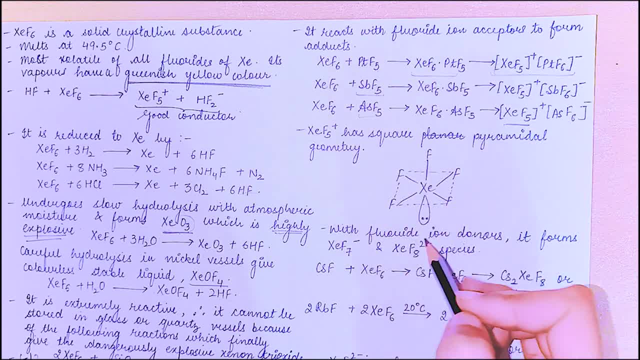 f5 positive. this one has square pyramidal. f5 positive. this one has square pyramidal geometry. it has a square pyramidal geometry. it has a square pyramidal geometry. it has a square pyramidal geometry. you can see with fluoride and 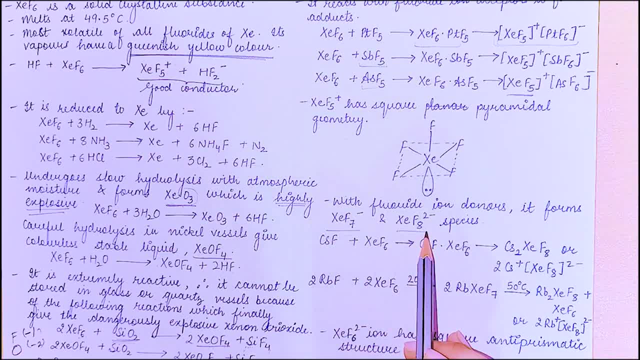 geometry you can see with fluoride and geometry you can see with fluoride and donors. it forms XE f7 negative and XE f8 donors. it forms XE f7 negative and XE f8 donors. it forms XE f7 negative and XE f8 to negative species. excision fluoride. 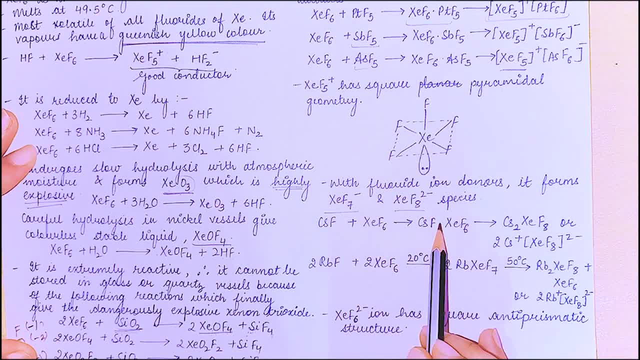 to negative species: excision fluoride to negative species: excision fluoride: plus XE f6 gives cesium dot. XE f6- adapt. plus XE f6 gives cesium dot. XE f6- adapt. plus XE f6 gives cesium dot. XE f6- adapt. or you can see this in an: in an ionic. 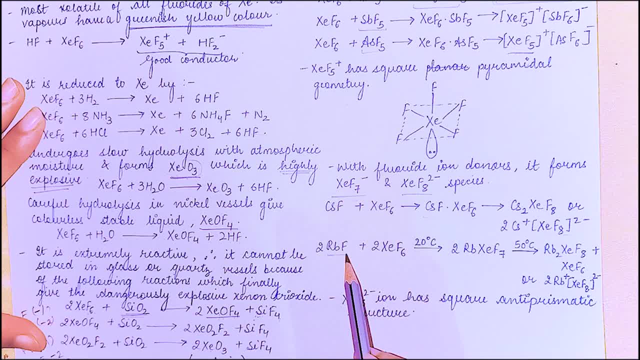 or you can see this in an in an ionic, or you can see this in an in an ionic forms game: the reaction with the medium forms game, the reaction with the medium forms game, the reaction with the medium, and it also has a square and it also has a square. 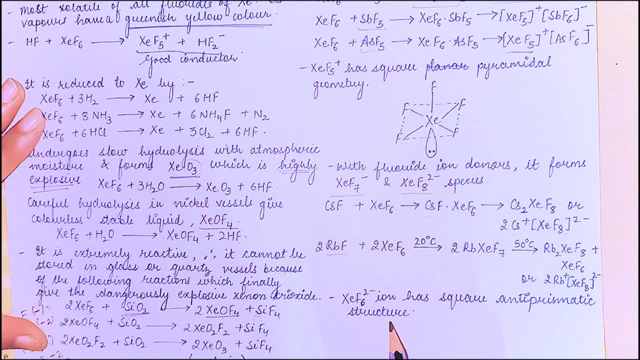 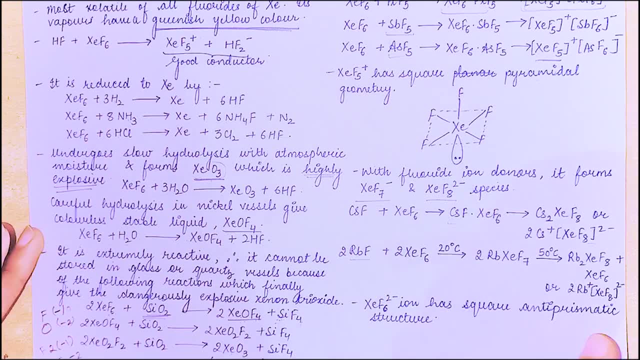 and it also has a square anti prismatic structure. the structures of anti prismatic structure. the structures of anti prismatic structure, the structures of all compounds. I have already told you all compounds. I have already told you all compounds. I have already told you that we are going to do that at the end. 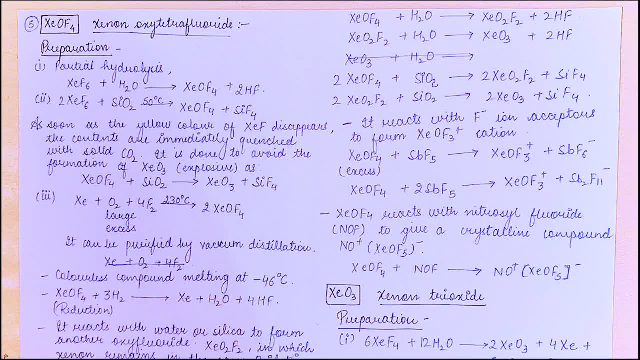 that we are going to do that at the end, that we are going to do that at the end. we have already done four compounds. this: we have already done four compounds. this: we have already done four compounds. this is the fifth compound: XCO, f4, xenon. 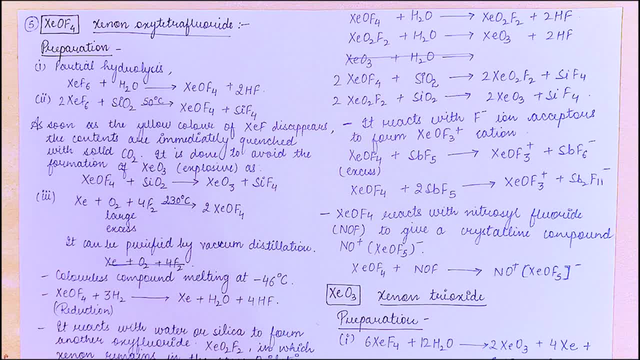 is the fifth compound. XCO f4- xenon is the fifth compound: XCO f4- xenon. oxytetrafluoride by partial hydrolysis of oxytetrafluoride, by partial hydrolysis of oxytetrafluoride, by partial hydrolysis of xenon hexafluoride, we get XCO f4 plus HF. 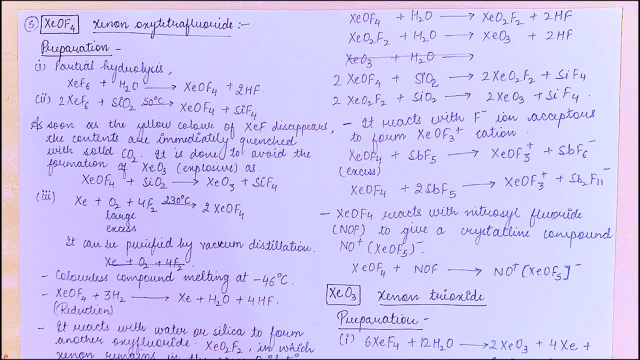 xenon hexafluoride, we get XCO f4 plus HF. xenon hexafluoride, we get XCO f4 plus HF. then on reacting with SiO2, it gives, then on reacting with SiO2, it gives, then on reacting with SiO2, it gives again, gives that product XCO f4 as. 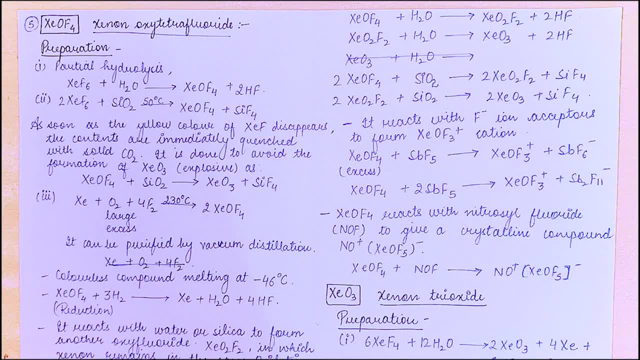 again gives that product XCO f4, as again gives that product XCO f4. as soon as the yellow color of XCF, soon as the yellow color of XCF, soon as the yellow color of XCF disappears, the contents are immediately. disappears, the contents are immediately. 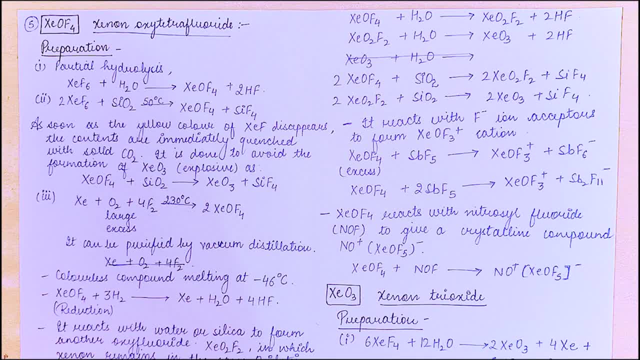 disappears, the contents are immediately quenched with solid carbon dioxide. it is quenched with solid carbon dioxide. it is quenched with solid carbon dioxide. it is done to avoid the formation of the done, to avoid the formation of the done, to avoid the formation of the explosive compound. you must remember this. 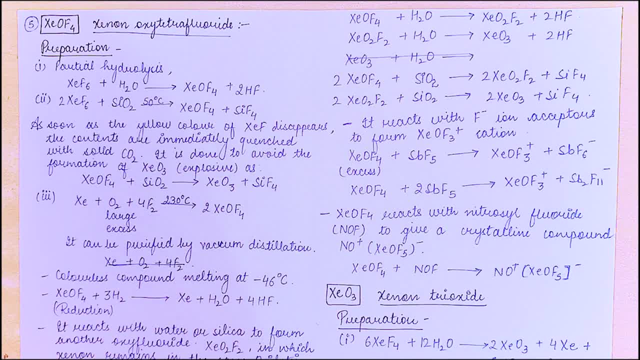 explosive compound. you must remember this explosive compound, you must remember this. XCO 3- XCO 3: this is explosive right. XCO 3- XCO 3: this is explosive right. XCO 3- XCO 3: this is explosive right. it is XCO f4 plus SiO2 gives XCO 3 plus. 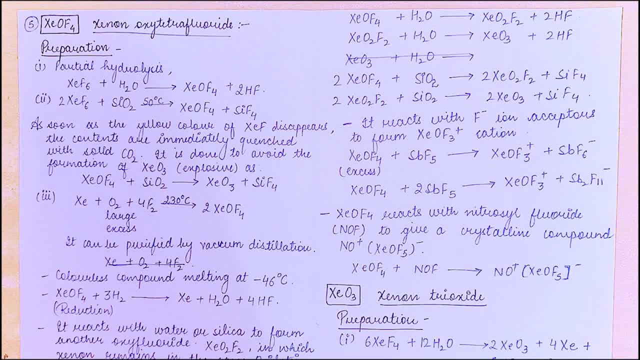 it is XCO f4 plus SiO2 gives XCO 3 plus. it is XCO f4 plus SiO2 gives XCO 3 plus. SiF4 xenon in presence of large excess. SiF4 xenon in presence of large excess. 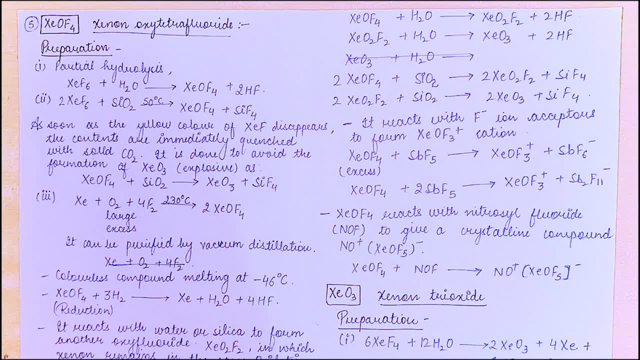 SiF4 xenon in presence of large excess of oxygen plus fluorine at a temperature of oxygen plus fluorine at a temperature of oxygen plus fluorine at a temperature of 230 degrees Celsius. yes, XCO f4 so of 230 degrees Celsius. yes, XCO f4 so. 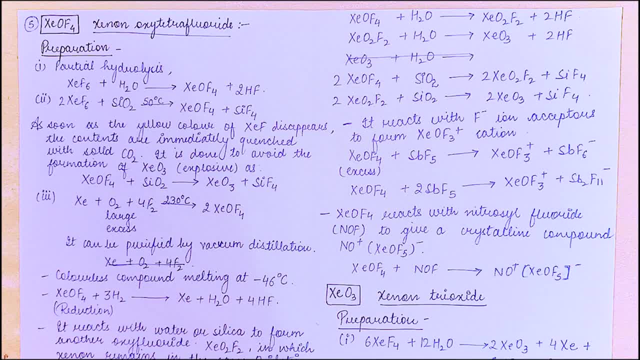 of 230 degrees Celsius. yes, XCO f4. so these are three types in which you can. these are three types in which you can. these are three types in which you can prepare xenon oxy tetrafluoride. it can. prepare xenon oxy tetrafluoride. it can. 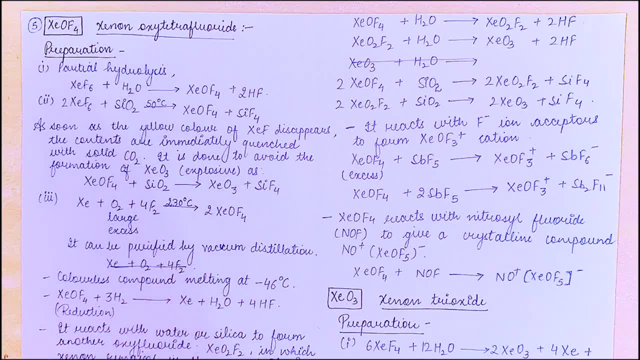 prepare xenon oxy tetrafluoride. it can be prepared by vacuum distillation in. be prepared by vacuum distillation in. be prepared by vacuum distillation in this reaction: right next we have. it is a this reaction. right next we have. it is a this reaction. right next we have. it is a colorless compound. melting point is: 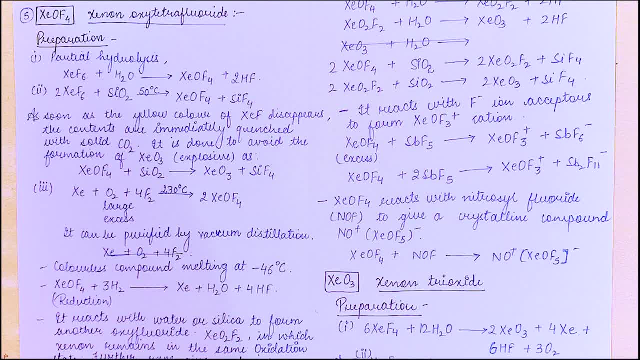 colorless compound melting point is colorless compound. melting point is minus 46 degrees Celsius. it from the minus 46 degrees Celsius. it from the minus 46 degrees Celsius. it from the blue reduction on reaction with the blue reduction on reaction with the blue reduction on reaction with the hydrogen to form xenon. it reacts with. 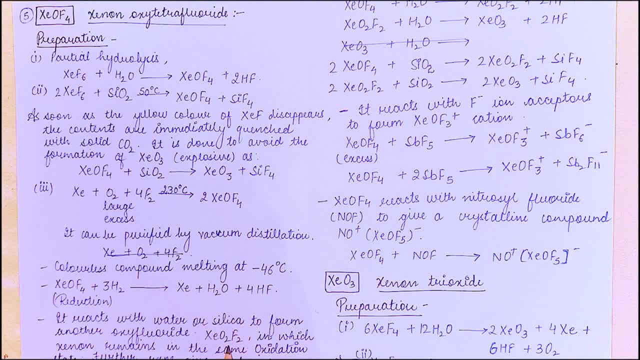 hydrogen to form xenon. it reacts with hydrogen to form xenon. it reacts with water or silica to form another water or silica to form another water or silica to form another oxy fluoride XCO 2- f2. so you can see that in oxy fluoride, XCO 2- f2. so you can see that in. 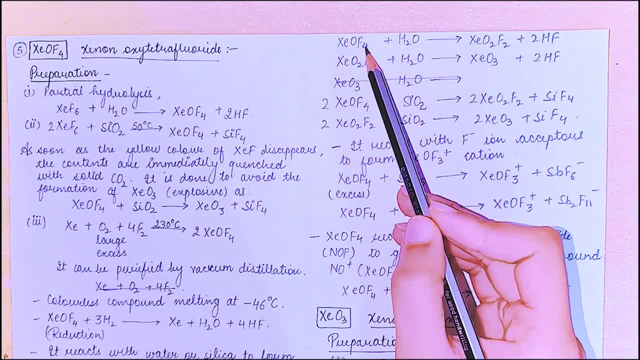 oxy fluoride XCO 2 f2. so you can see that in XCO 4 o f4 there are four fluorines. XCO 4 o f4. there are four fluorines. XCO 4 o f4. there are four fluorines here. so we remove two fluorine, add one. 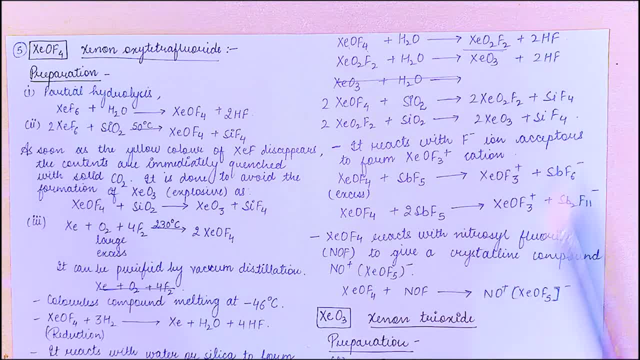 here. so we remove two fluorine. add one here. so we remove two fluorine, add one oxygen. we get XCO 2- f2 in this xenon oxygen. we get XCO 2- f2 in this xenon oxygen. we get XCO 2- f2 in this xenon remains in the same oxidation state. I. 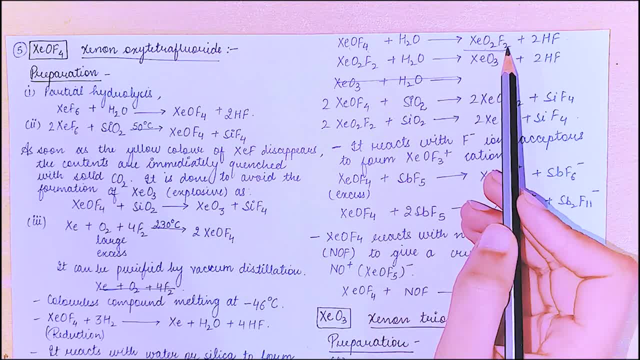 remains in the same oxidation state. I remains in the same oxidation state. I have already told you: furtherings give. have already told you furtherings give. have already told you: furtherings give explosive compound. that means, if we have already told you, furtherings give explosive compound. that means, if we 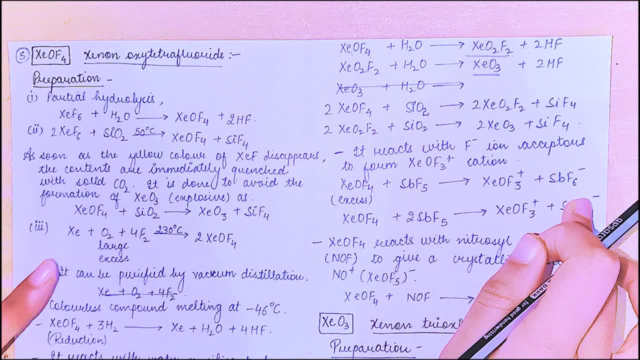 have already told you, furtherings give explosive compound. that means if we fusion, we get the explosive compound and fusion we get the explosive compound, and fusion we get the explosive compound. and similarly on reaction with silica, also similarly on reaction with silica, also similarly on reaction with silica also the same reaction occurs. it reacts with. 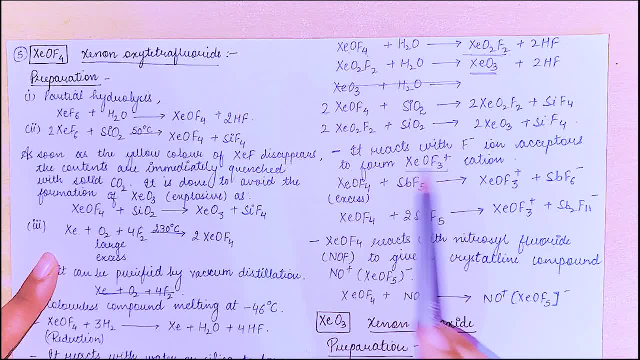 the same reaction occurs. it reacts with the same reaction occurs. it reacts with: fluoride ions. acceptors to form XCO f3. fluoride ions. acceptors to form XCO f3. fluoride ions. acceptors to form XCO f3. positive cation. right on addition of: 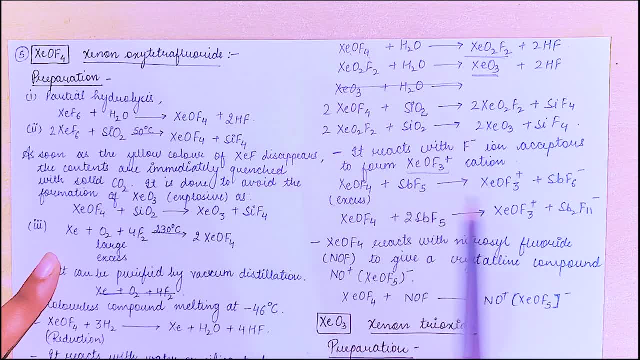 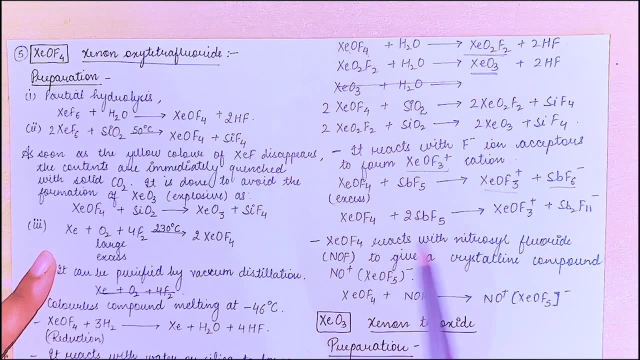 positive cation right on addition of positive cation right. on addition of excess XU f4 plus SPF 5. we get this XU excess XU f4 plus SPF 5. we get this XU excess XU f4 plus SPF 5. we get this XU f3 positive plus SPF 6. negative XCO f4. 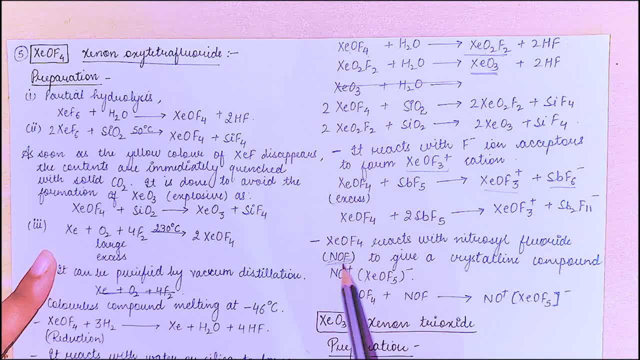 f3 positive plus SPF 6 negative XCO f4. f3 positive plus SPF 6 negative XCO. f4. reacts with nitrosyl to ride and no F reacts with nitrosyl to ride and no F reacts with nitrosyl to ride and no F to give crystalline compound. n? o positive. 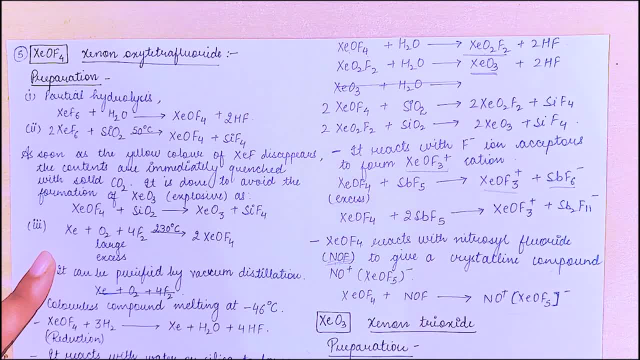 to give crystalline compound n o positive. to give crystalline compound n o positive: XCO f5 negative. so this is the reaction. XCO f5 negative. so this is the reaction. XCO f5 negative. so this is the reaction. the next compound is xenon trioxide. 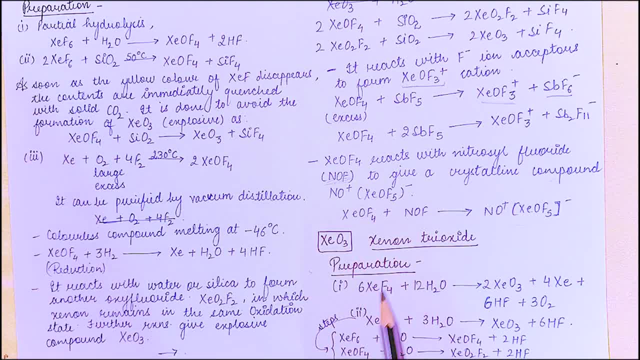 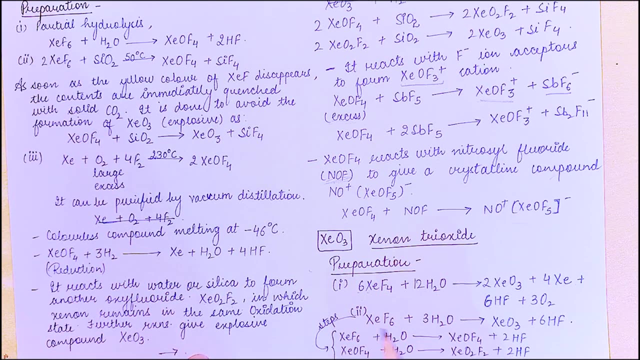 the next compound is xenon trioxide. the next compound is xenon trioxide. let's see the preparation XC f4 on. let's see the preparation XC f4 on addition of water gives xeo3 plus 4, xc, 6, hf and oxygen and xeo6 plus 3. water gives again xeo3. 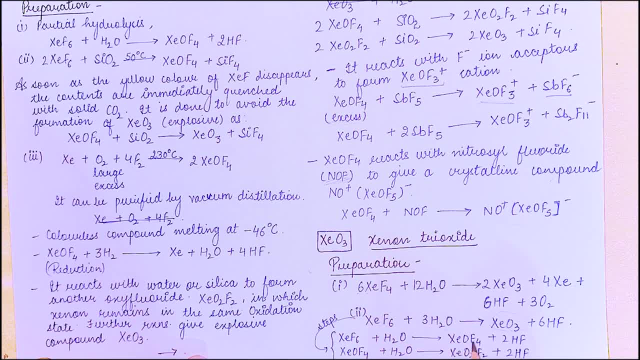 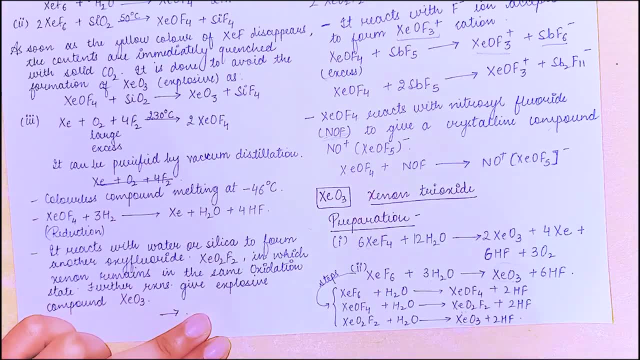 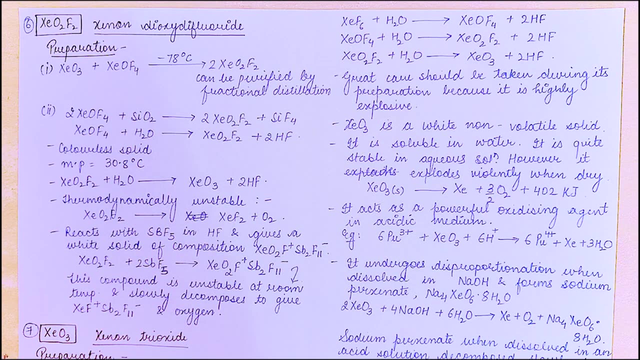 explosive compound. we have already done this reaction: remove 2 fluorine, add 1 oxygen. remove 2 fluorine, add 1 oxygen and finally we get the explosive compound here. so the next compound is xenon dioxydifluoride, xeo2 f2. the preparation is on addition of xeo4 into xeo3. this explosive 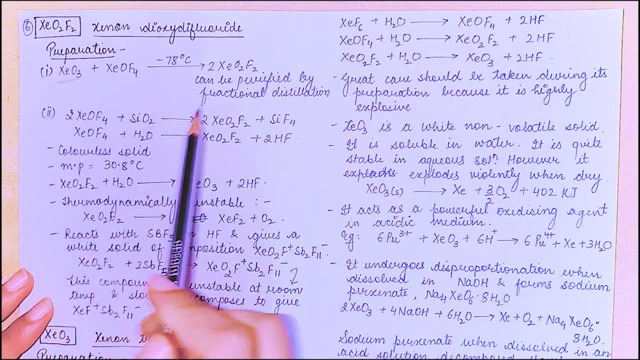 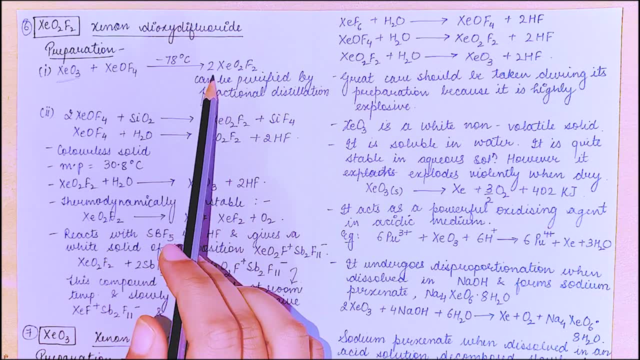 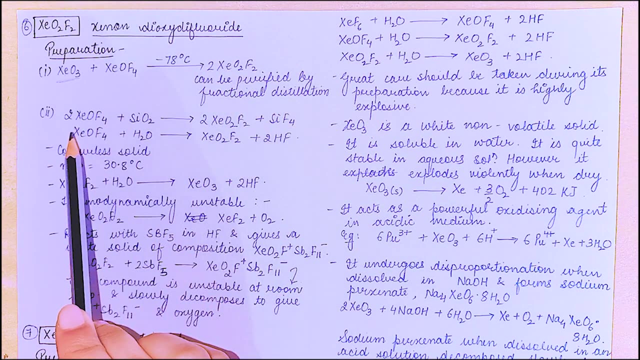 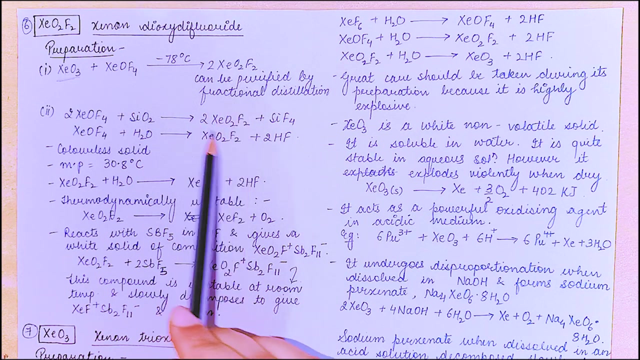 compound. on addition of xeo4 to this explosive compounding, at minus 78 degrees celsius we get this xenon diphloro dioxydifluoride. it can be purified by fractional distillation right now. on reaction with silica it forms again xenon dioxydifluoride. on reaction with water again. 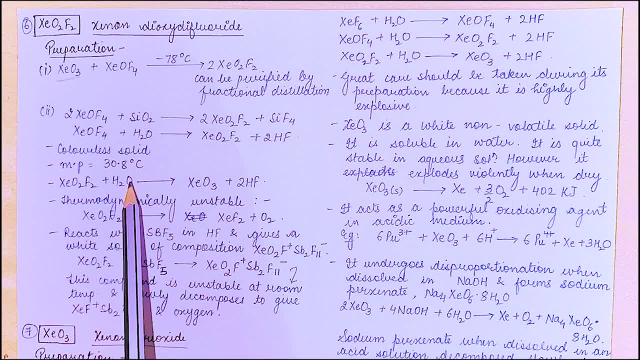 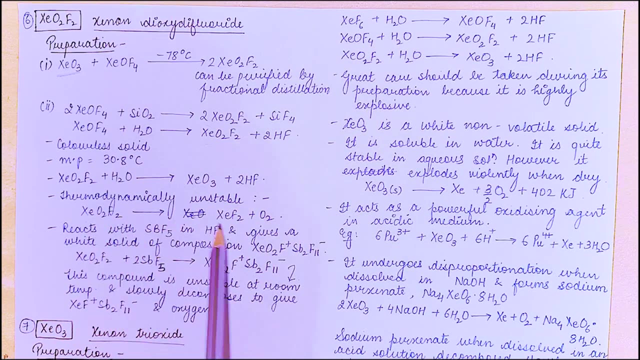 we get the product colorless, solid. all were colorless till now. right, melting point is 30.8 degree celsius on reaction with water it forms that explosive compound plus hf, thermodynamically xeo2 f2. it gives xe f2 plus oxygen. that means it is an unstable compound. it reacts with sb f5 in hf. 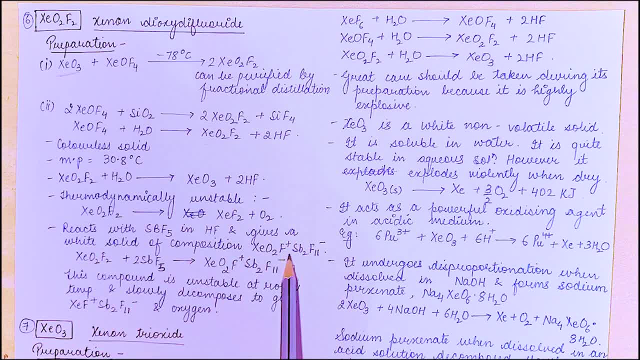 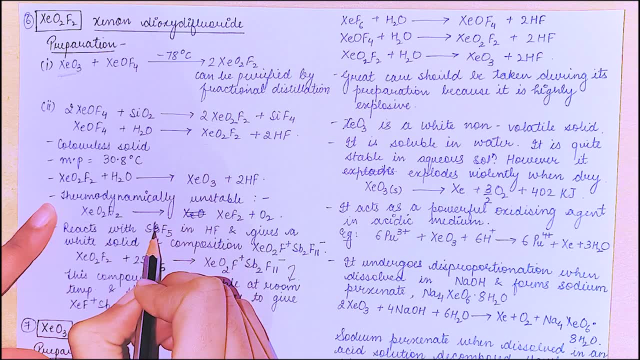 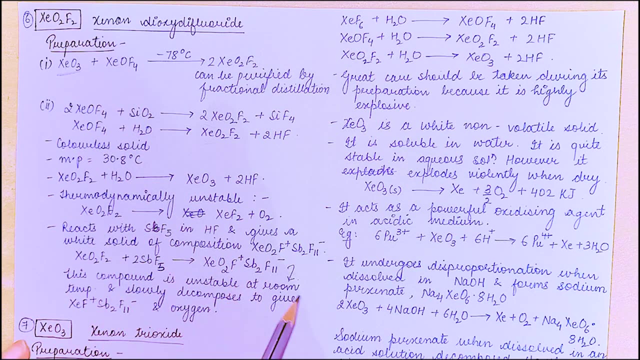 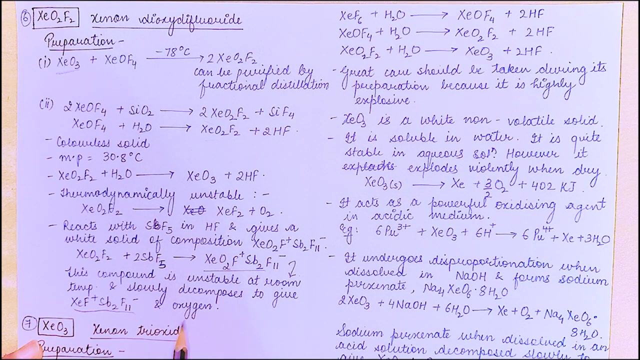 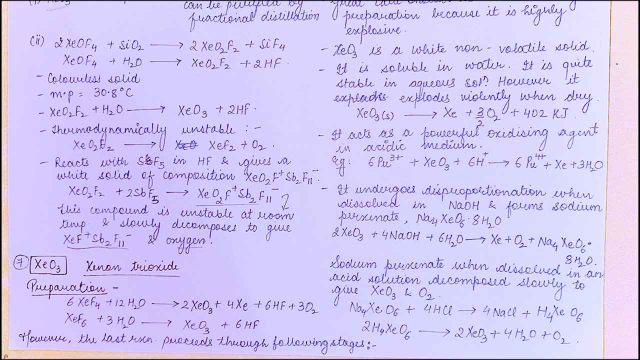 and gives a white solid of composition, xeo2, f positive, sb, f11 negative. it is sb antimony, all right. this compound is unstable at room temperature and slowly decomposes to give xe f positive, sb twice, f11 negative and oxygen. the next compound is xenon trioxide. the preparation: 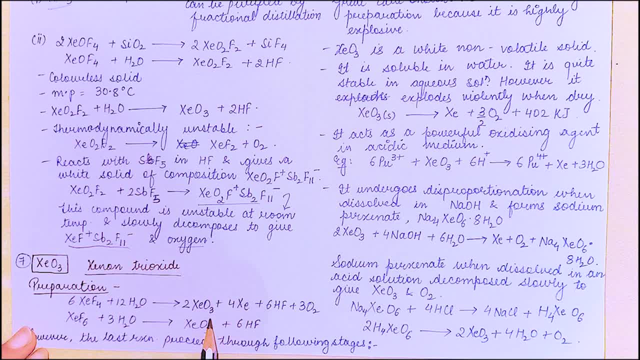 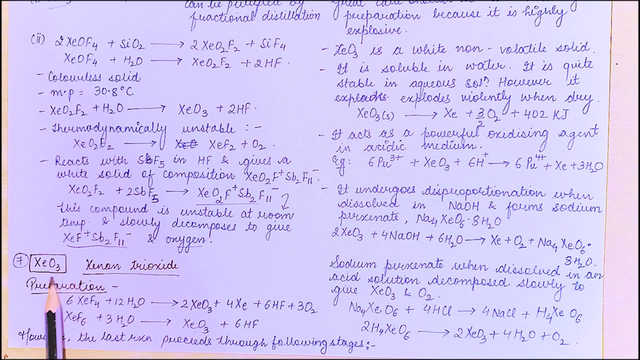 is xe f4 plus water, gives xeo3 plus xenon plus hf plus oxygen. then again, on adding water to xe f6, you get the same product. we are talking about xenon trioxide. this is the same product. we are talking about xenon trioxide. this is the same product. we are talking about xenon trioxide. this is the 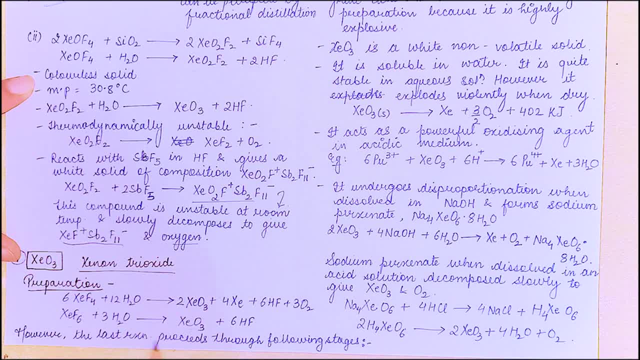 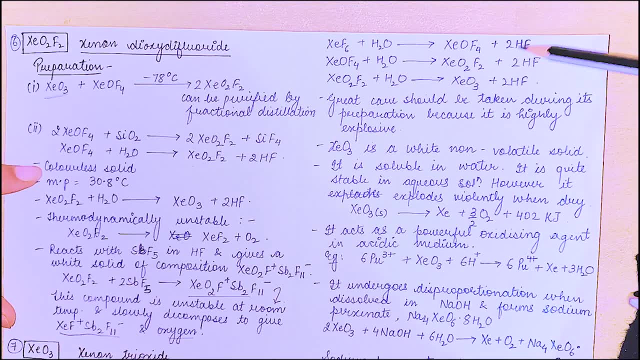 explosive product. however, the last reaction proceeds through the following steps: remove two fluorine, add one oxygen, and so on. great care should be taken during its preparation because it is highly explosive. xeo3 is a white non-volatile solid, so this is white in color and it is. 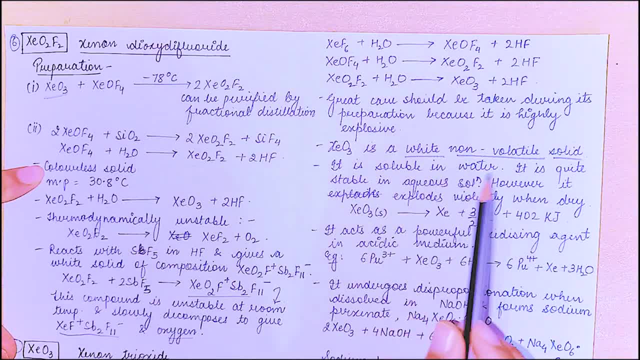 non-volatile. it is solid, it is soluble in water. it is quite stable in air. it is quite stable in water, but it will go to effervescence. it is extremely strong at ready status, and so it will graduallyWelcome you to this simple reaction experiment. right here we are going to talk. 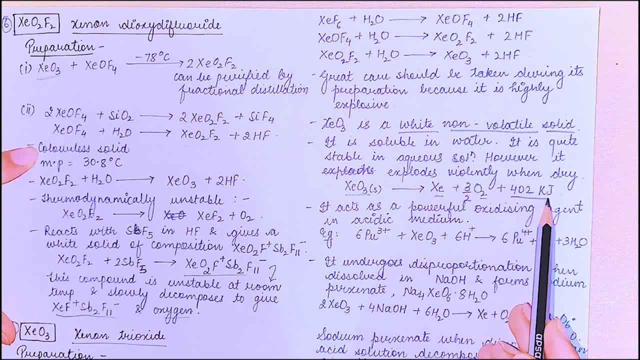 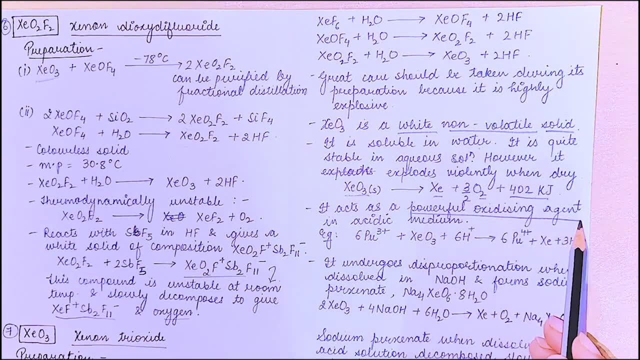 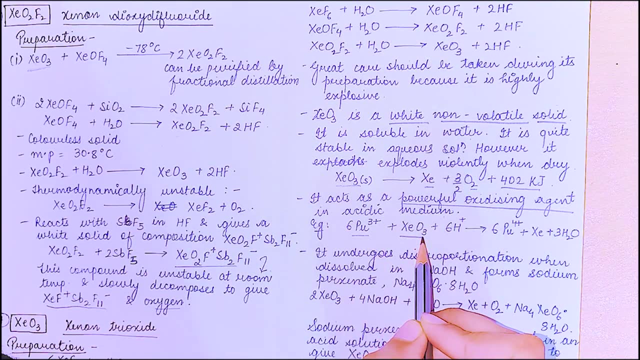 about carbon dioxide and how we are going to get cups of hydrogen out of the lake. so what is carbon dioxide and how? the most about this one is carbon dioxide comes in quedes. of course you can talk about that in bigger details, but let me be brief about what it. 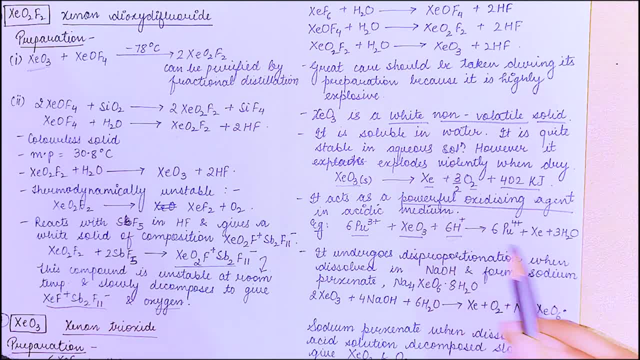 is, and let me show you what is exactly. carboxy Creatinine hydrogen is a hydrogen that釀 メ is for life. release aiotêu lack-beats Bear, but 줄 xeo2ω. in the presence of hydrogen, that iki hydrogen you get fu当然, lets say ionic. 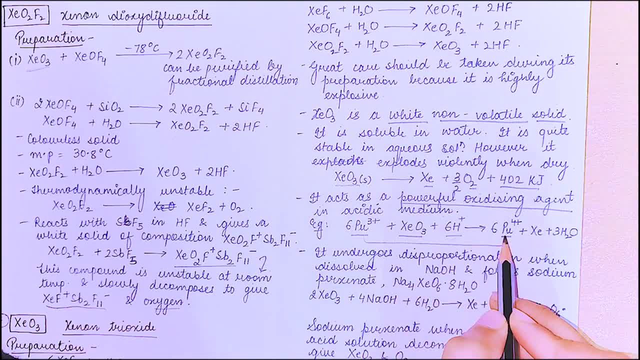 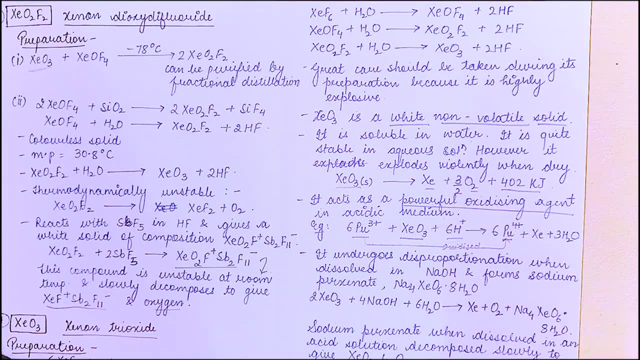 esting the reaction it creates. when xeo3ichtet slid through hydrogen and it is because oxygen- bad four positive- it is being oxidized, right, oxy diced. so what is the oxidizing agent that is being reduced? that is getting reduced here? xenon is going from plastic. 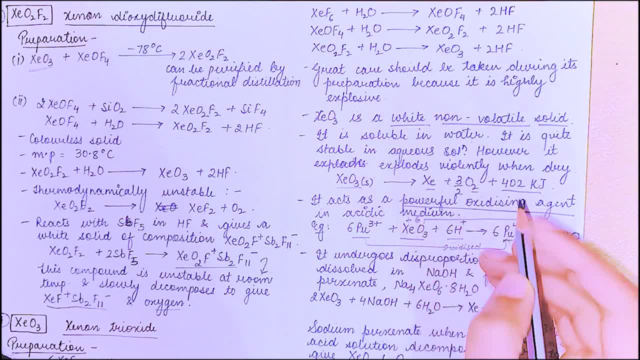 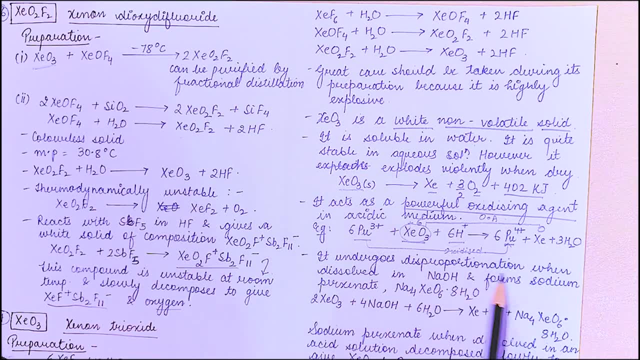 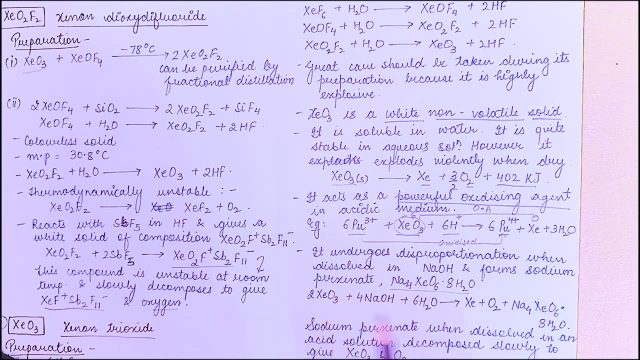 state to zero. that means it is getting reduced. so this is an oxidizing agent. so XCO 3 is an oxidizing agent. it undergoes this proportionation when dissolved in NaOH and forms sodium parzenate. this is the compound right, sodium parzenate. when 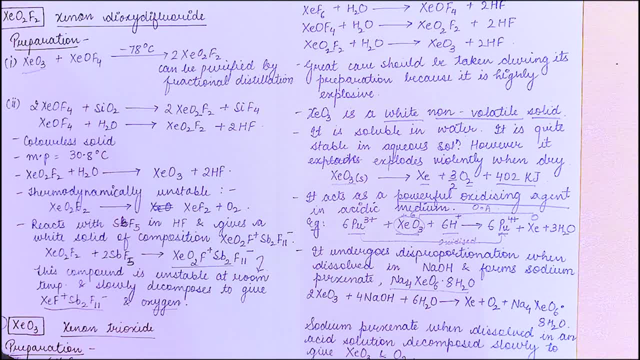 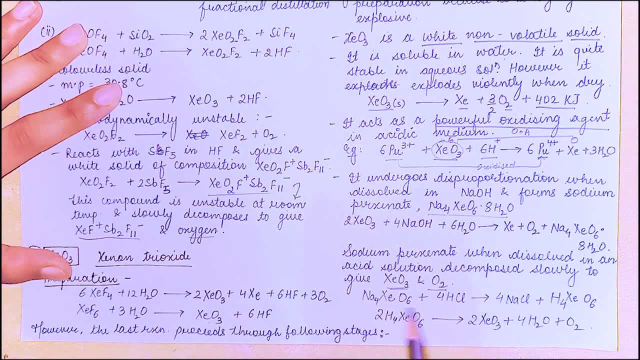 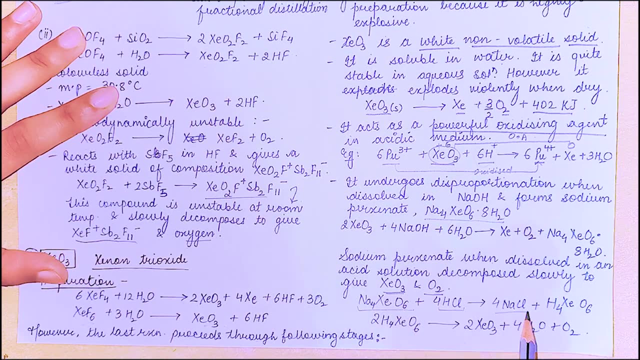 dissolved in an acidic solution decompose slowly to give XCO 3 and O2, as you can see here. so Na4- XCO 6 on addition of HCl gives NaCl plus H4- XCO 6. now this furthers the oxidizing agent and this is the oxidizing agent that is. 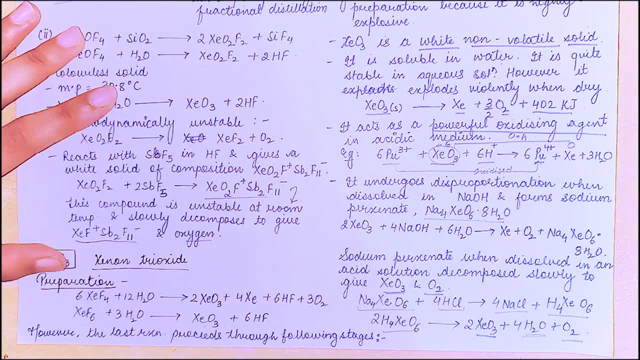 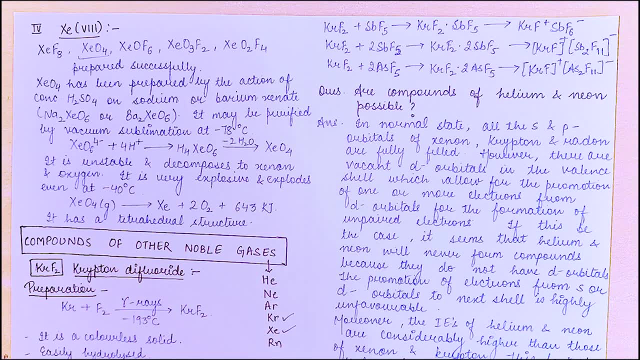 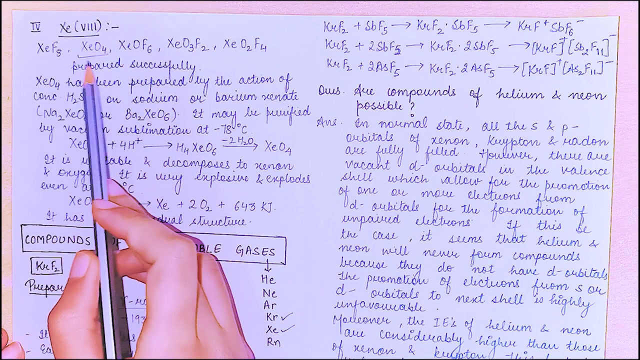 giving XCO 3, plus water, plus oxygen. so next we have xenon in plus state oxidation state. there are compounds like XCF 8, XCO 4, XCO F6, XCO 3, F2, XCO 2, F4. these can be prepared. this compound, XCF 4, it is successfully prepared, it has 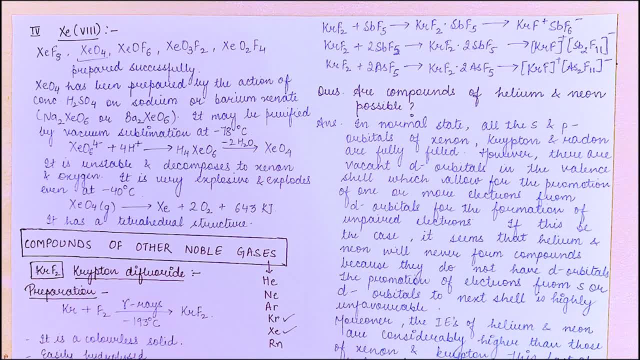 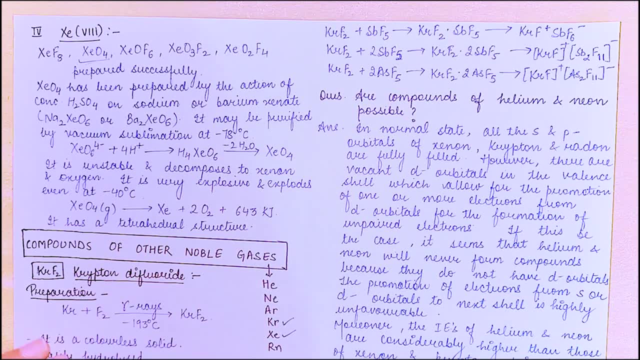 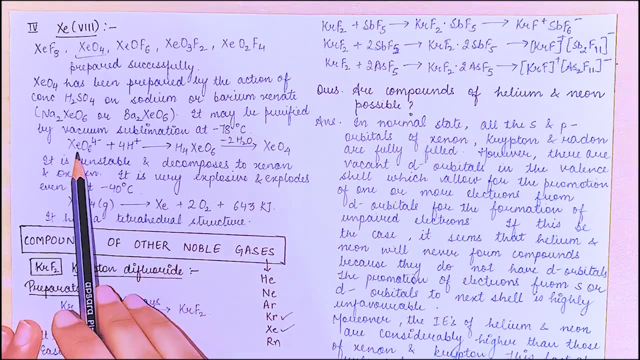 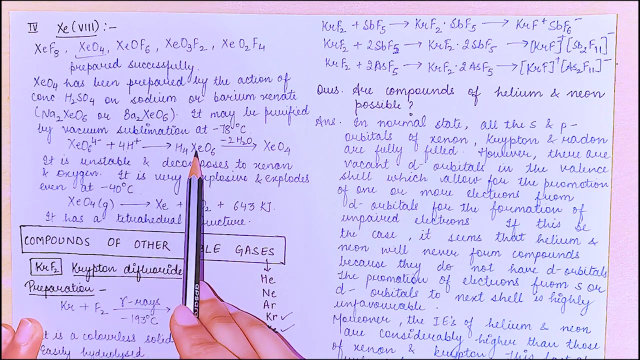 been prepared by the action of concentrated sulfuric acid on sodium or barium xenate. this is sodium xenate and this is barium xenate. it may be purified by vacuum sublimation at minus 78 degrees Celsius. now this XC O6 4 negative in acidic medium. it gives H4, XC O6 and gives XC O4 when water is removed. when water is removed. 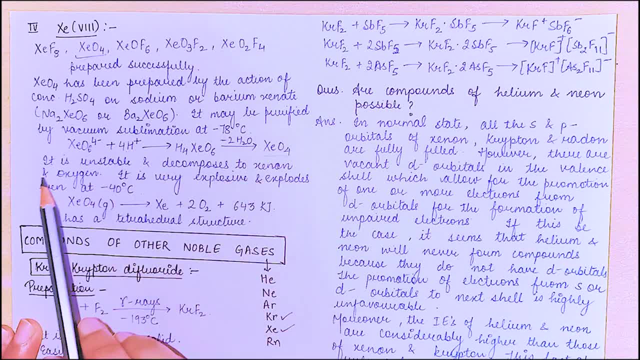 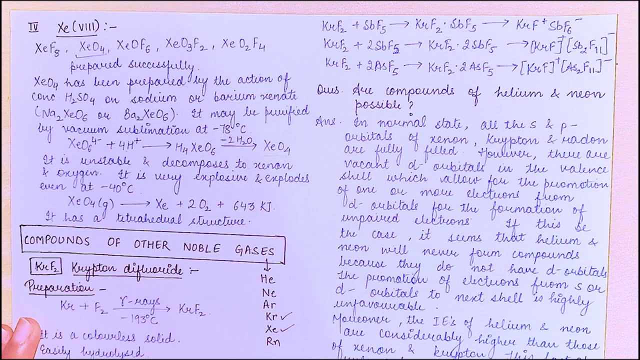 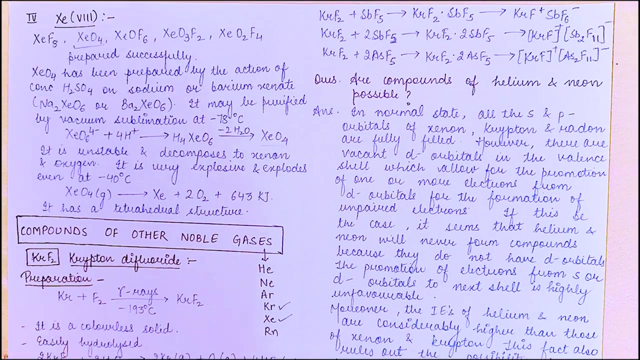 right. it is unstable and it decomposes to Xenon and oxygen. it is very explosive and explodes even at minus 40 degrees Celsius. so it is: it explodes even at such a cool temperature. it has a tetrahedral structure. we will discuss the structures later. now let's see the compounds of other noble gases. here we have cryptic. 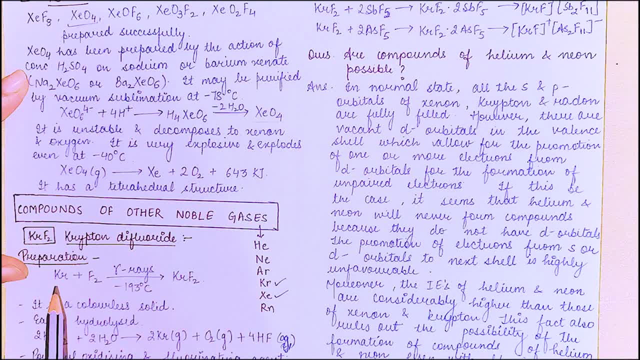 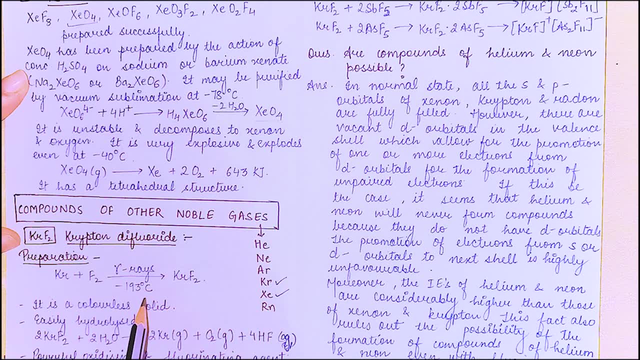 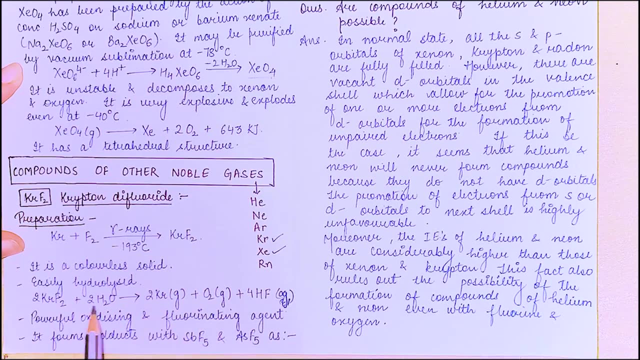 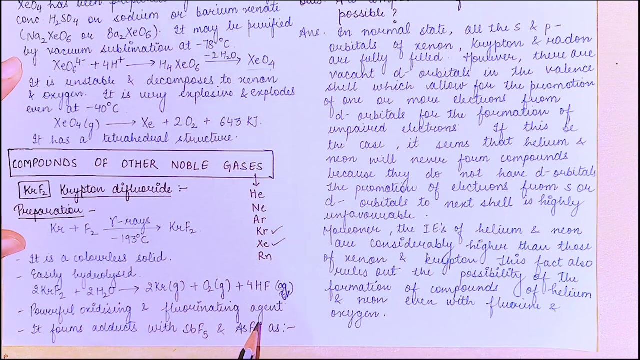 di fluoride. right preparation: krypton on addition of fluorine, in the presence of gamma rays at minus 193 degrees Celsius, gives krypton di fluoride. it is a colorless solid, easily hydrolyzed on addition of water. gives krypton oxygen and HF. it is a powerful oxidizing agent and fluorinating agent. oxidizing. 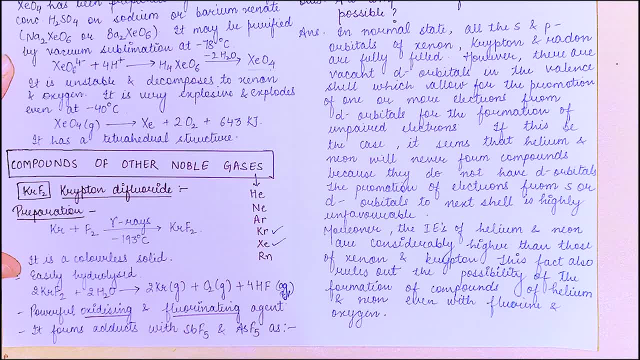 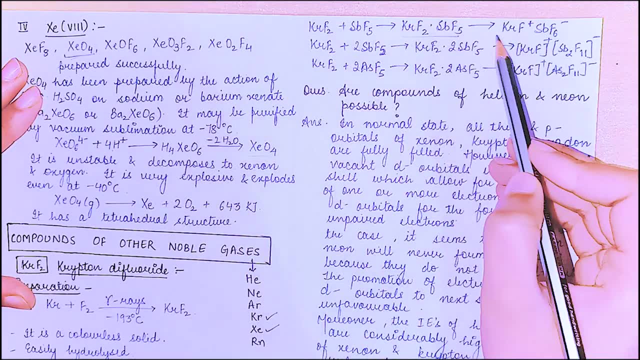 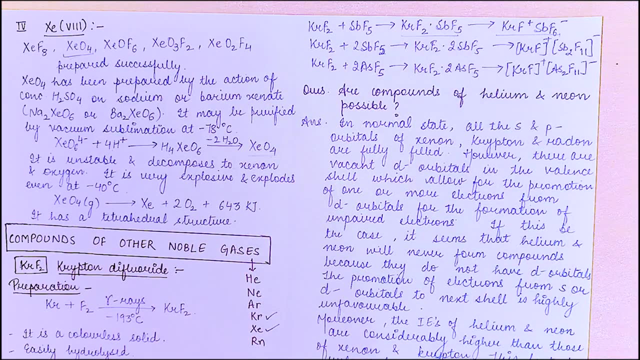 fluorinating. it forms adducts with SBF 5, ASF 5, as the other compounds were doing so, right from the ducts and you can write it as ionic form also. so there is a question for you: are the compounds of helium and neon possible? so let's see. 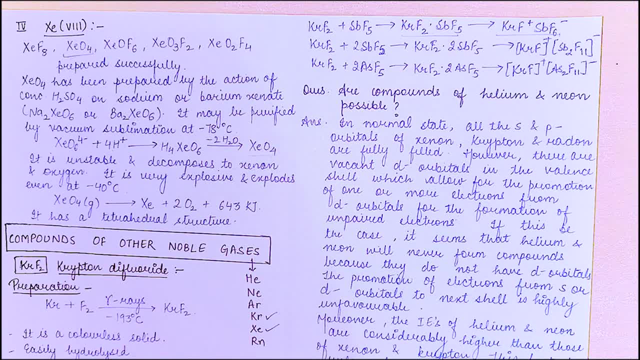 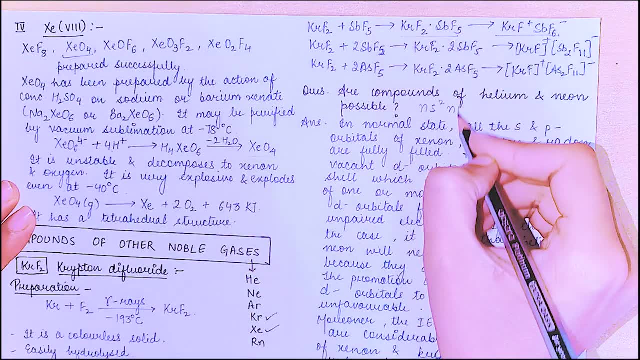 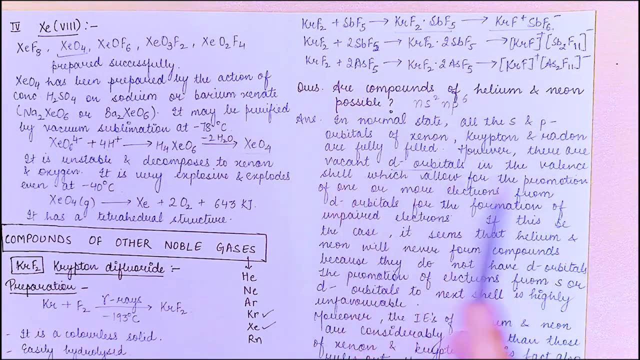 the answer. in normal state, all the s and p orbitals of xenon, krypton and radon are fully filled. we know the electronic configuration is ns2, np6. however, there are vacant d orbitals in the valence shell which allow for the promotion of one or more electrons from. 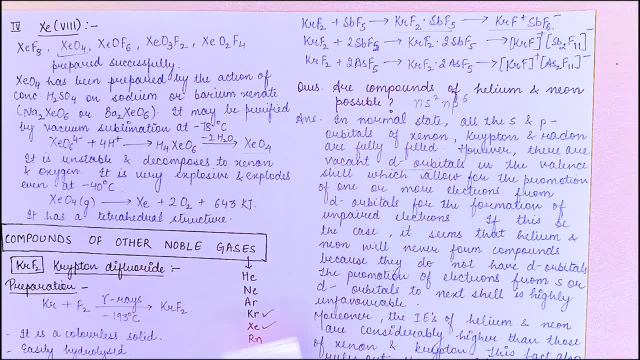 d orbitals for the formation of unplayed electrons, so the vacant d orbitals may accept electrons. if this be the case, it seems that helium and neon will never form compounds because they do not have d orbitals. so the motion of electrons from s or d orbitals to next shell is highly unfavorable right. 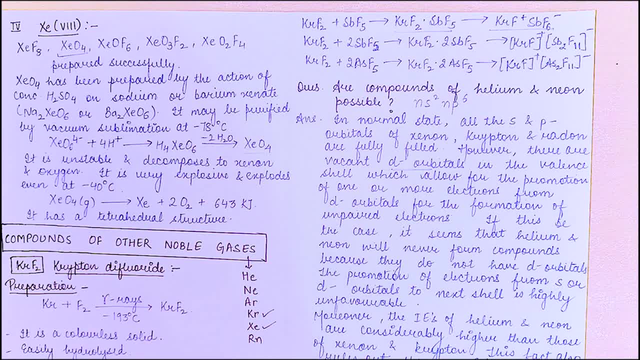 moreover, the ionization energies of helium and neon are considerably higher than those of xenon and krypton. this fact also rules out that possibility of formation of compounds of helium and neon even with fluorine and oxygen. we'll be doing more such types of experiments in the future, so stay tuned for more information. 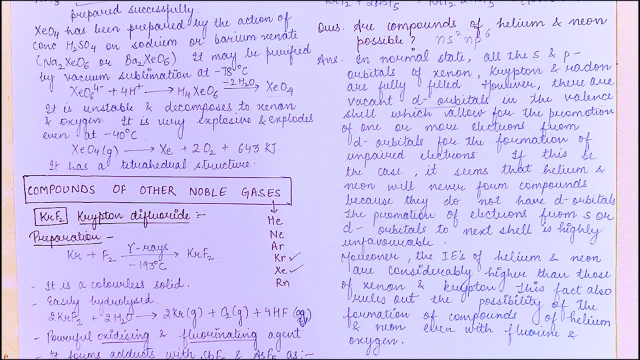 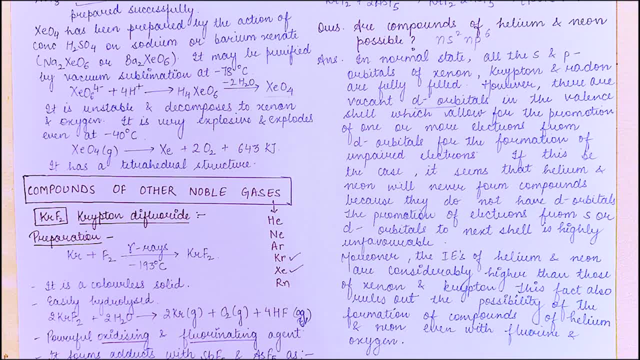 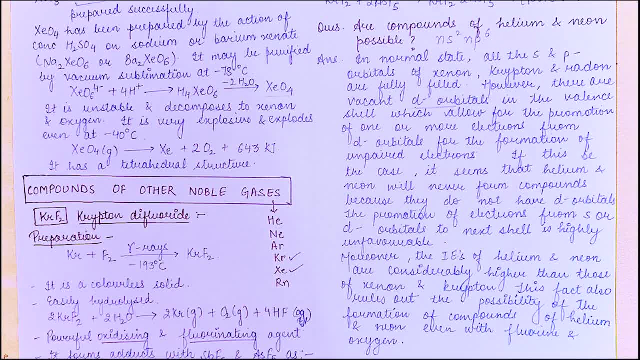 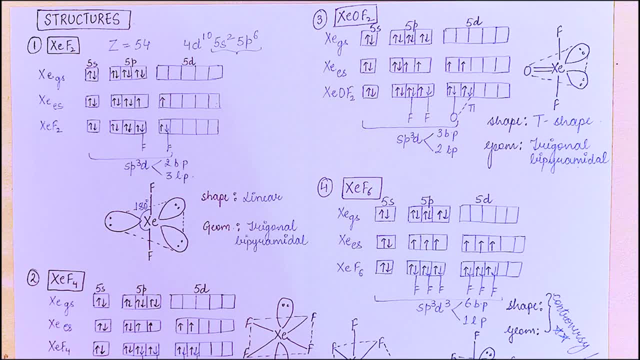 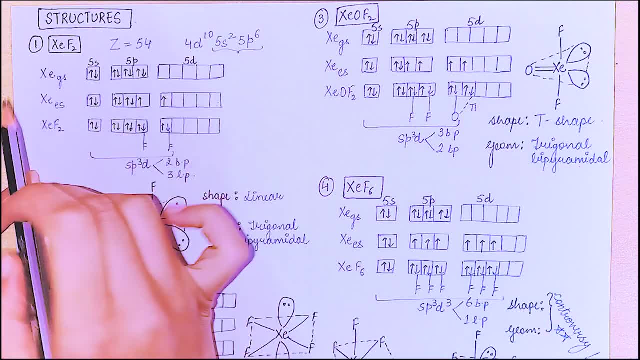 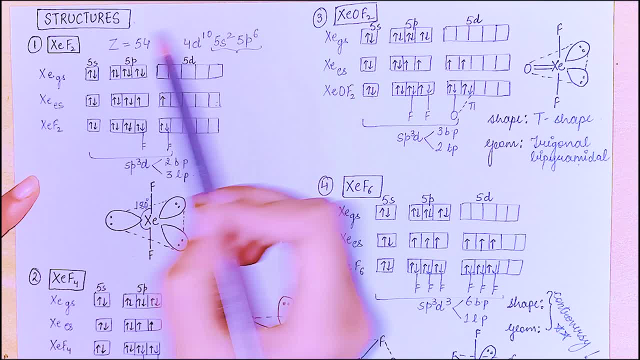 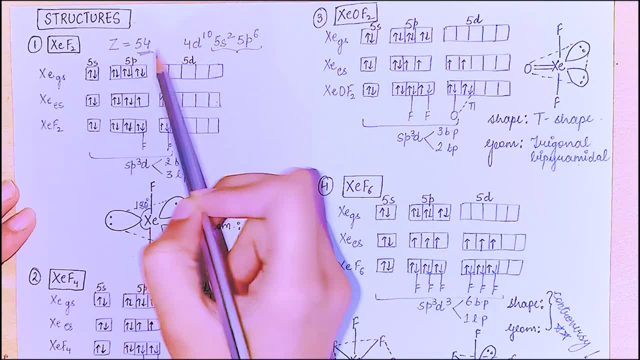 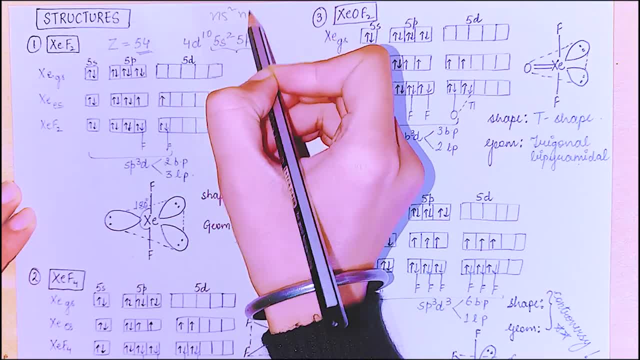 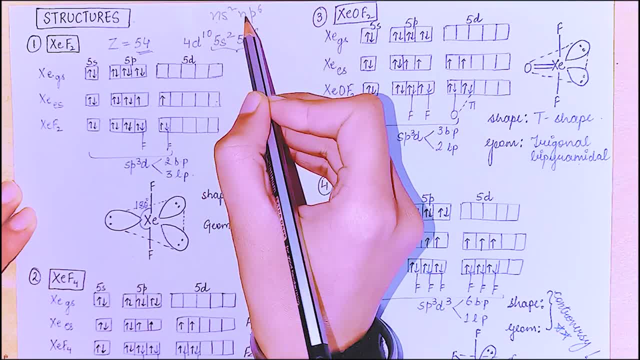 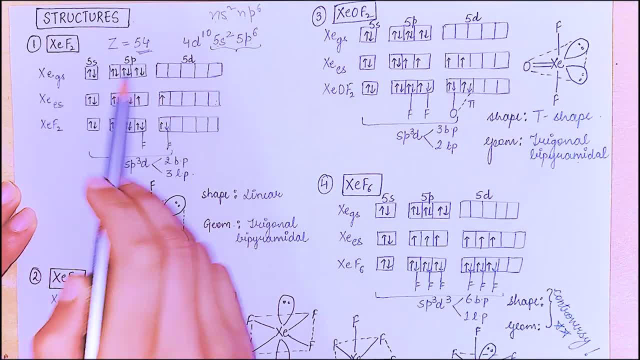 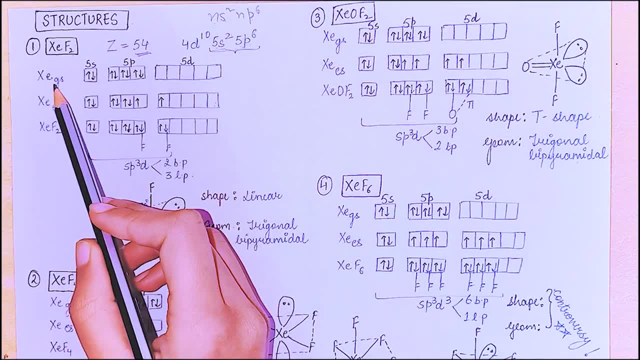 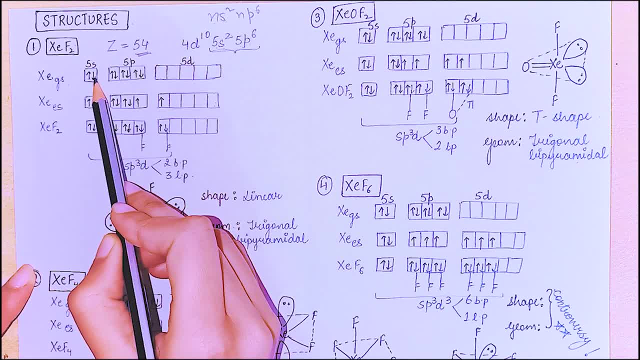 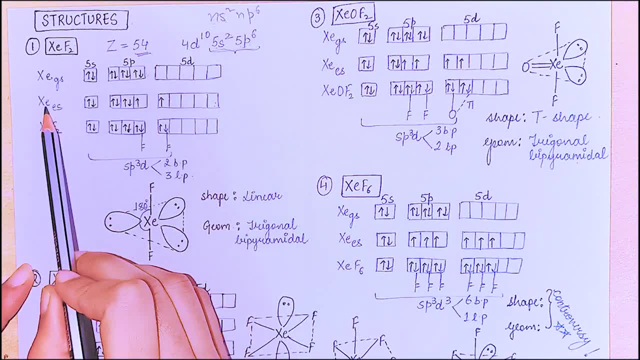 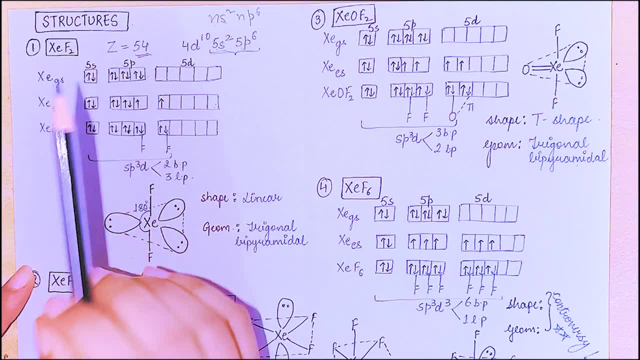 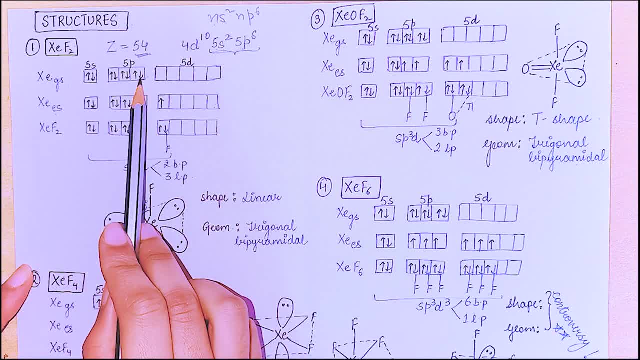 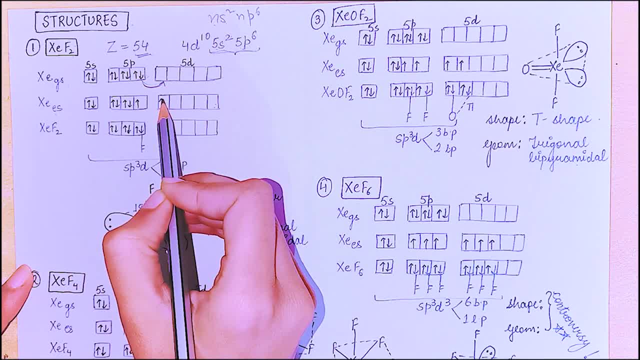 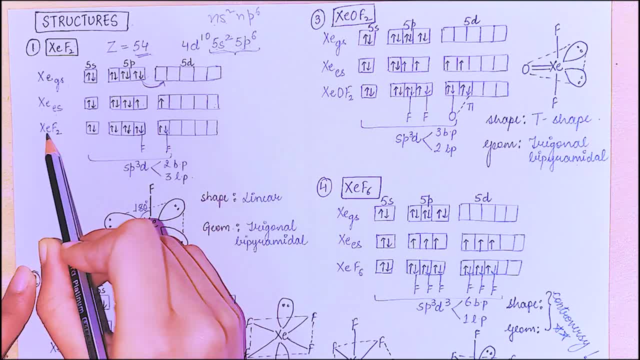 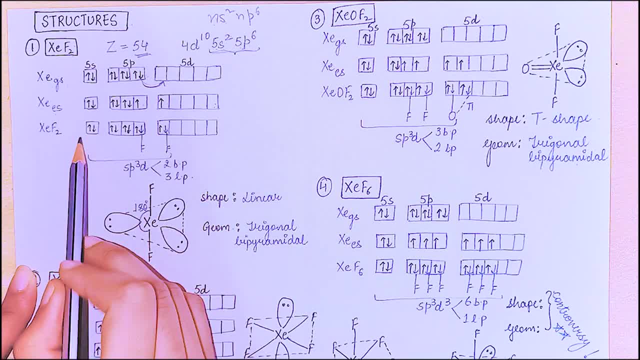 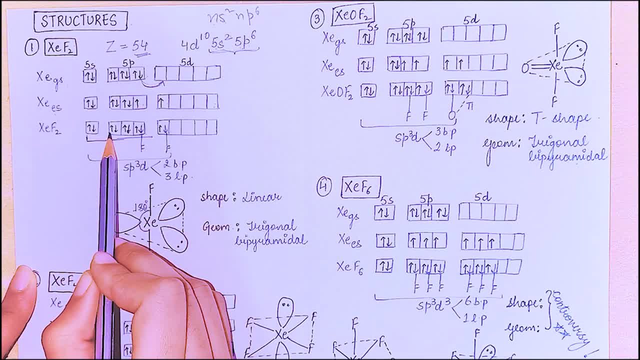 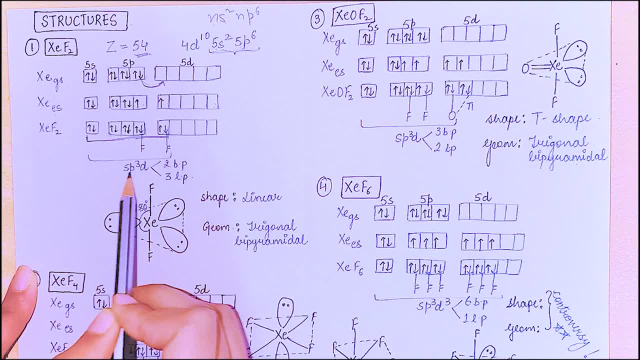 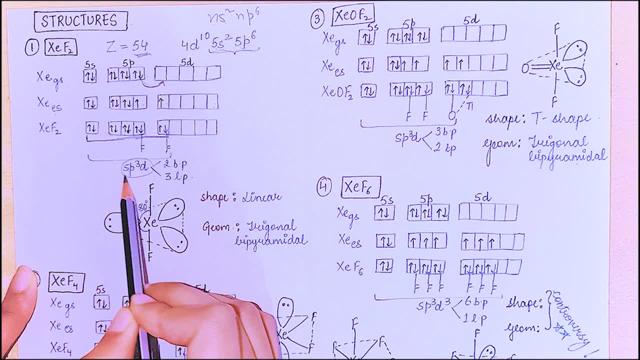 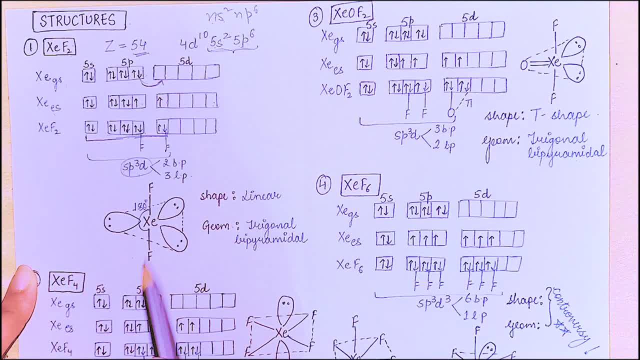 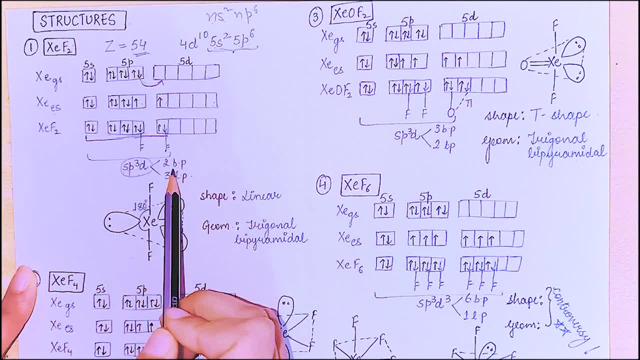 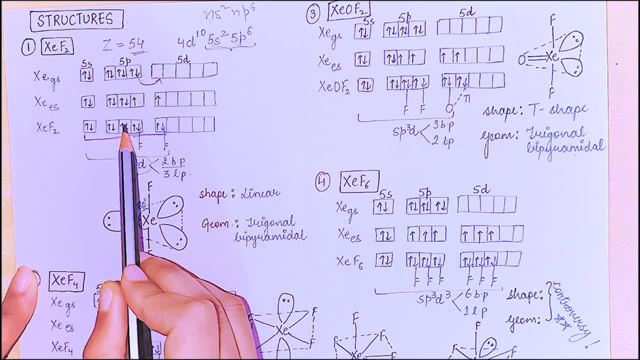 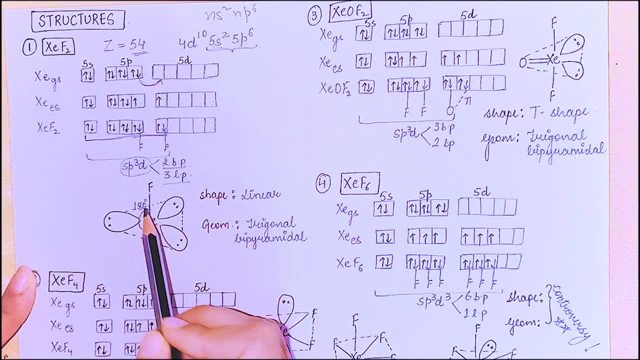 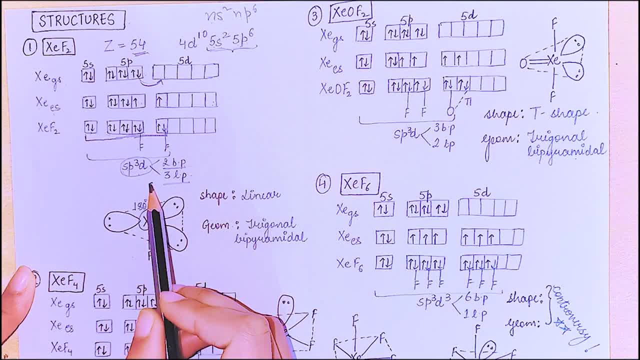 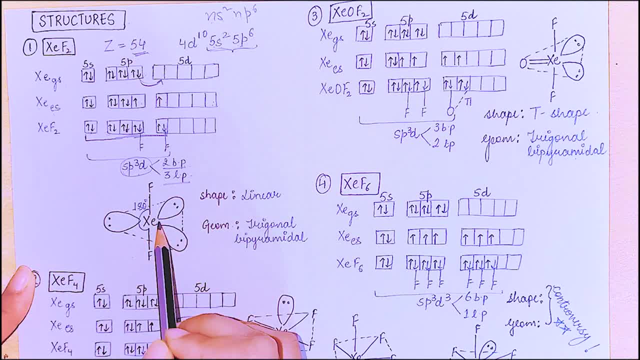 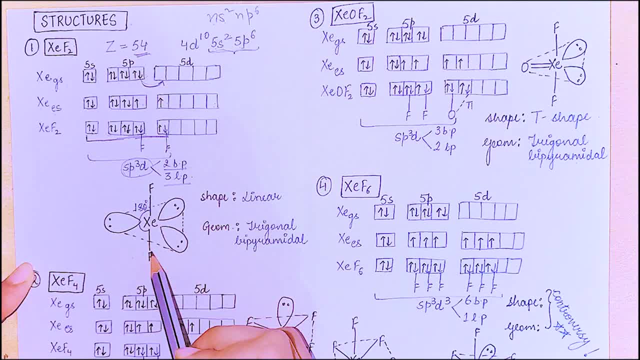 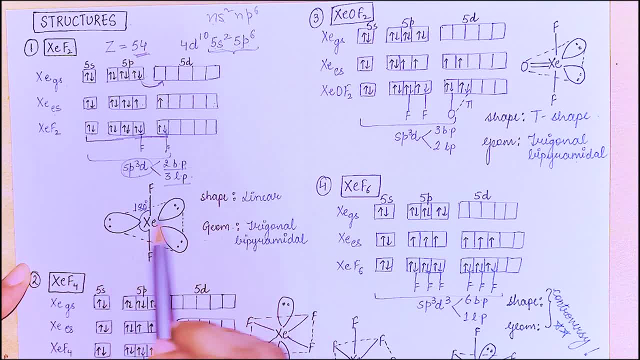 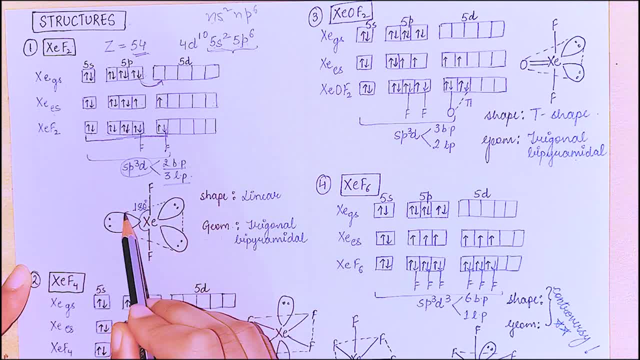 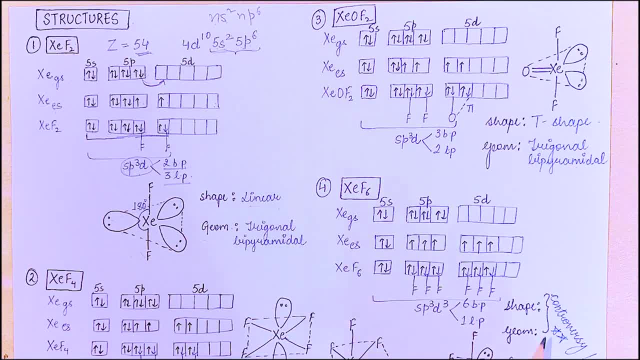 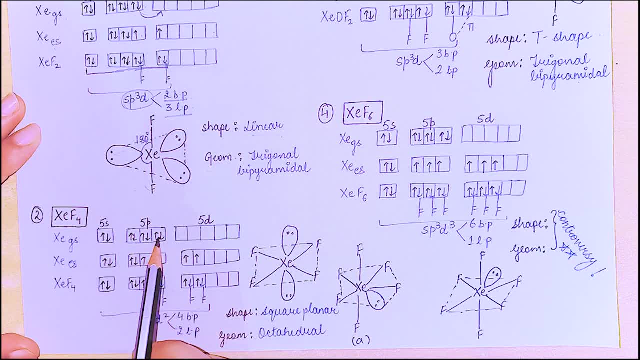 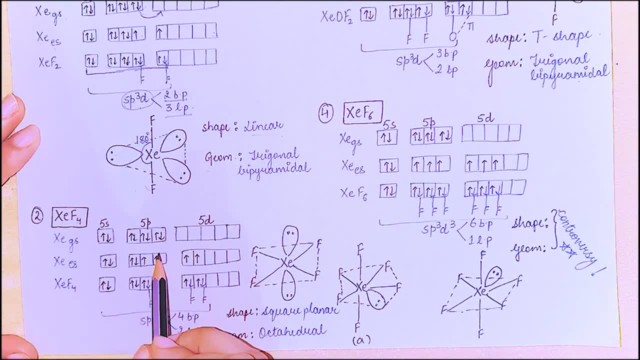 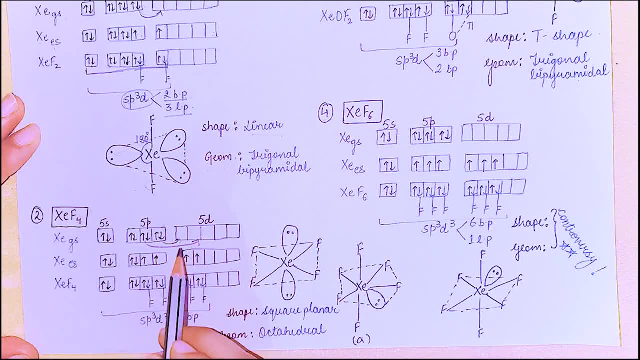 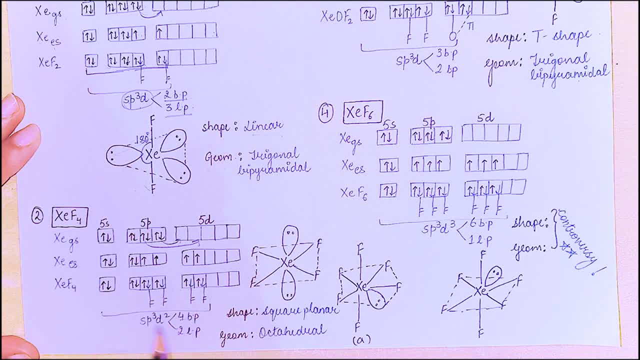 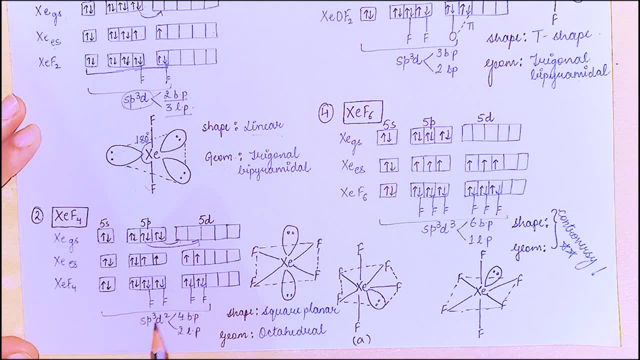 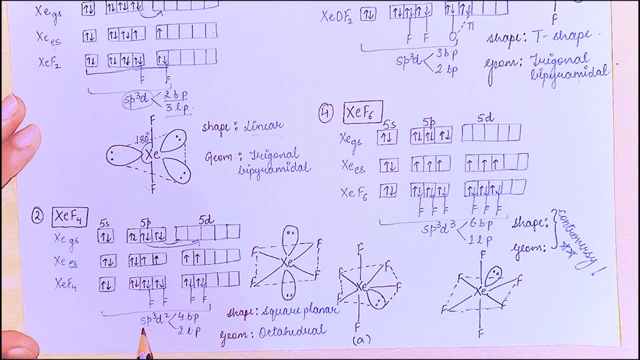 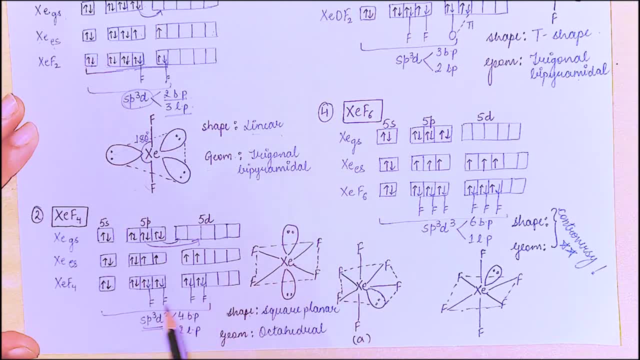 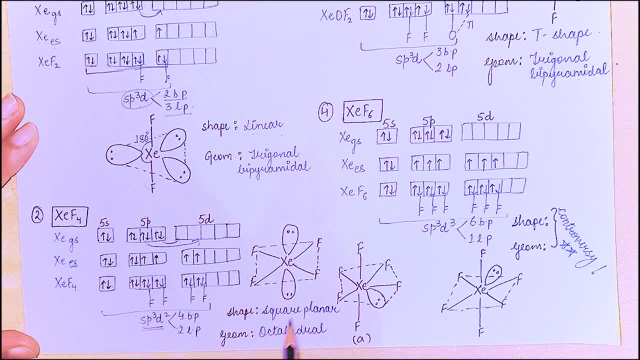 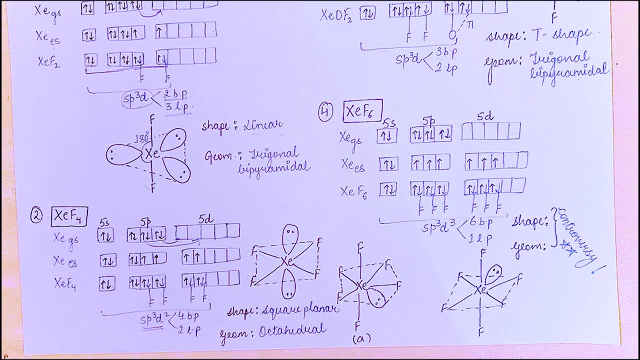 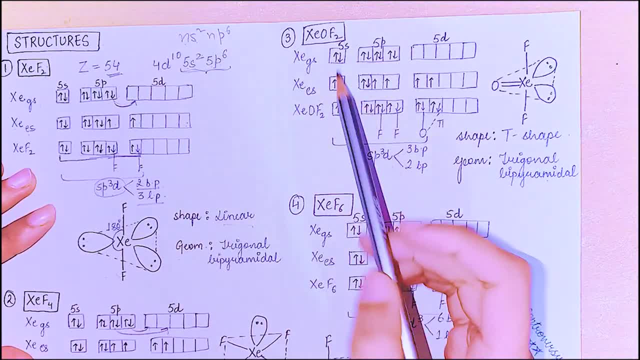 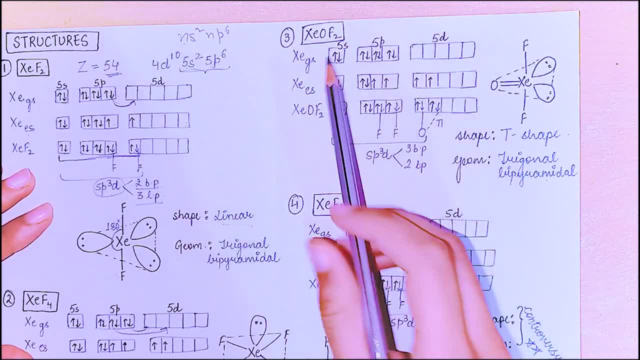 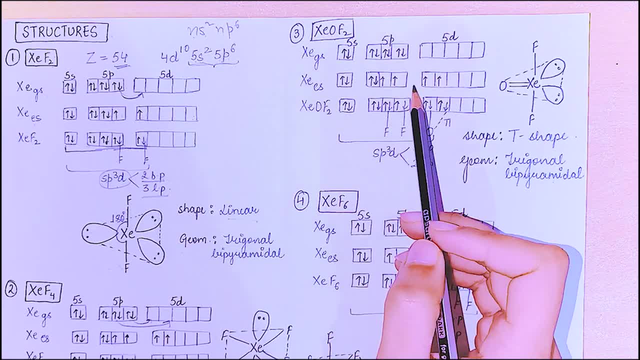 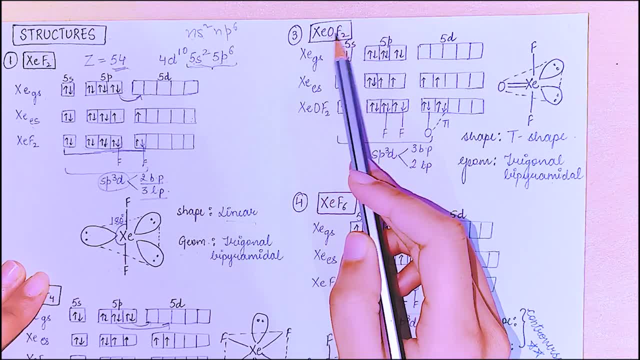 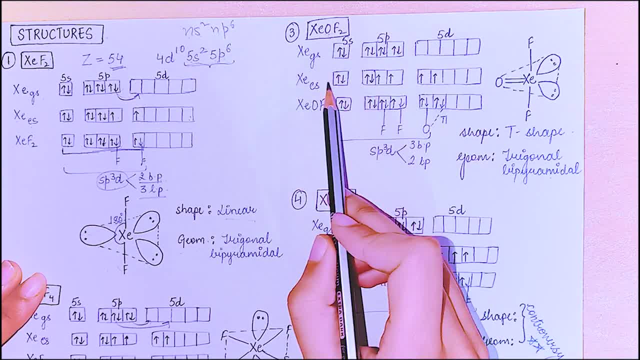 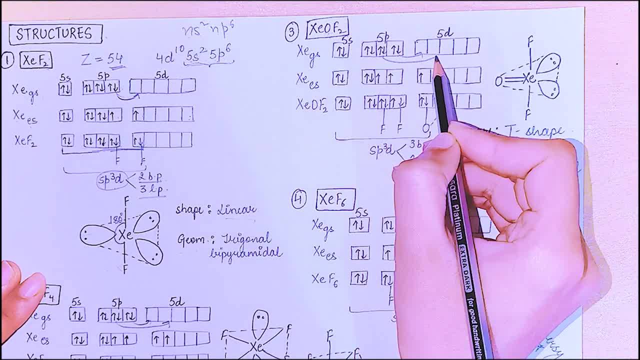 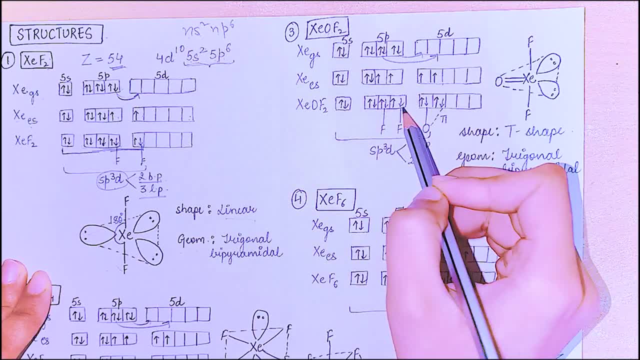 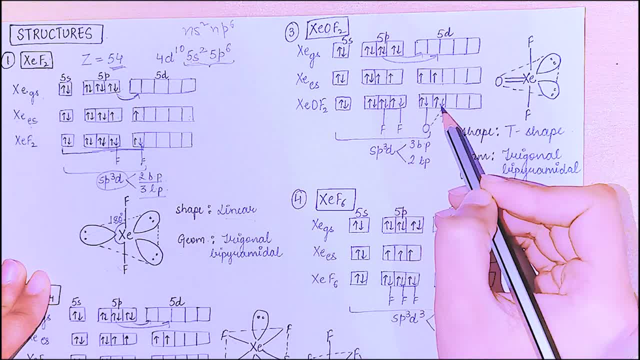 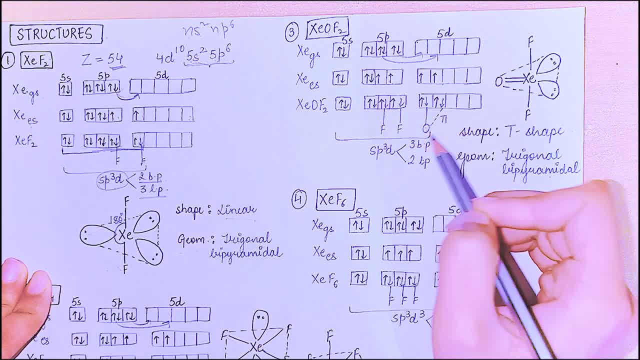 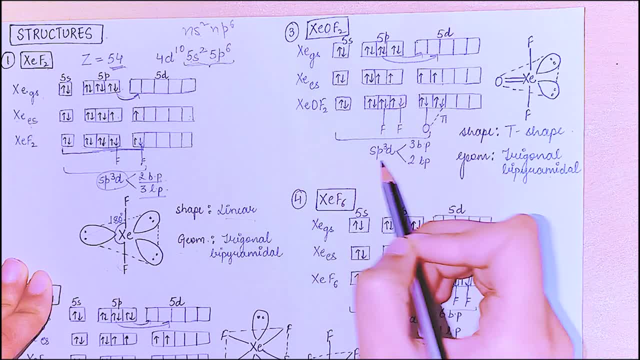 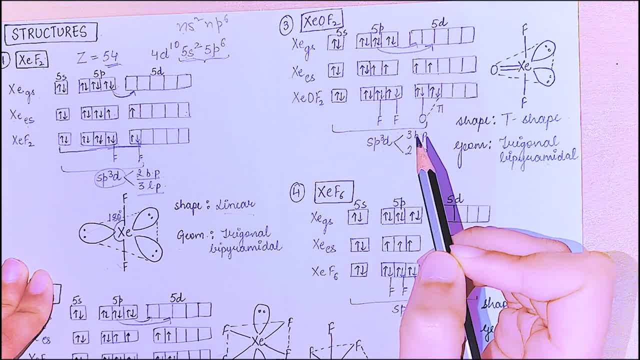 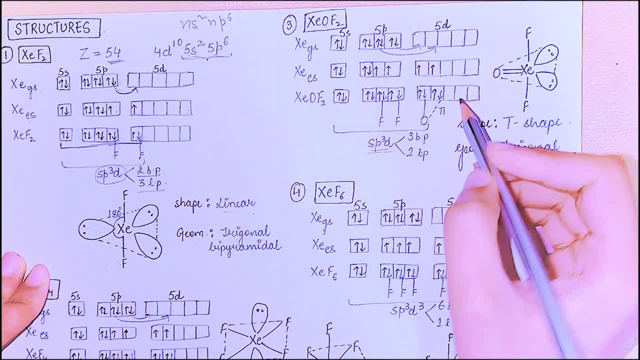 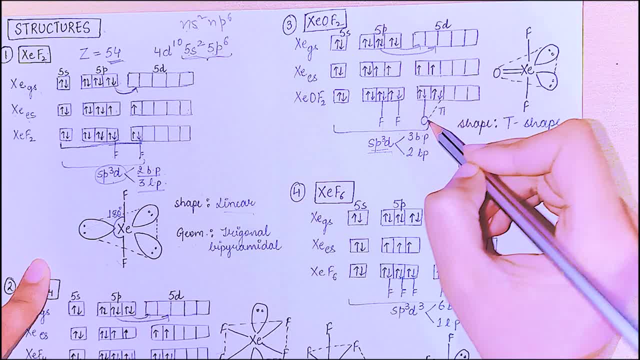 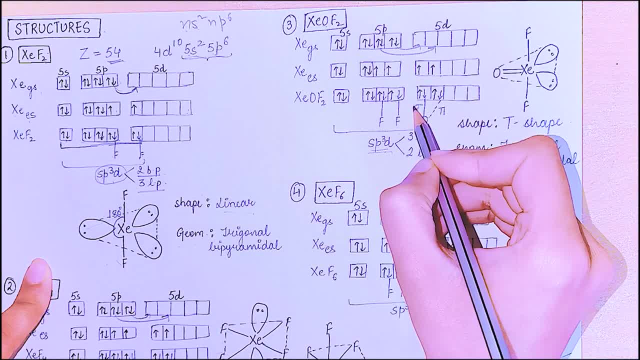 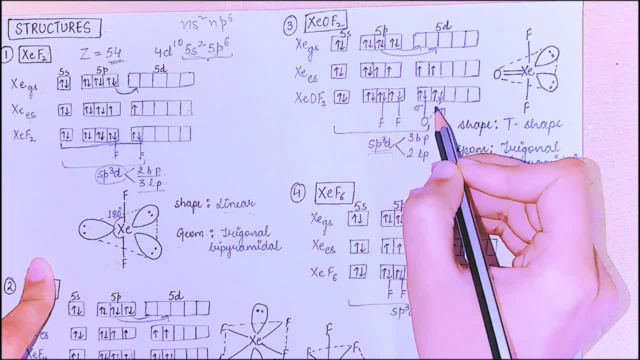 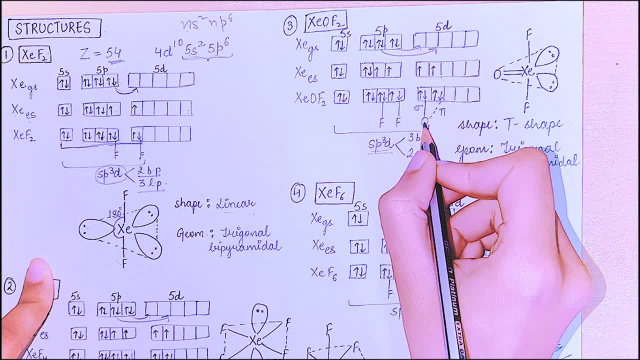 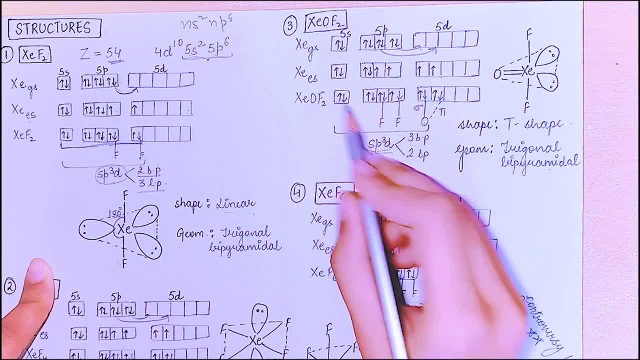 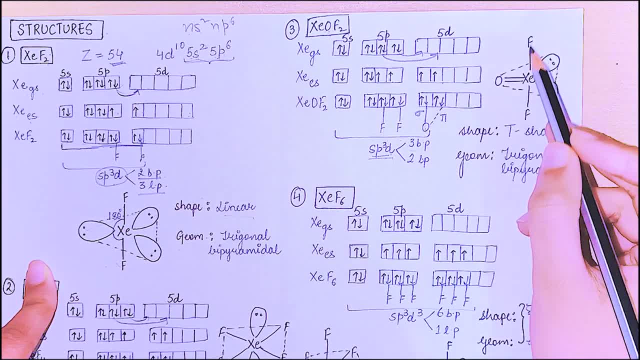 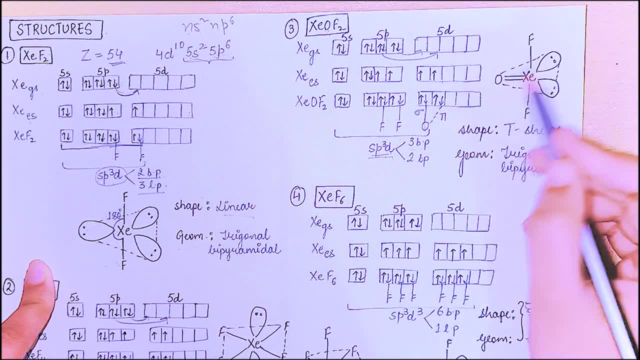 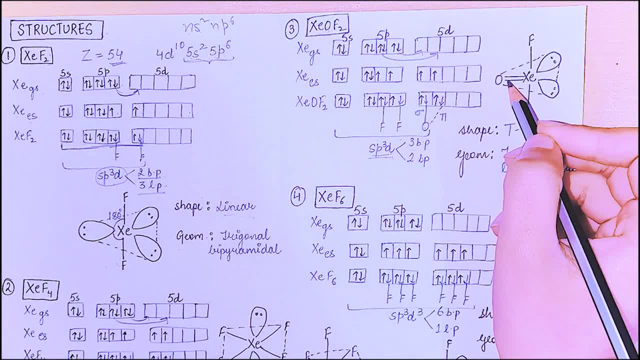 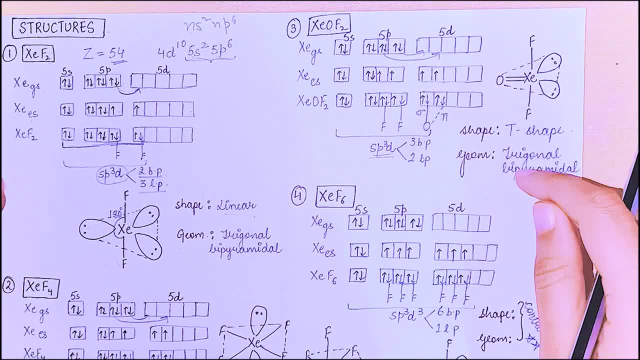 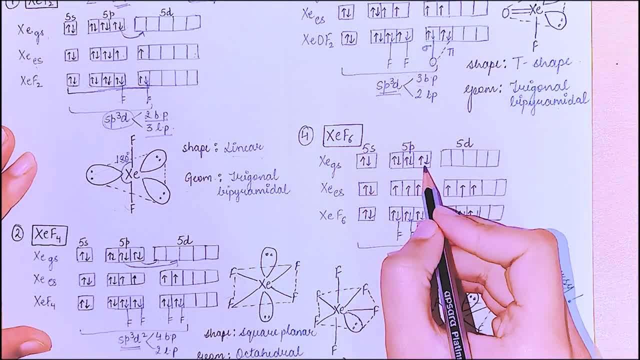 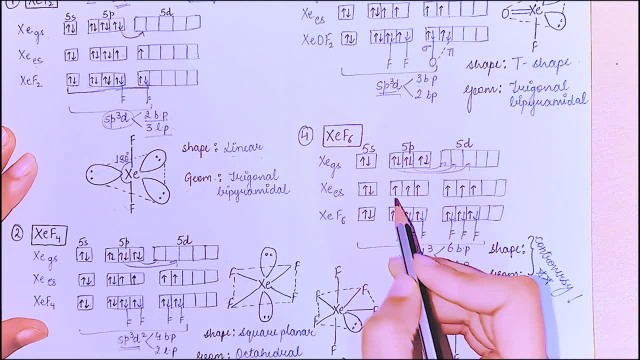 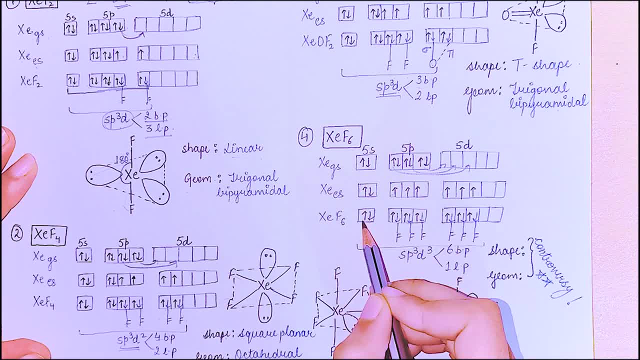 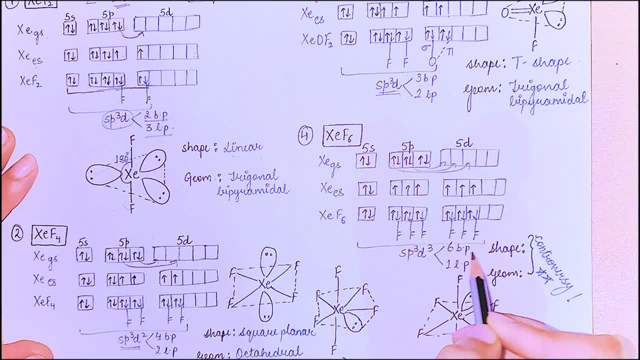 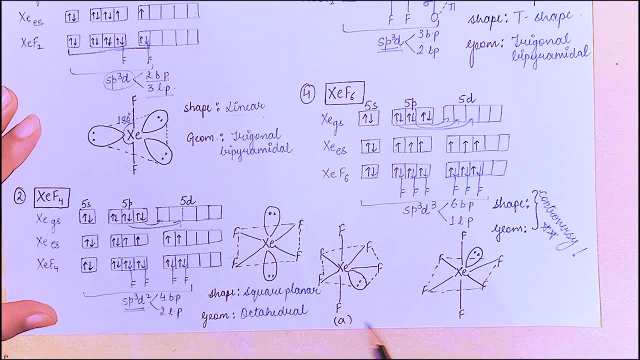 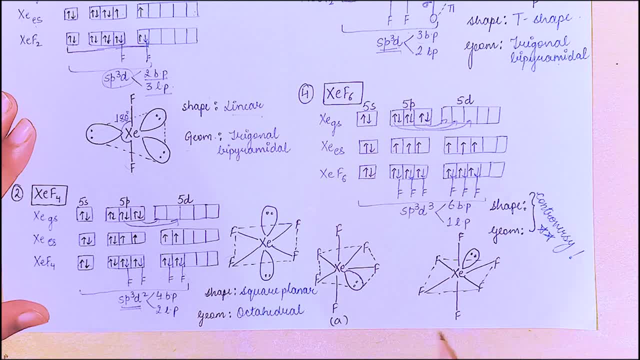 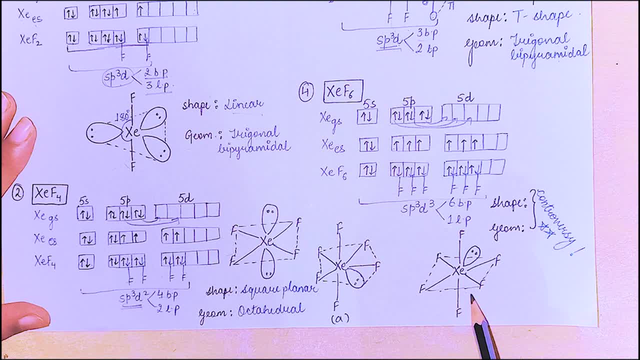 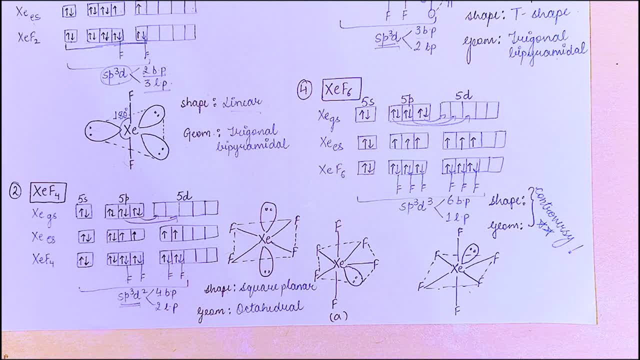 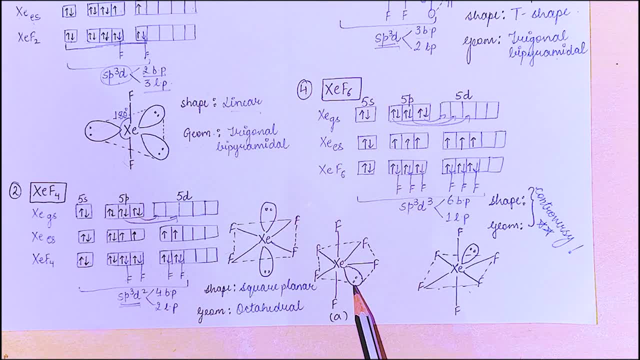 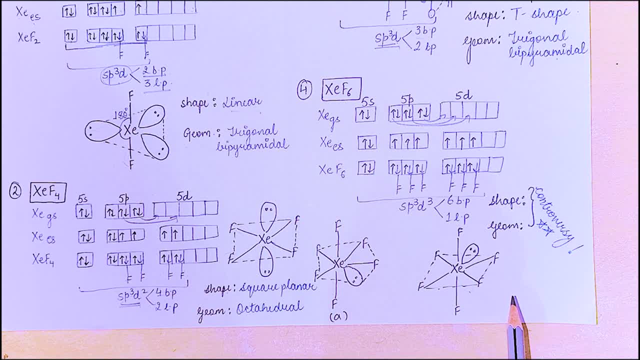 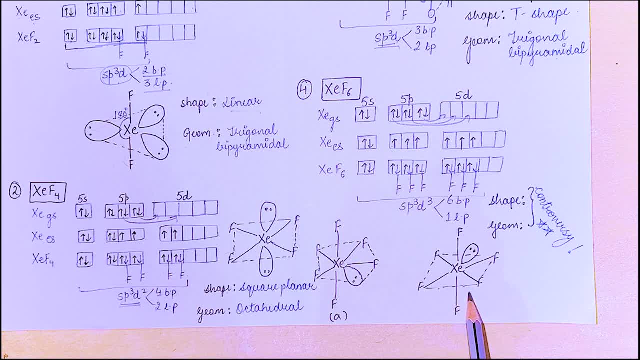 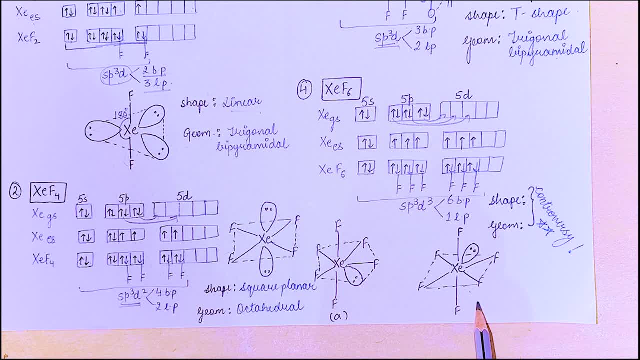 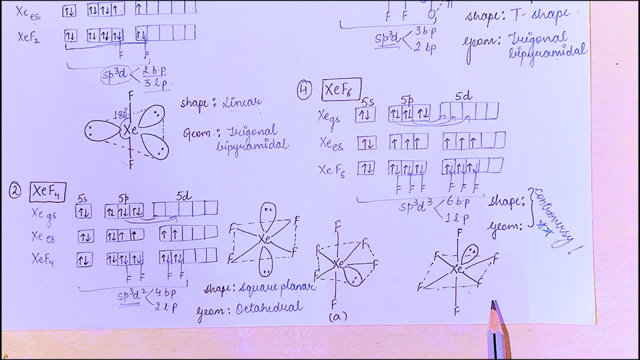 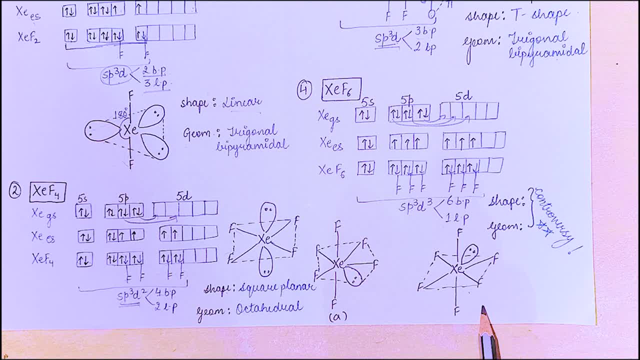 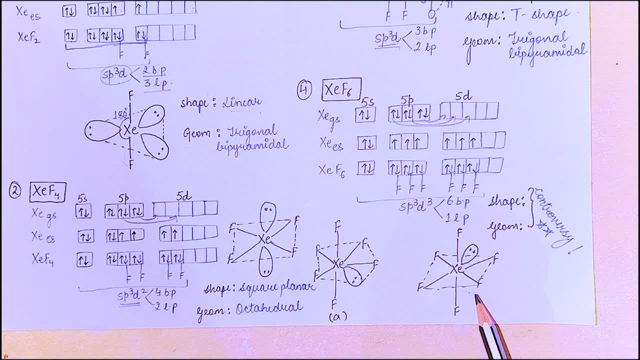 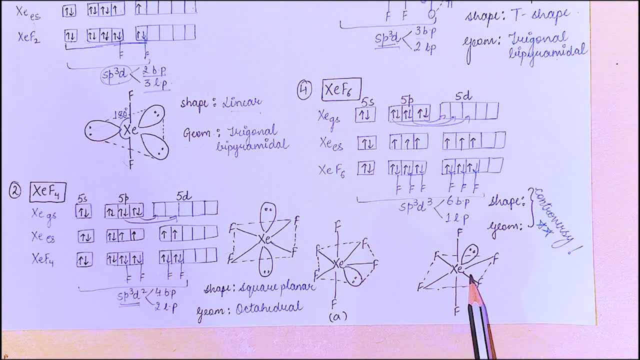 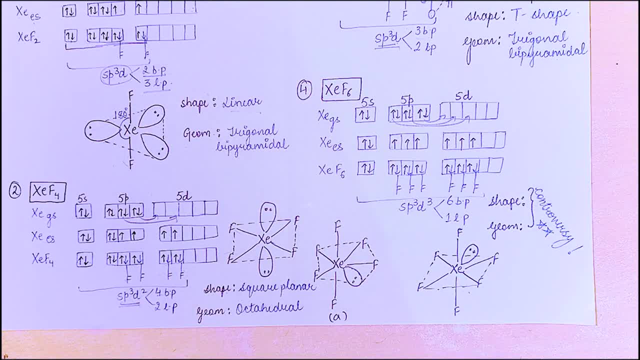 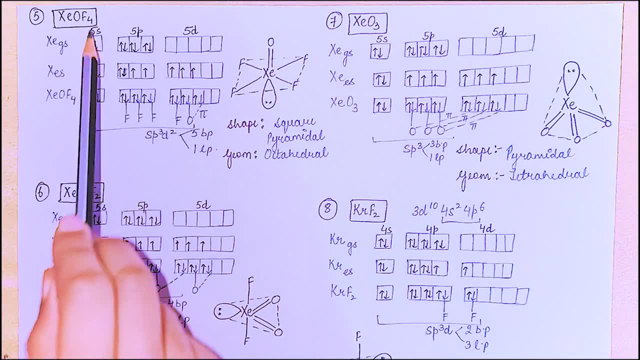 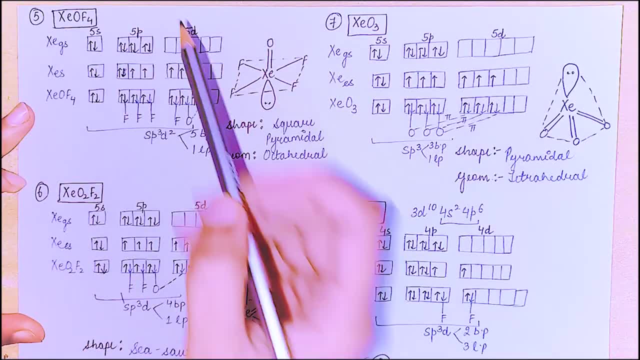 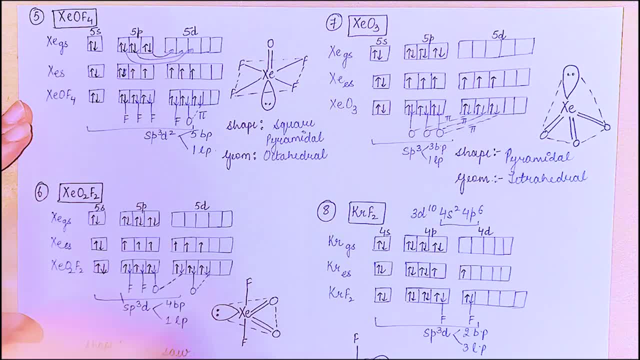 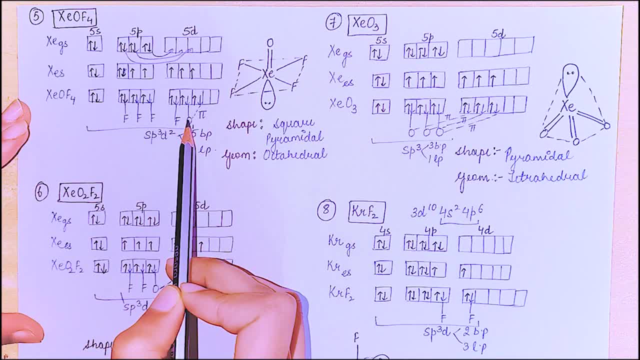 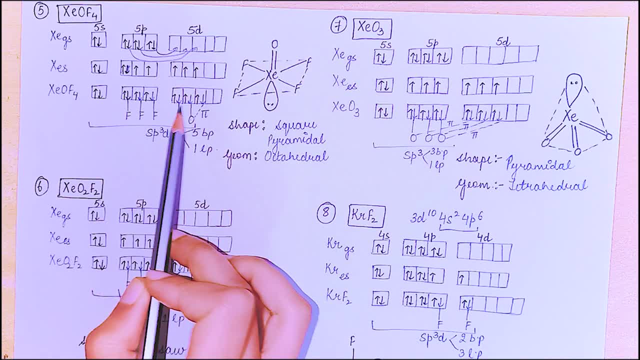 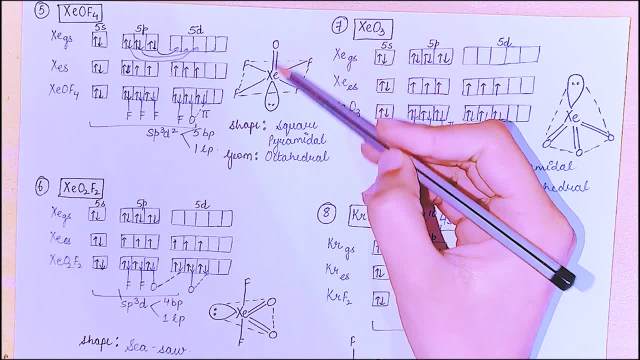 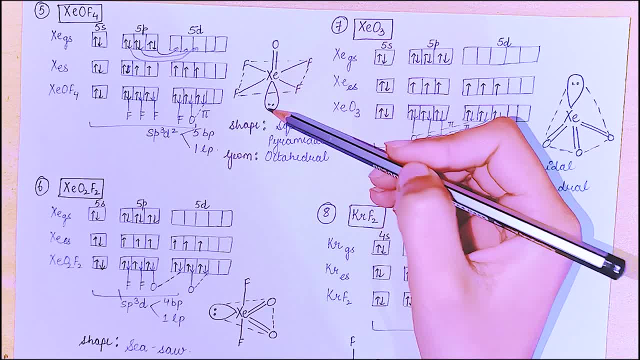 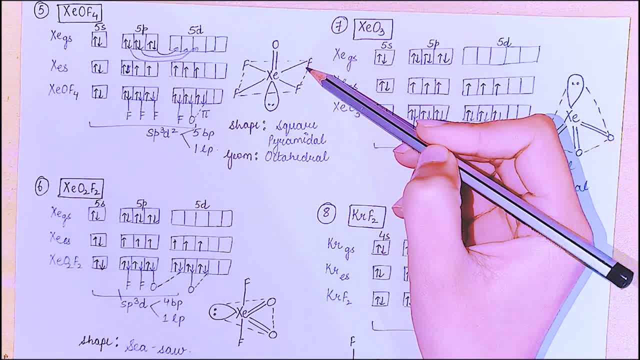 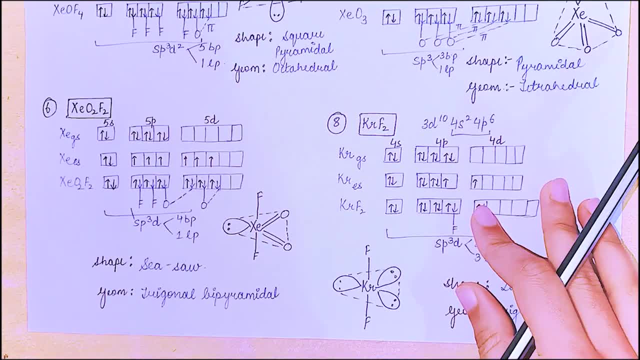 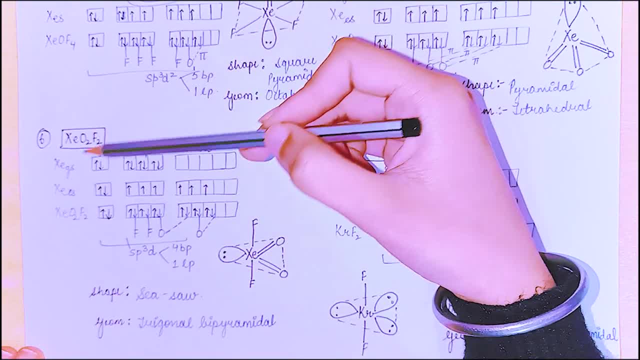 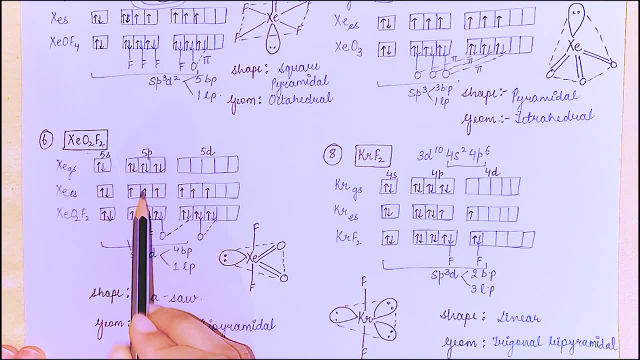 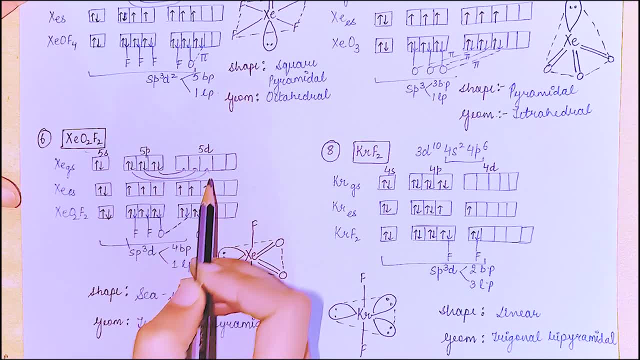 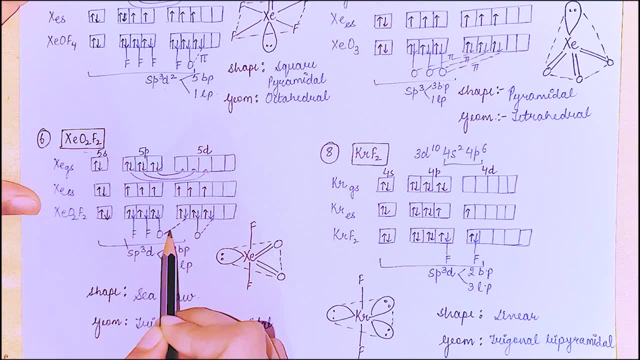 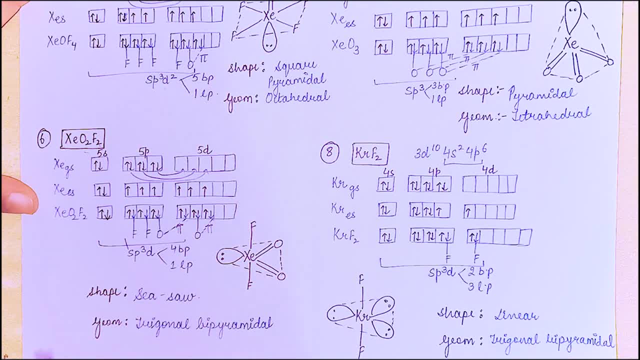 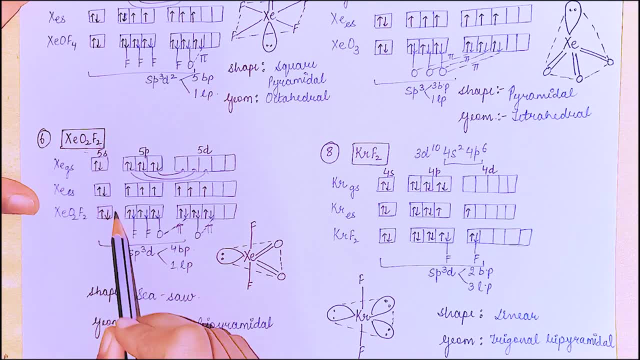 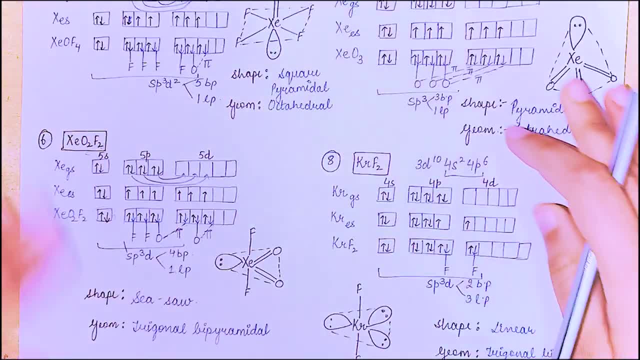 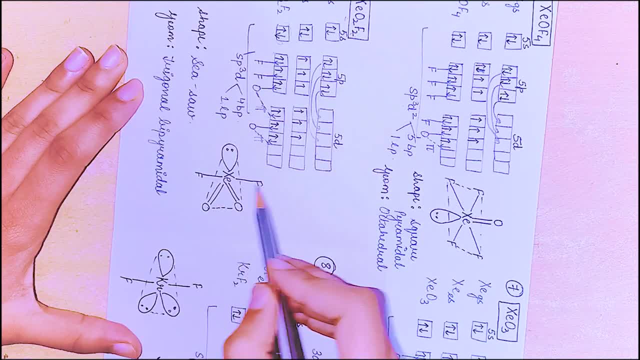 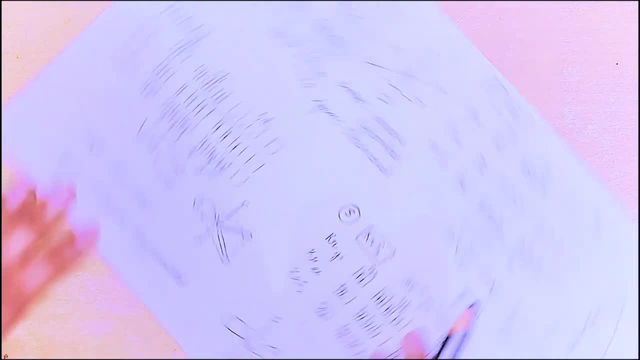 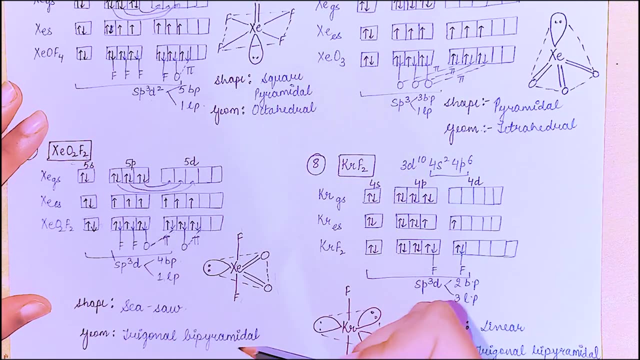 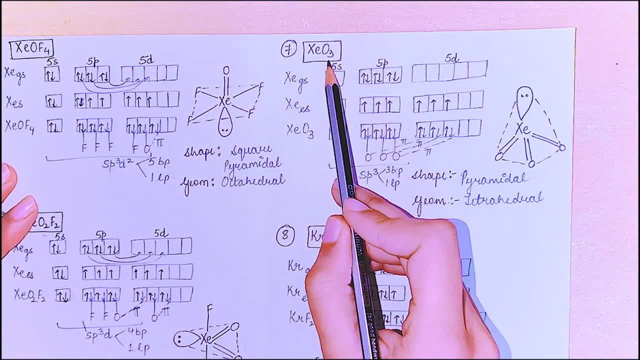 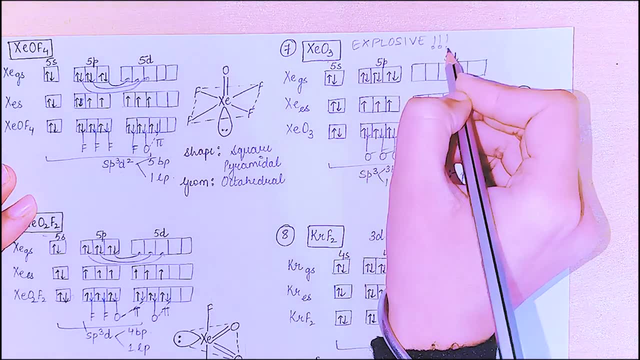 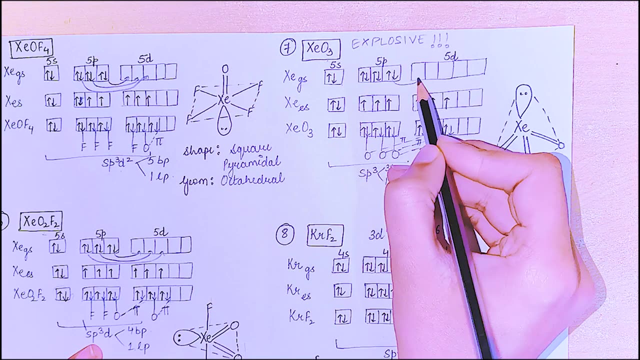 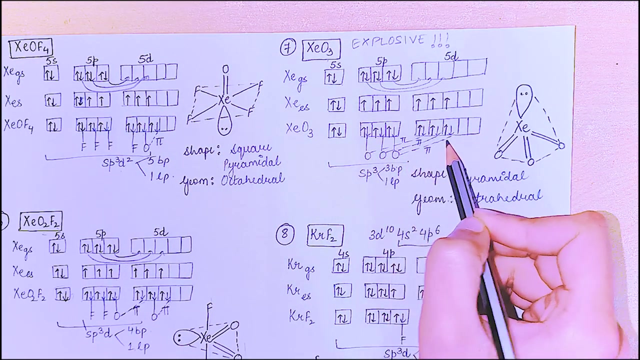 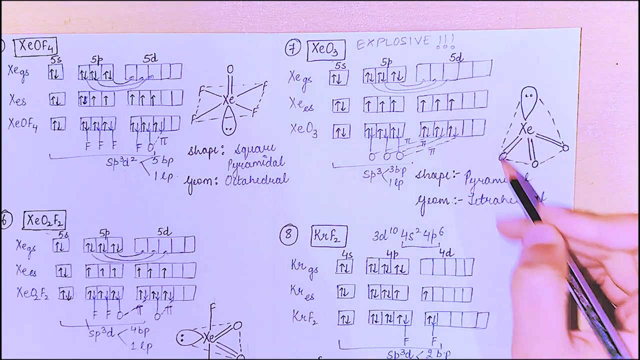 geometry. next compound is xco3, don't forget it is explosive. so xenon, we need to excite again three electrons to get six places empty. we put three oxygens and form three more pi bonds here. so the shape is pyramidal, it forms like a pyramid, so it is called a pyramidal shape and geometry is tetrahedral, as you can see next. 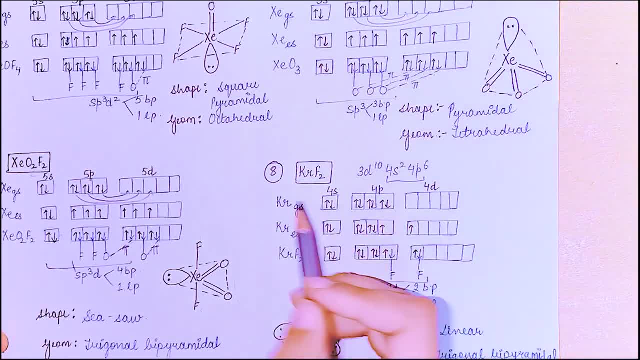 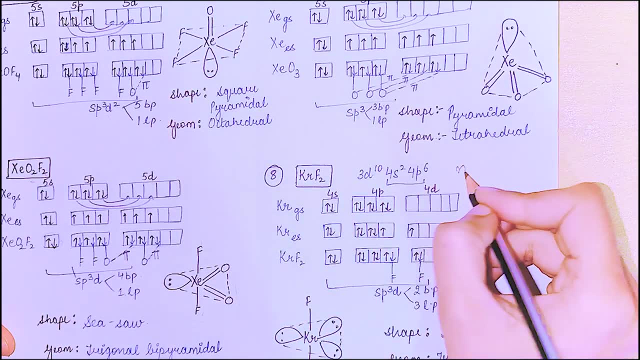 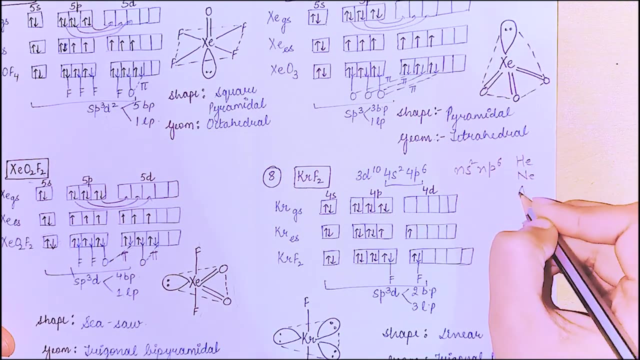 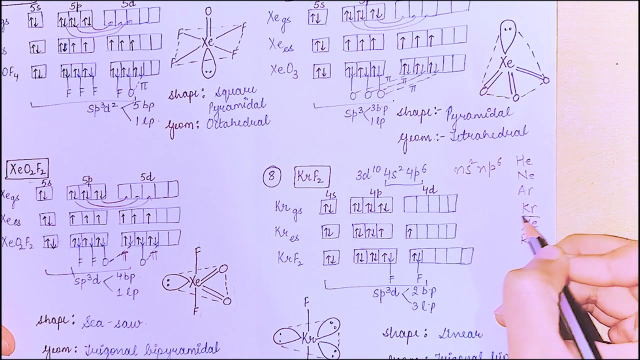 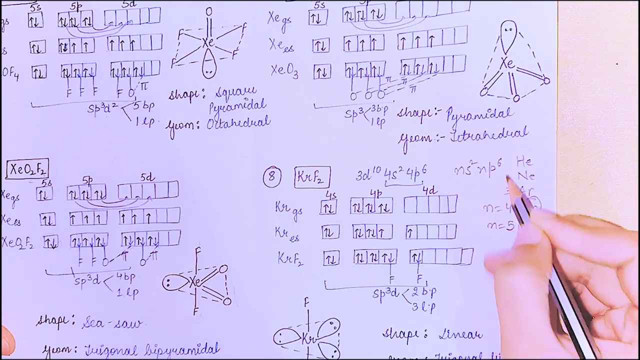 compound is of krypton. it is krf2, krypton difluoride. the configuration is again ns2, np6. in this way you can say: this is xenon. we have written n is equal to five. so for krypton, n will be equal to four, three, two, one. this is to remember the electronic configuration. n is equal to five. 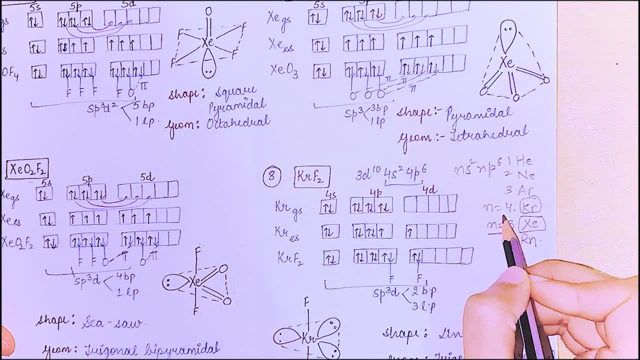 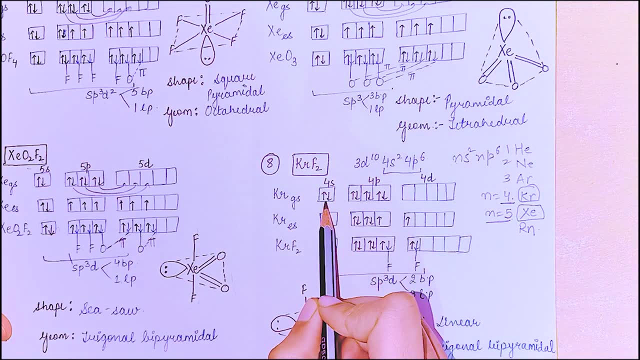 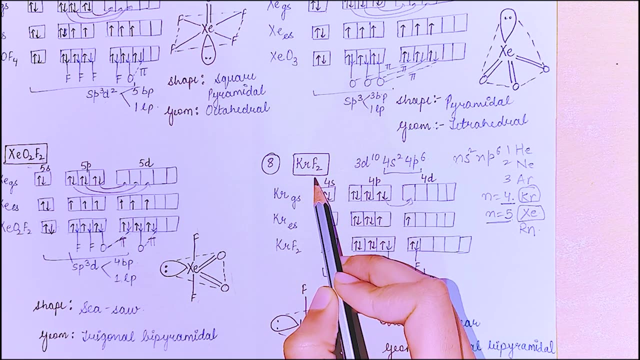 so five s2, five p, six for xenon and for four krypton. it will be four s2, four p6. so it is fully filled. now in the ground state, in the excited state, we have excited one electron because we just have to fill two fluorines. two places are empty. we can write. 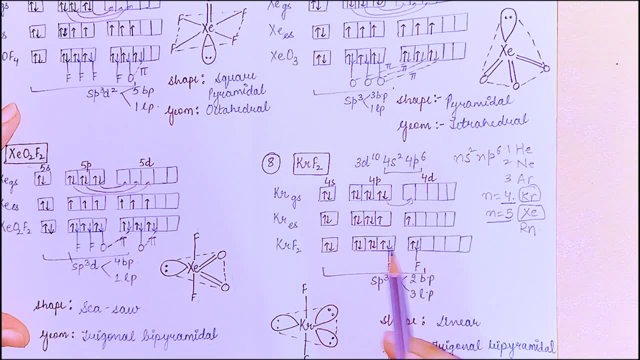 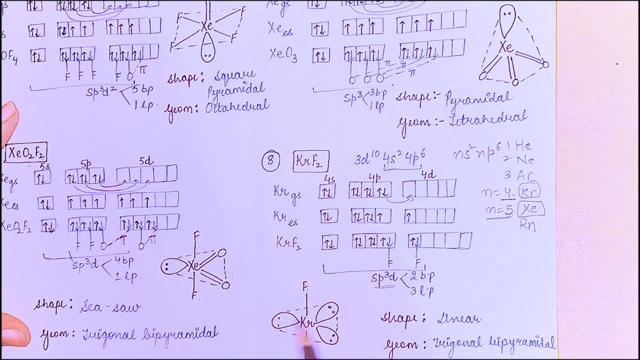 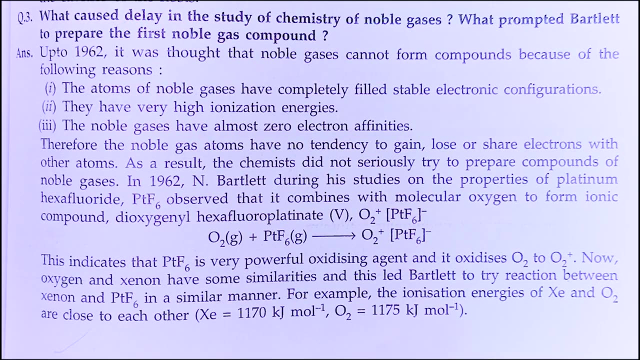 the fluorines. the hybridization is sp3d- two bond pair, three lone pair, two bond pair. so we form a linear shape and the geometry is trigonal bipyramidal, as you can see here. so we have already filled the neutral edge part, so it will go on the positive sphere. 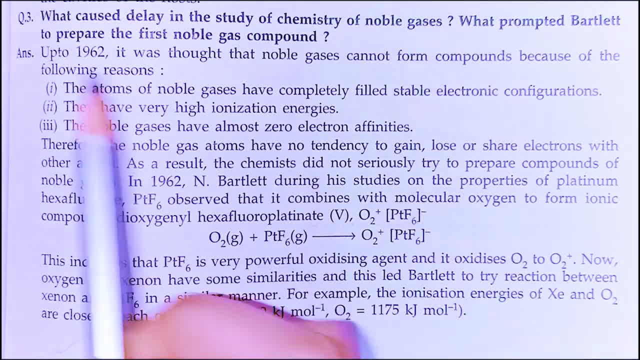 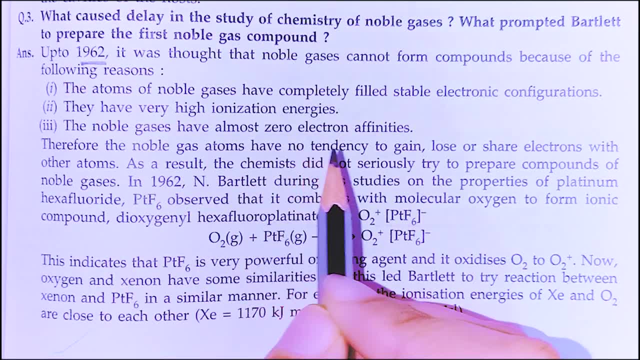 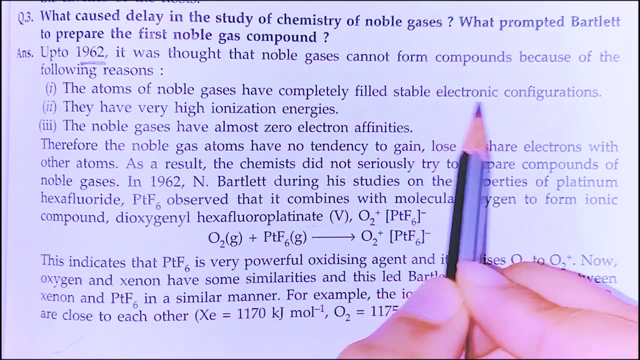 it is till shape: three a by относ plus one. we cannot ہے. star is equal to zero, so, and the value of alpha is zero, so this paste is ns2. come and let us deviate here. this is negative, so, and this is negative, so in this sense, we just have to limit this. Prince, think about it like it. they have very high ionization energies and the noble gases have almost zero electron affinities. therefore, the noble gases and noble gas atoms have no tendency to gain, lose or share electrons with other atoms. as a result, the chemist 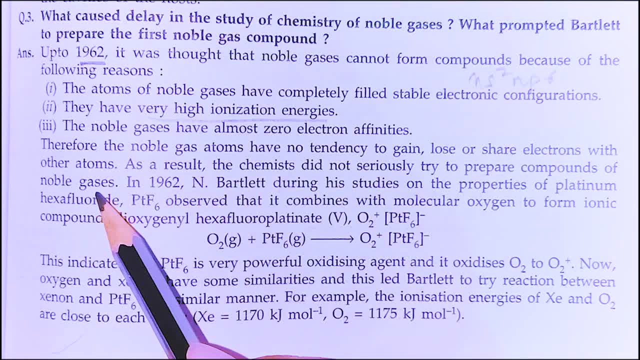 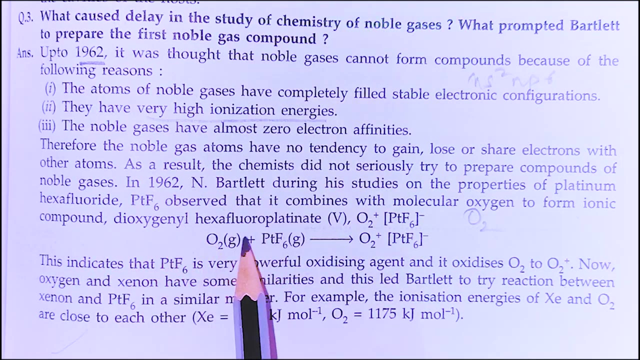 did not seriously try to prepare compounds of noble gases. in 1962 Neil Barlett, during his study on the properties of platinum hexafluoride, that is, ptf6, observed that it combines. it combines with molecular oxygen, that is O2, to form ionic compound, that is dioxygenyl hexafluoroplatinate. 5 in plus. 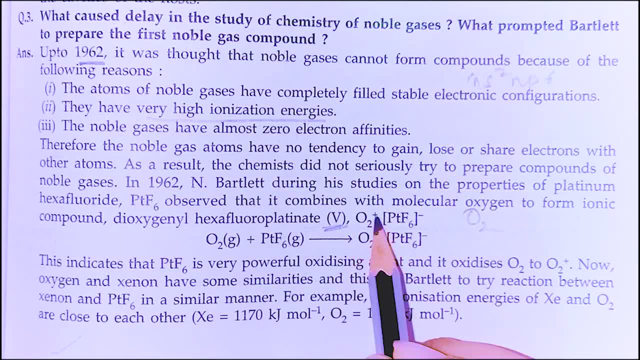 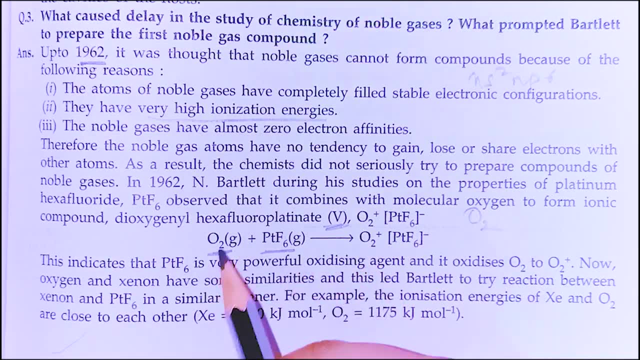 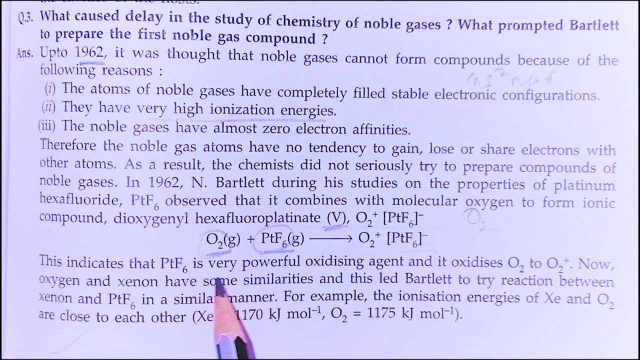 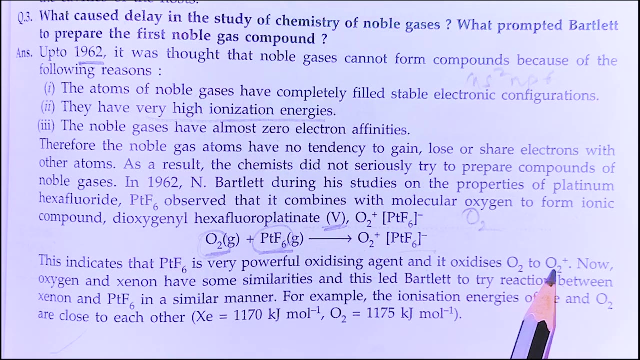 5 oxidation state that is, O2 positive- ptf6 negative oxygen oxygen. oxygen oxygen on reaction with ptf6 forms O2 positive- ptf6 negative right. this indicates that ptf6 is very powerful oxidizing agent and it oxidizes oxygen to O2 positive. 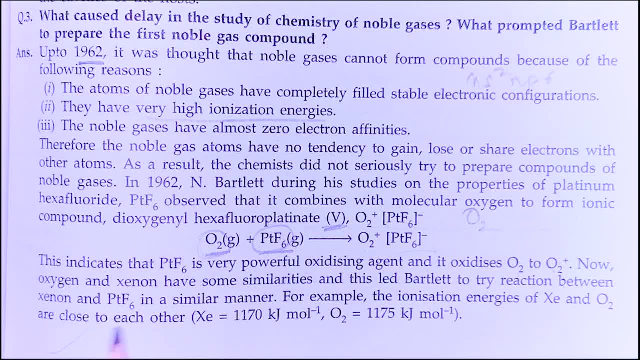 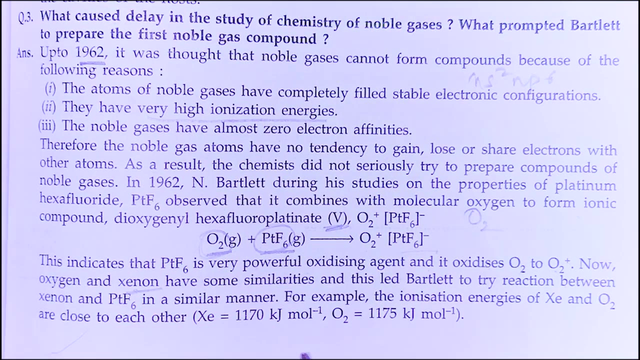 now, oxygen and xenon have some similarities, and this led Barlett to try reaction between xenon and ptf6 in a similar manner. so what is the relation between these, this reaction and the noble gases? they say that the oxygen, O2, is similar to xenon, so we can try xenon in place of 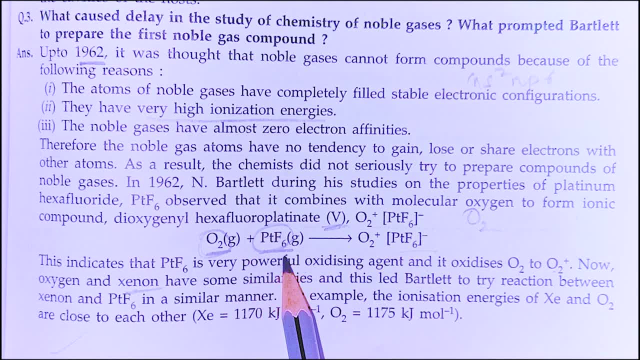 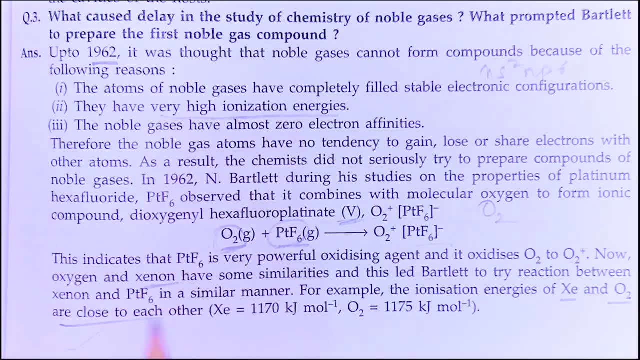 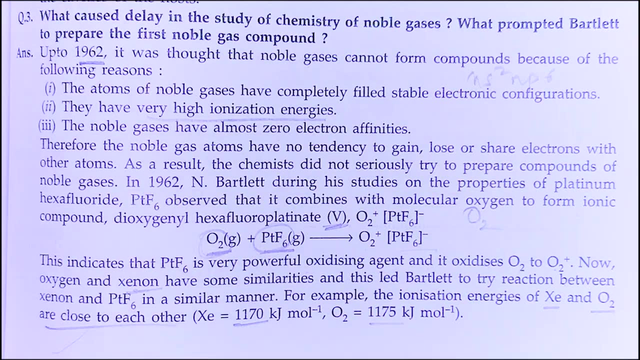 oxygen and reacted with ptf6, for example. the ionization energies of xenon and oxygen are close to each other. that is 117 zero for a xenon and for O2 it is 117: 5, so the properties might also be have be same. on this basis, ballet reacted xenon and platinum. 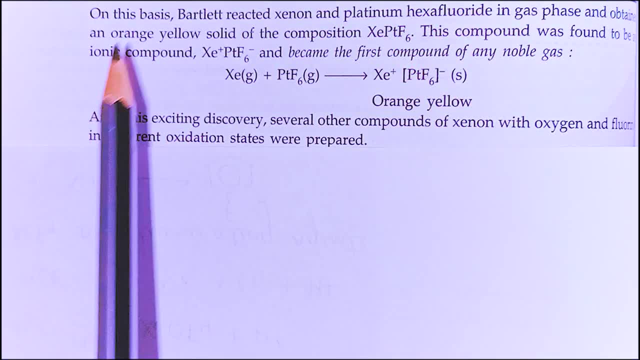 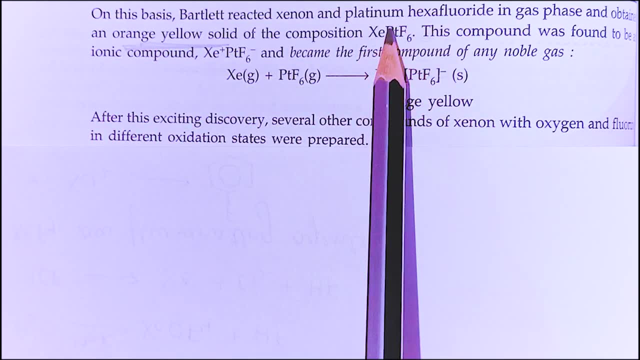 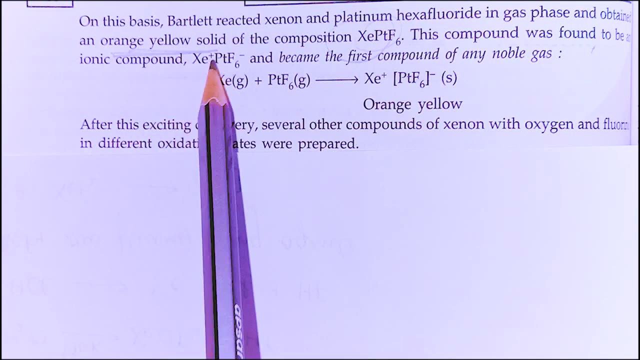 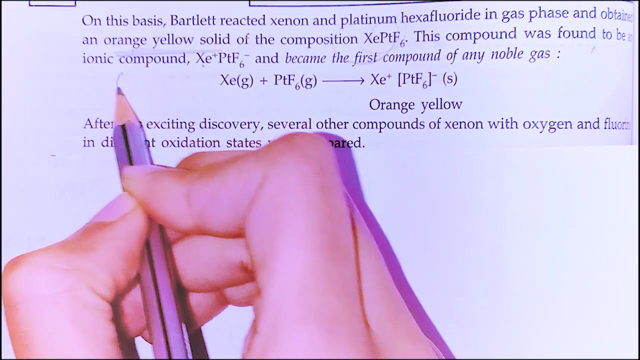 hexafluoride in gas phase and obtained an orange yellow solid. this orange yellow solid of composition xc, ptf6- this compound. this compound was found to be an ionic compound in the form xc positive, ptf6 negative, in the same way we got earlier. we got o2 positive, ptf6 negative. here we 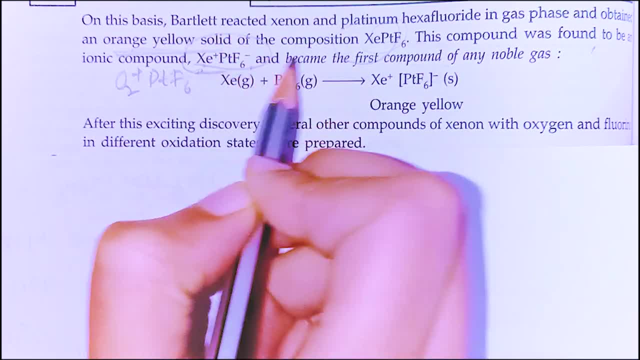 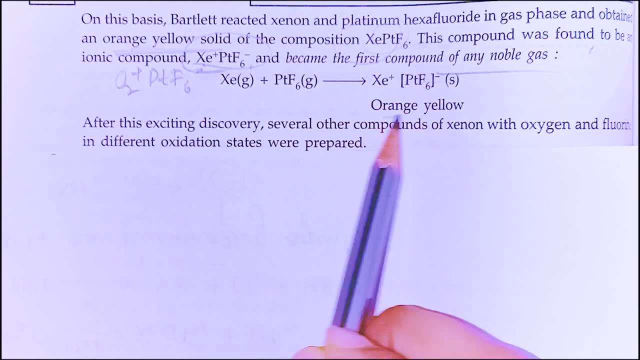 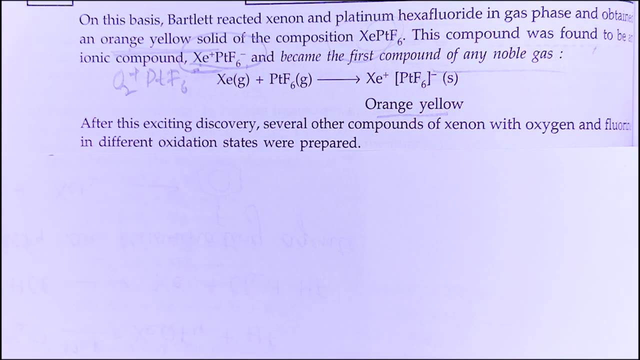 got xc positive, ptf6 negative and became the first compound of any noble gas. xenon plus ptf6 give this orange yellow compound. after this exciting discovery, several other compounds of noble of xenon with oxygen and fluorine in different oxidation states were prepared. so this was the beginning of reactions of noble gases. 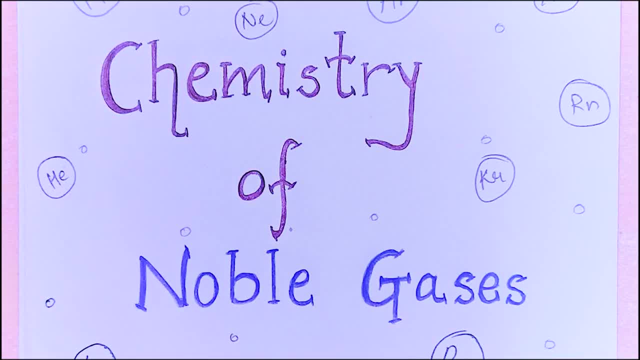 so this was about the chapter chemistry of noble gases. this video is getting longer, so i think i should make the questions in the next video, so stay tuned. don't forget to subscribe the channel, like the video and share it with your friends so that everybody can be helped from this video. okay, then, thanks for watching, bye.